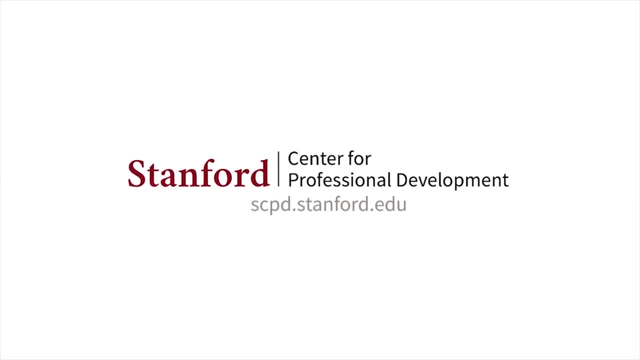 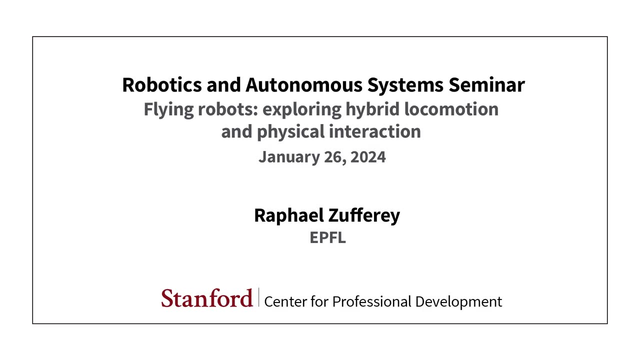 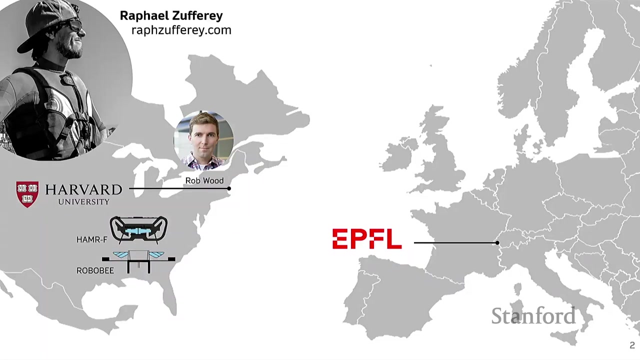 All right, awesome, Fantastic. So yeah, I worked with Rob Wood on two different robots, So here you have the Hammer F, a small legged robot, really exciting work- at about like one gram scale- and the RoboBee project, which, in this context here we're trying to have come out of the water. 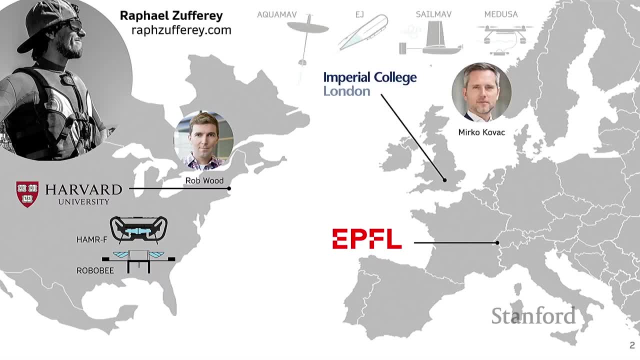 So that was one of the projects. I then continued with a PhD with Merkle at Imperial College, And so there that led me to work on several different platforms, which I'll be presenting a bit more in detail today. You have them up there in the slides, And I then did a short 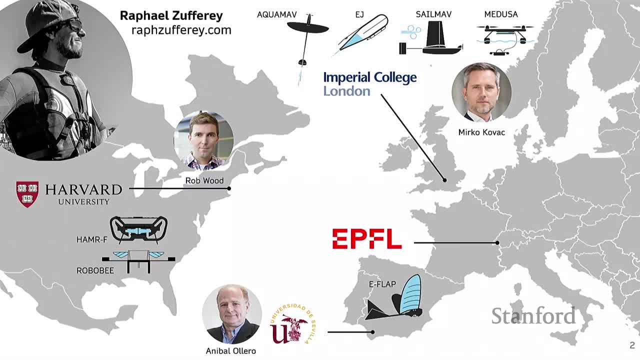 postdoc in the south of Spain with Anibal, And Anibal worked on very exciting large scale flapping robots, And so this will cover a bit today as well. And now I'm back at EPFL. I've got my own research grant to work on hybrid aerial aquatic flapping robots, And so we'll finish. 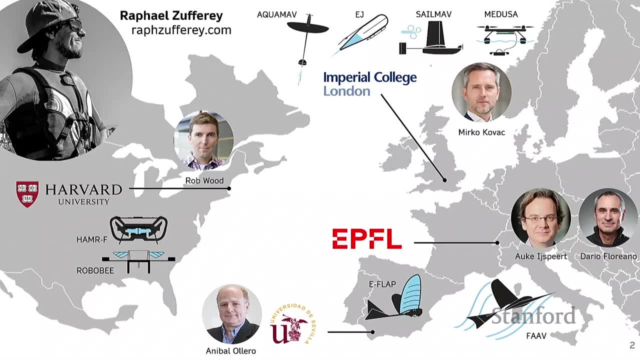 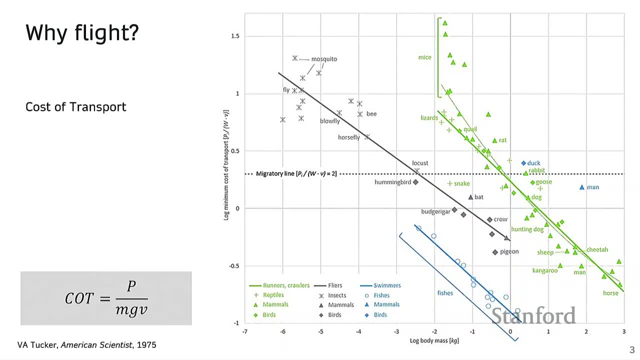 on that. So all of this, essentially all of these- were flying robots. And the first question is a bit like: OK, why flight? Why are we so interested about this? And one of the main reasons is cost of transport. So cost of transport can be defined as power over the mass of your vehicle, your 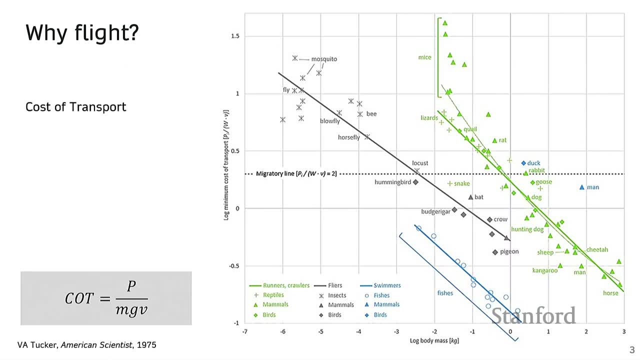 animal multiplied by its velocity, You can also define in terms of energy over distance. And essentially here in this plot you see three different categories of animals. You have walking animals- Those are the green lines- Flying animals, the gray and the fishes. 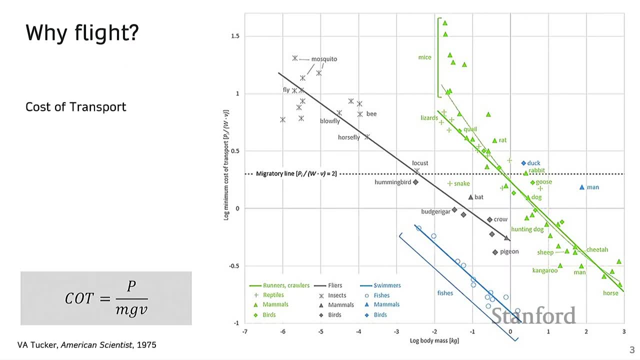 and swimming animals are in blue, And so what you can see here is, regardless of the scale, flying is more efficient in terms of cost of transport as a walking robot, So this is one of the reasons that I think flight carries a lot of potential. of course, You also have 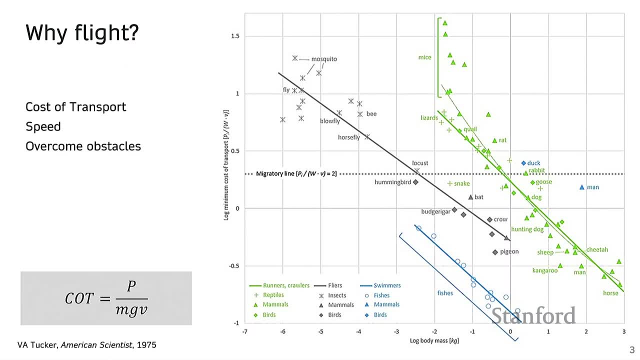 higher speeds that you can achieve in terms of flight, And you can also, over the course of time, overcome obstacles. So these are kind of the reasons why I think working with flying robots is particularly exciting. Now, when we look at our planet, it actually looks like this: 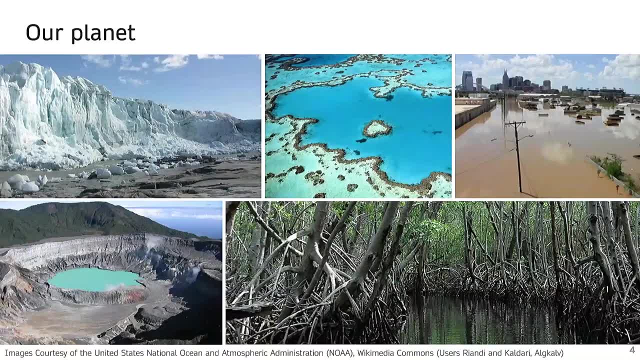 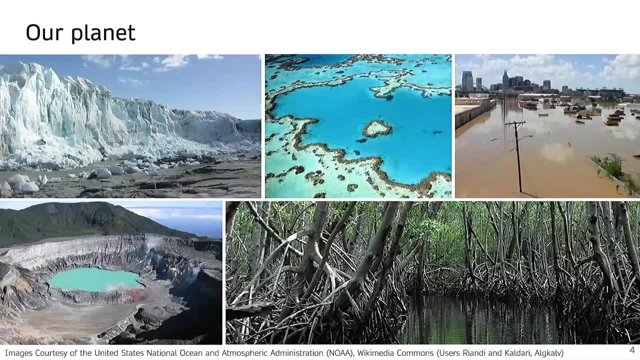 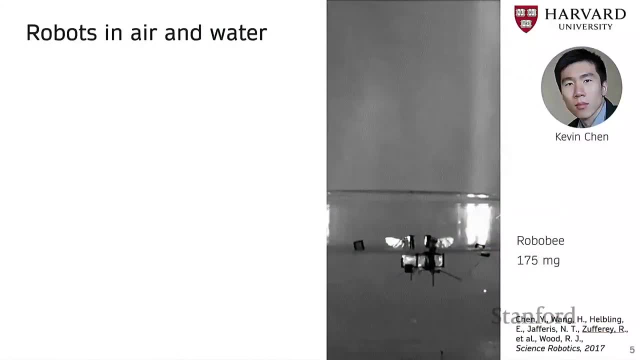 work in these types of scenarios, So that's a bit what motivates me to work on this hybrid locomotion. So let's start with an example: the Robobee. So this was developed with Kevin Chen, who's now a faculty at MIT. 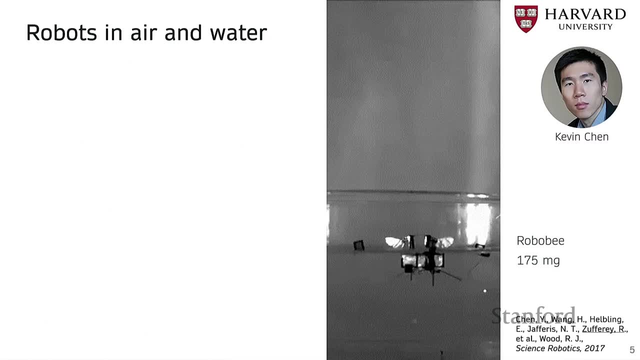 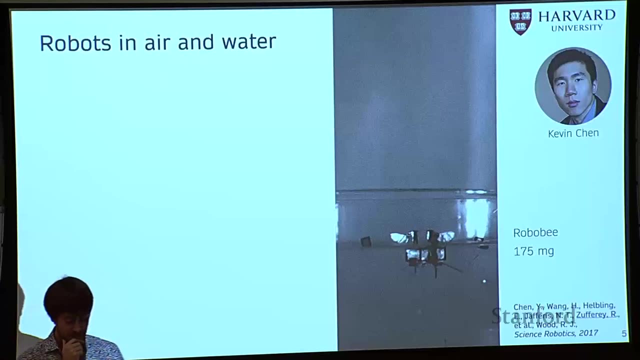 And the Robobee is 175 milligrams. Here you see it resting on the water surface inside of a beaker, So it's a tiny robot right a few centimeters across, And so the part that's underwater here is actually a tiny combustion chamber, and you have the wings that are outside of the water. 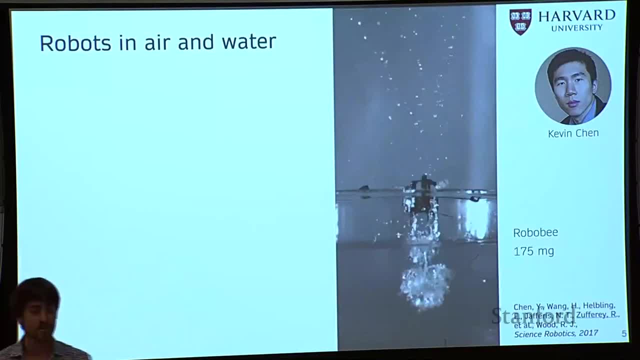 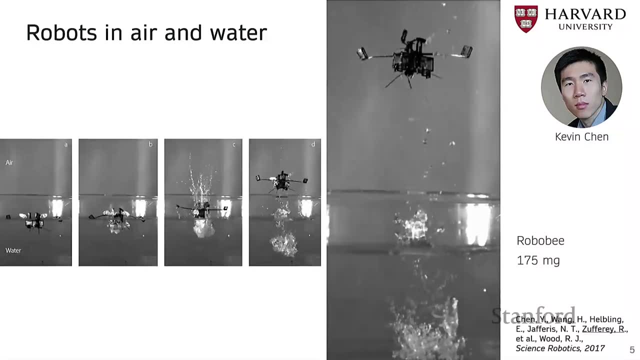 surface. And so here, slowed down 200 times, you can see how the robot is able to come out of the water and get into a flight phase. Let's break it down a little bit together. So the first step that the robot does is electrolysis. So here we have essentially two plates that are sticking inside. 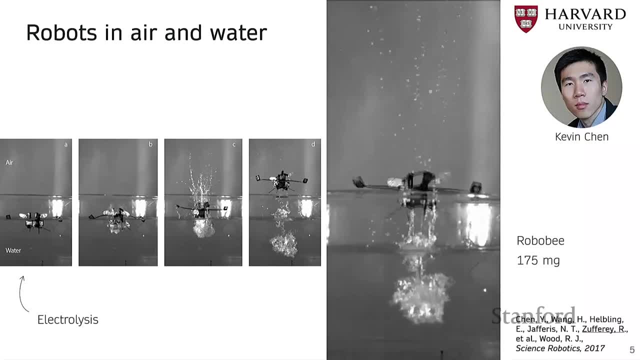 of the water inside of this chamber at the bottom, And we apply a current between these plates and so you separate the water into hydrogen and oxygen, And so what's nice about that is it starts to fill this tiny combustion chamber a few millimeters across. It starts to fill this chamber and the robot just naturally gets to the. 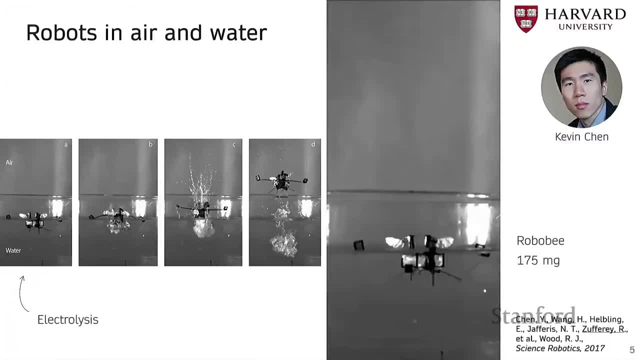 water surface. So that's one of the nice things about this- And you have this combustible gas that you have at the water surface that you can then ignite. And one of the benefits of these types of robots is they work with piezoelectrics. 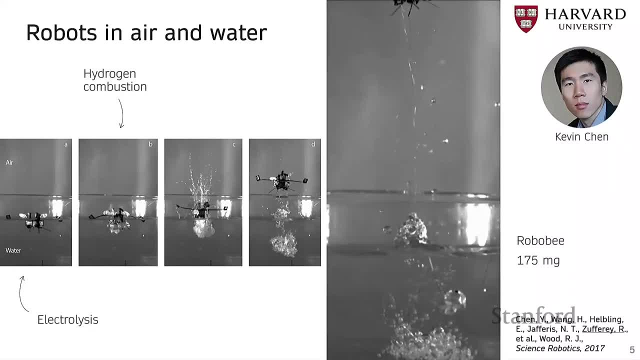 And piezoelectric motors run at high voltage, So around 200, 300 volts, And that's actually sufficient to generate a spark between two very closely located contacts. So actually, without adding much in terms of spark electronics, you can get to ignite this gas mix. 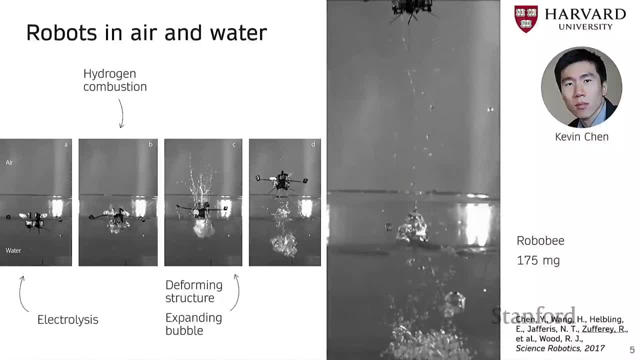 We then have the combustion progress within this chamber, and yet there are several things that are happening here. We have a bubble that gets created on the water. A lot of energy gets dissipated in that, And we have a highly deforming structure. 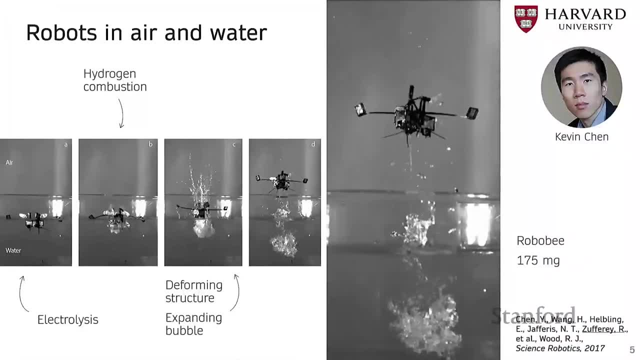 So suddenly this robot that essentially was rather hard becomes very deforming from the forces that we have, And then we get into free flight, And so this was published in 2017.. Very exciting project, And it was a bit the start of aerial aquatic locomotion for me. 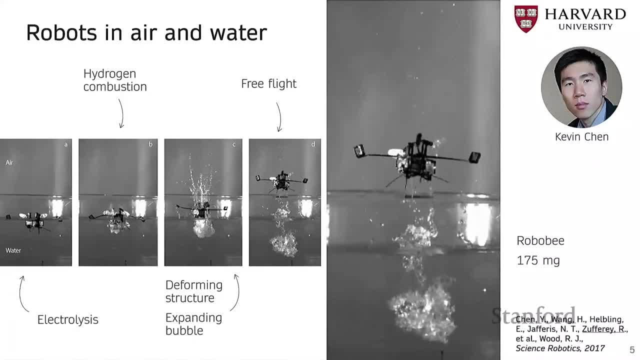 And we see here that, even though this is very promising, there's still a lot of limitations. Of course, it's a microscale robot. It's tethered, The water surface has been changed in terms of surface tension, So several things have been done. 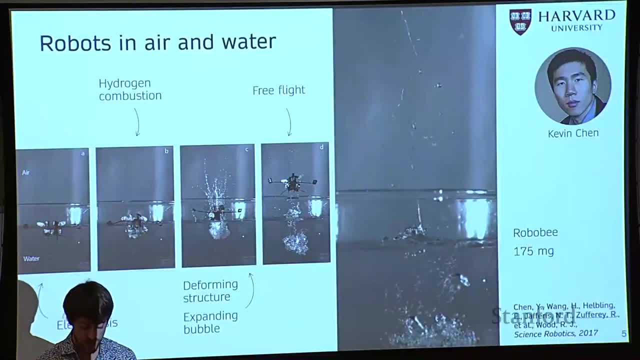 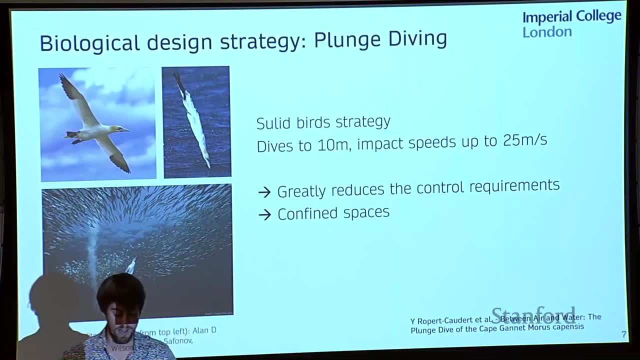 To be able to enable this, And then, when I started my PhD, we're looking at different strategies for bigger robots. So you will change scale. Now we'll go to like kind of the half meter scale type robots, And one of the strategies that birds employ to dive into, to go into the water is they dive head first. 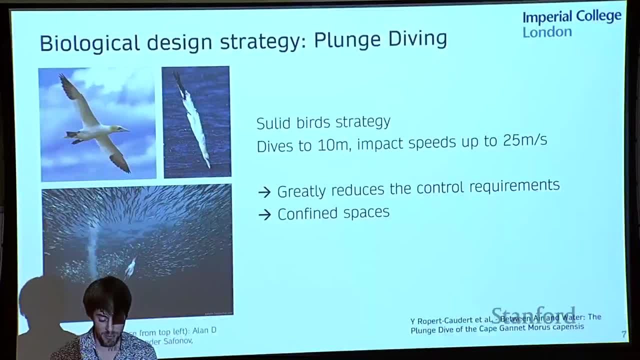 And so this is pretty cool. I should actually put a video of this rather than the photos, But you see how the birds are able to fold the wings and dive underwater, And this type of approach is nice because it reduces control requirements. You just really need to fold the wings and you dive in. 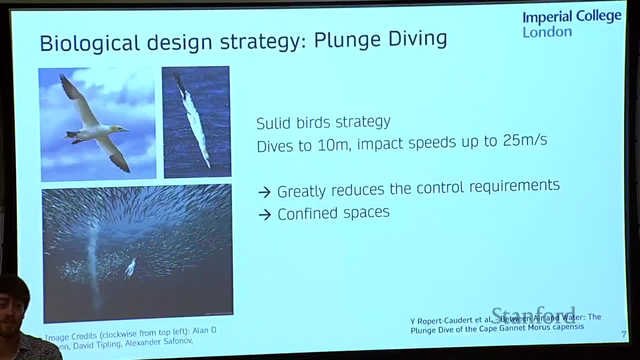 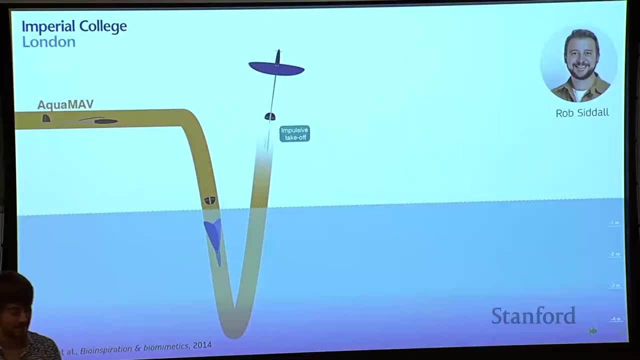 And you can do water entry in confined spaces, So you don't need a landing area to work with these robots. This was turned by Rob Siddall into a robot called the AquaMav 2014.. So this robot is able to fly with extended fixed wings. a propeller in the front folds the wings backwards and dives into the water. 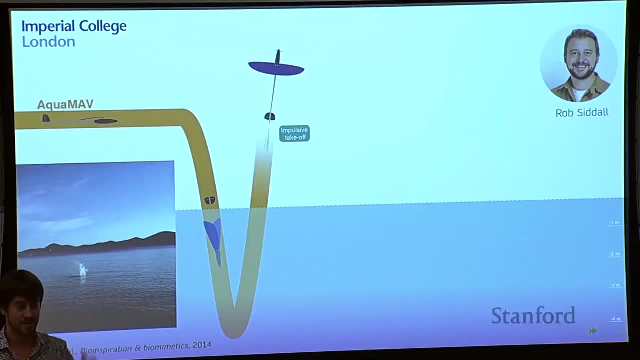 So this is a field test we're doing in Croatia. here You see, the robot kind of Loses control a bit as it as it dives, But that doesn't really matter. It still goes head first into the water. And then this robot has a tail and the tail is full of water. 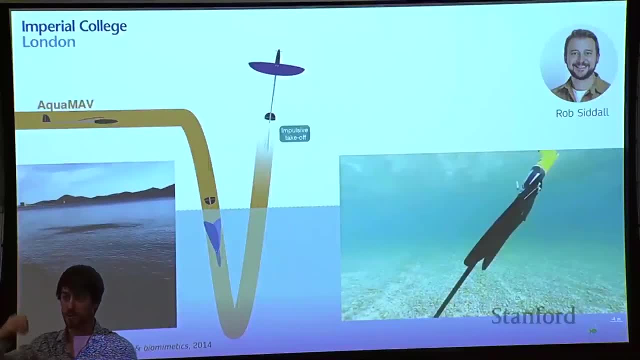 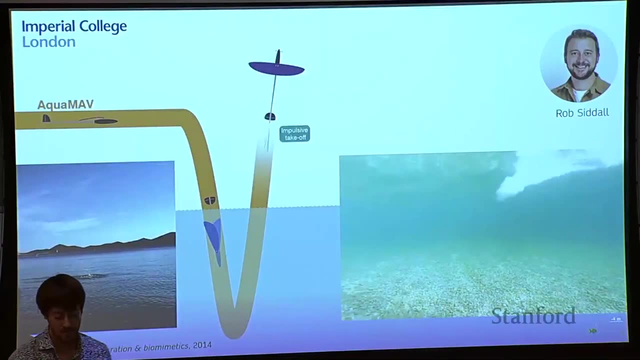 And when we open a gas cartridge that's inside of the head of the robot, we actually expel all this, all this water, out, And that creates a jet that launches the robot back into the air, And so this is really nice strategy. It's quite robust. 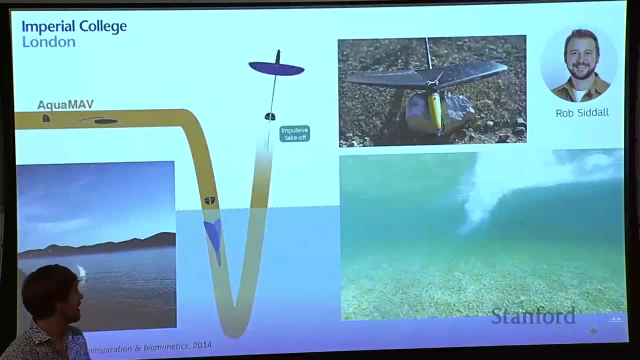 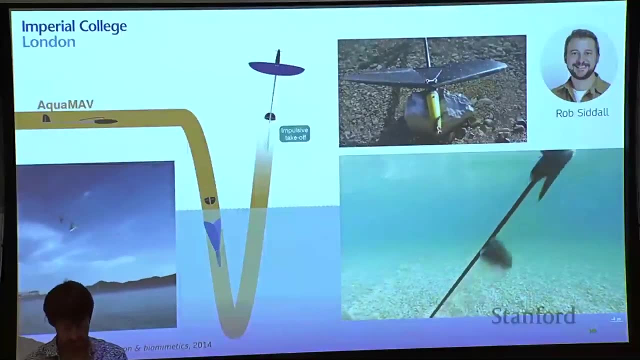 And we're able to essentially get speed. the flight speeds again. The wings are able to morph backwards, So they're servo actuated and the propeller is in the front, And this is a really cool project. A lot of successful success stories from this. 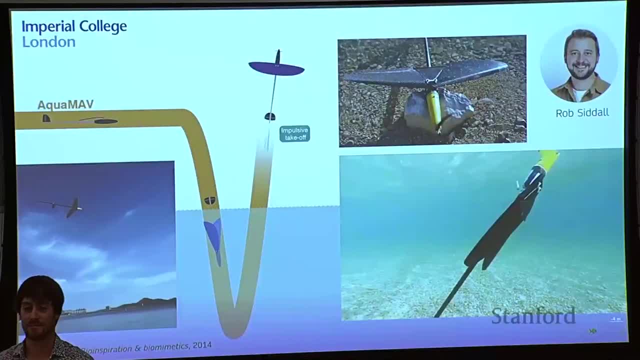 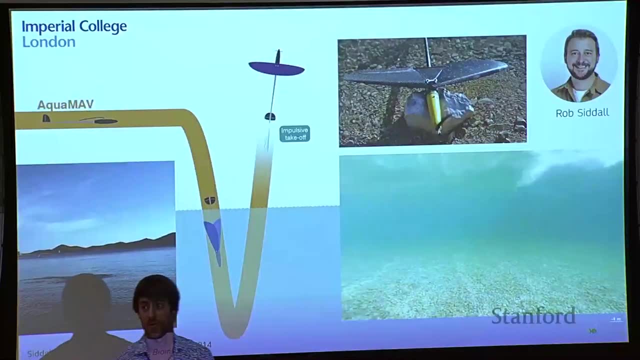 But it has. one issue is, once you open this gas cartridge, that's it. You've you've released the pressure, You've done your one jump and you cannot do anything else anymore, And sometimes the launch fails. So you'd be like stuck in the water. 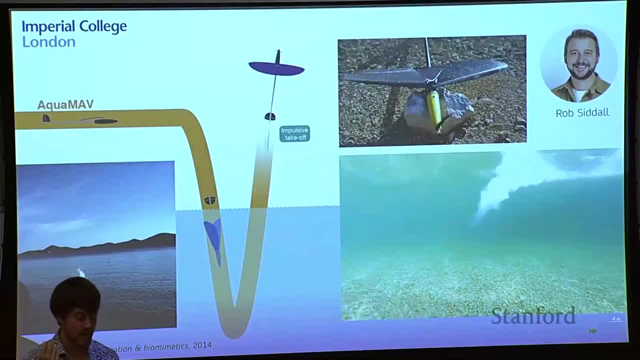 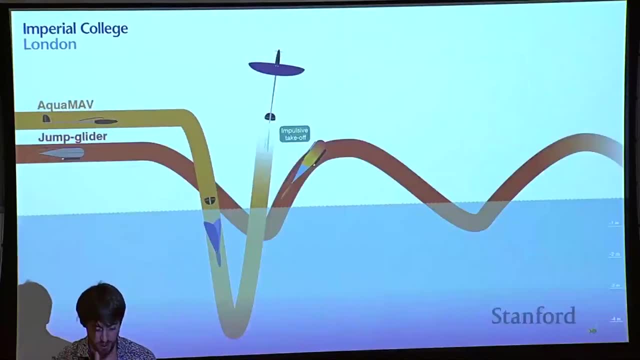 So one of the things we tried to solve was: OK, how can we do this? How can generate this high pressure on board Without actually having being able to do it multiple times? And so there we worked on the jump glider. So here it's a bit of a different approach, rather closer to flying fish and other animals. 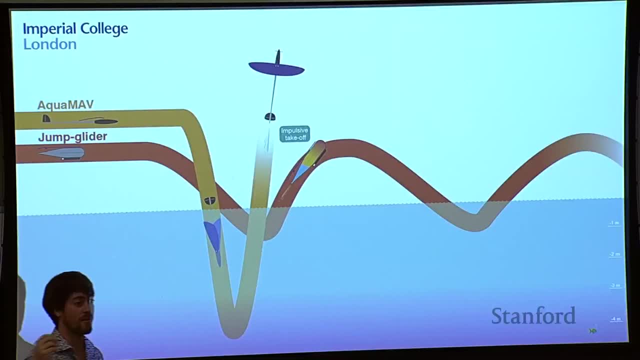 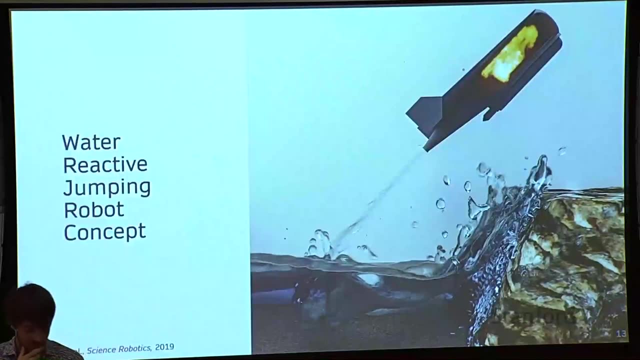 And the idea is that we can jump and jump multiple times out of the water and then glide to extend our distances, And so this led to the water reactive jumping robot concept that was published in 2019.. And and it was able- it was able- to leverage the energy in the environment to actually do this jump. 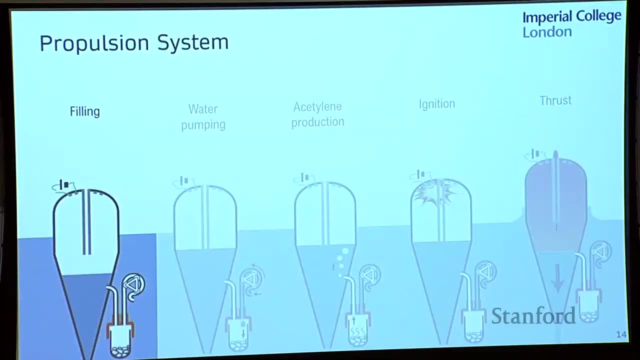 So stay with me on this one. This is a cross section of the robot, So we have a combustion chamber with a tiny amount, a tiny fuel amount that we have down here, And so what happens is we have calcium carbide at the bottom that we fill into this tiny chamber. 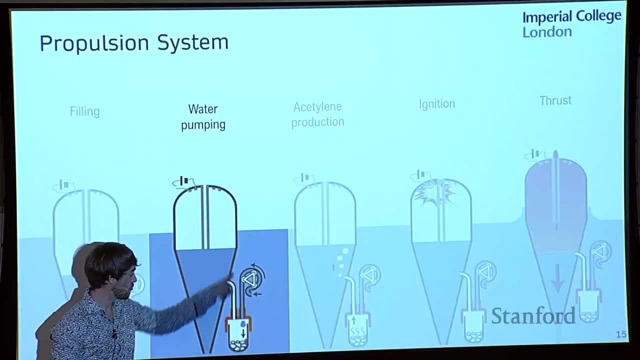 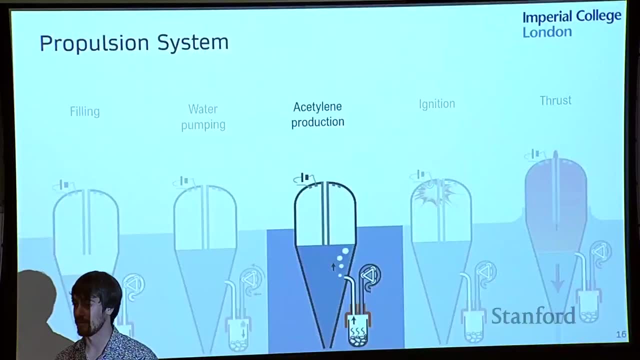 So we're talking about like a centimeter And we pump a drop of water onto this. calcium carbide, Calcium carbide, CAC2 reacts very strongly with water and creates acetylene. The acetylene then gets released into the main chamber and it mixes with the air that we had in the upper part of the robot. 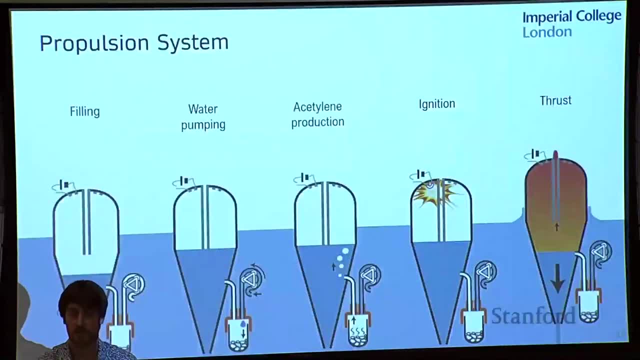 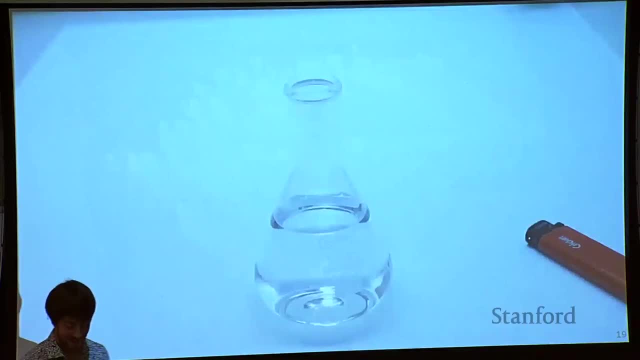 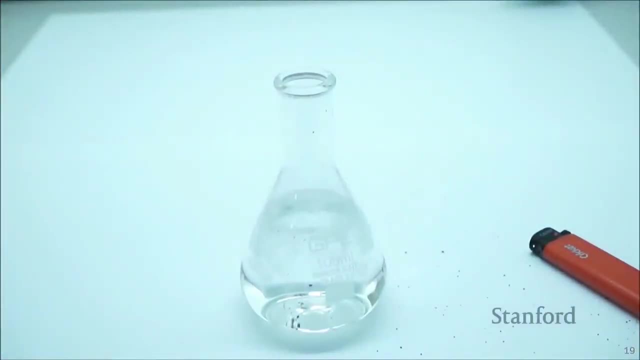 We then ignite this gas mix and that creates pressure and pushes the water out of the tank. So this is what it looks like in lab conditions. You take the water in your beaker, You add calcium carbide. Notice that it's a very small amount that we're pouring in. 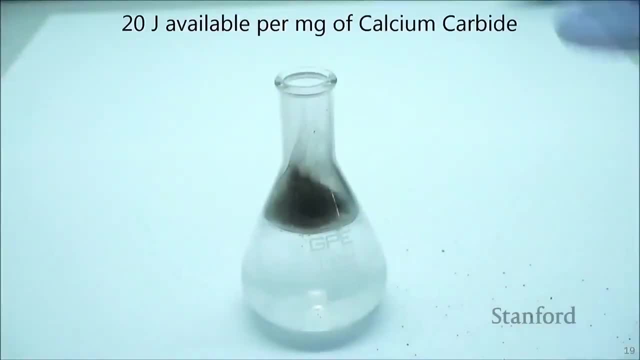 And then you can the acetylene, you can ignite it, And that happens really quickly, And so what's really nice is for a robot about this size- So we're talking about, like this, 200 grams- We need 50 milligrams of fuel to be able to jet back out of the water. 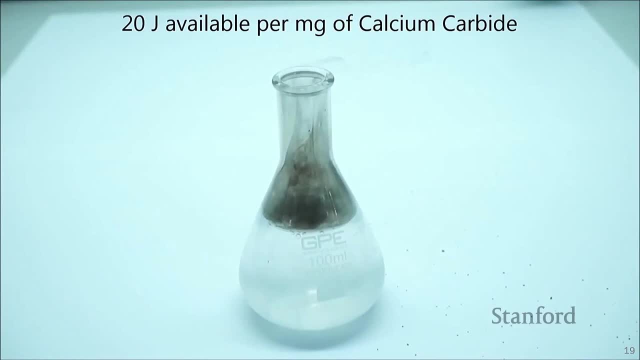 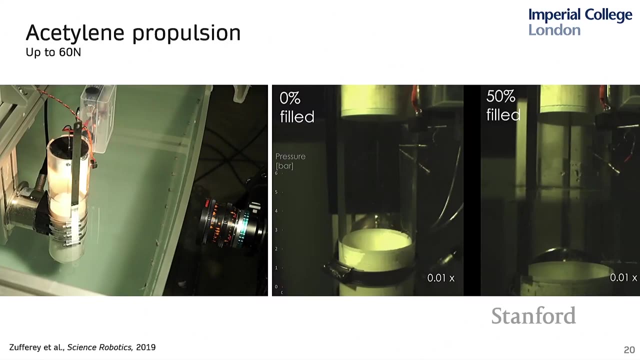 So the amount of fuel that's required is really small, And that means we can store quite a bit of it for several jumps. The first thing we did is actually try out this combustion chamber. This is a combustion concept into a transparent chamber. So this is a combustion chamber with 3D printed inserts that we're filming at high speed. 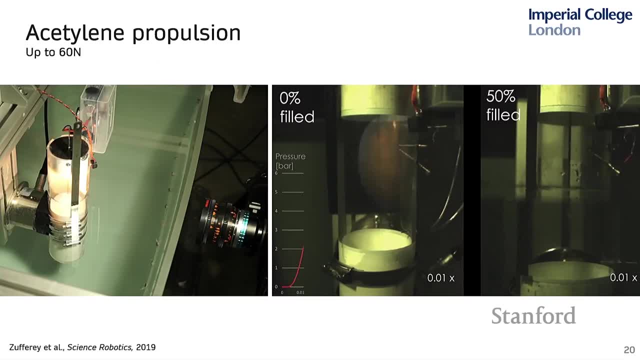 And here you see in the video the combustion progressing through the chamber And we're measuring the pressure in real time. So we have pressure sensors And the video on the other side is with water flooded already in the chamber, So you see the waterfront actually slowly getting pushed out. 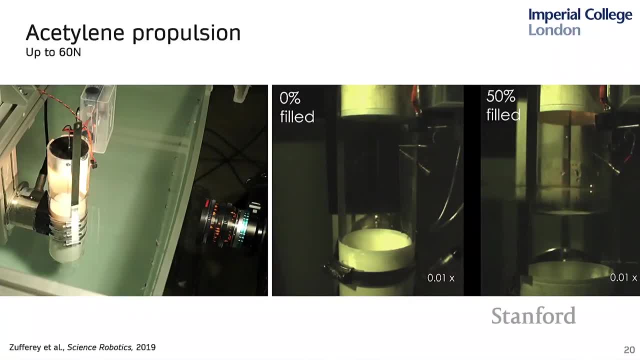 And so this was nice. We were able to test out some of the hypothesis that we had: verify that we can get a reliable combustion- Not so easy when you're in a water environment, But in the end we managed to figure out quite a lot of the details here. 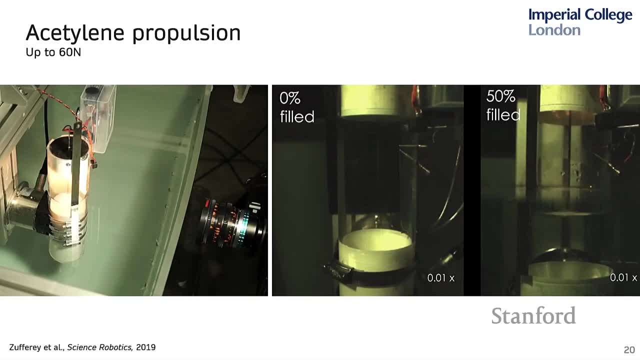 Now, there's still some things that we couldn't quite figure out just by looking at experiments like this Is how much water should we want in the robot in the first place, Or how big should the nozzle be, And so what we did is we actually developed a model, just an analytical model. 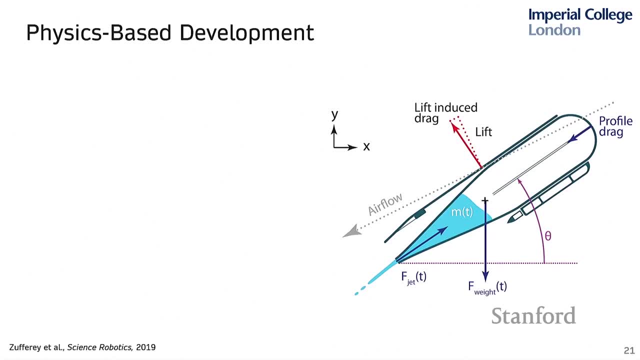 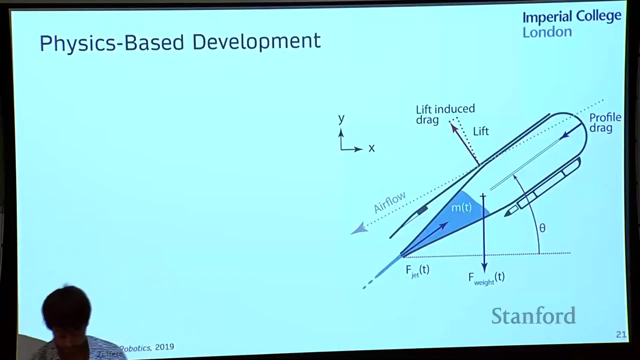 And when you try to approach this problem, there's two considerations. There's external aero considerations, where the forces on your wings, on your body, matter And the forces comes essentially from this jet. So you actually need to define this And it changes over time as your combustion process extends. 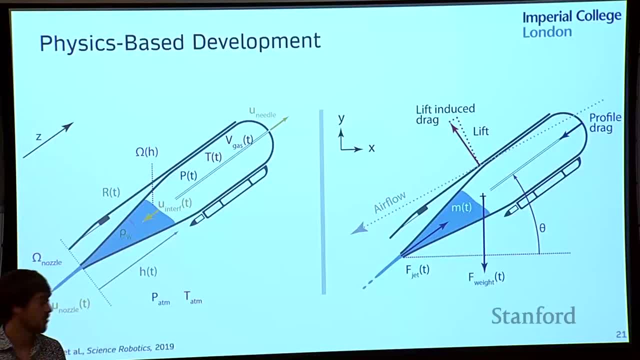 And so on the other side you need to consider the internal combustion processes, And here you have to solve the thermodynamics on the inside in the chamber And then your Euler's fluid equation for the escape. And if you solve that both together, 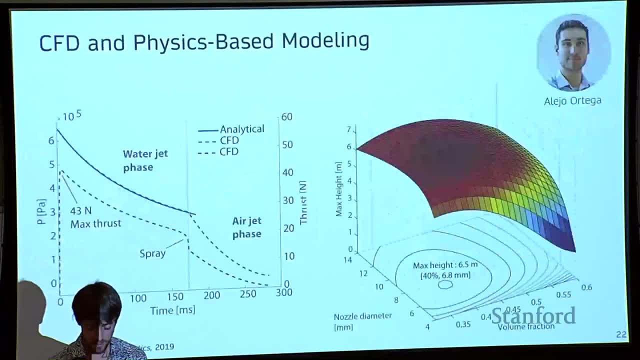 then you can get an approximation of your flight trajectory. We compare this against CFD- multi-phase flow, CFD inside of the chamber, And you can see here that the pressures align quite well with the CFD. We're modeling essentially the part. 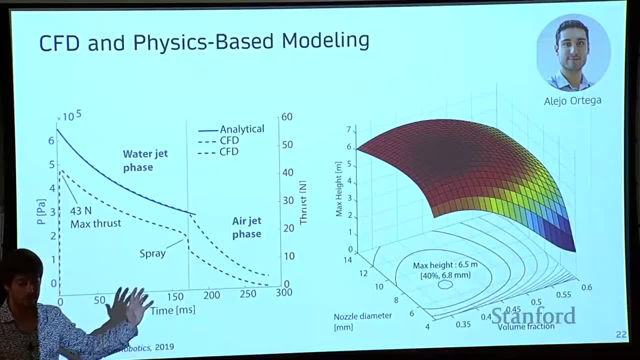 the first part of the process where there's still water in the chamber. After that it becomes sort of an air phase, where there's still pressure but the water is already gone, And with that we're able to optimize our robot to get the maximum height. 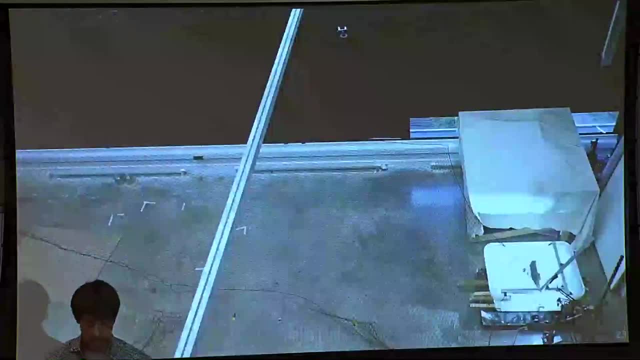 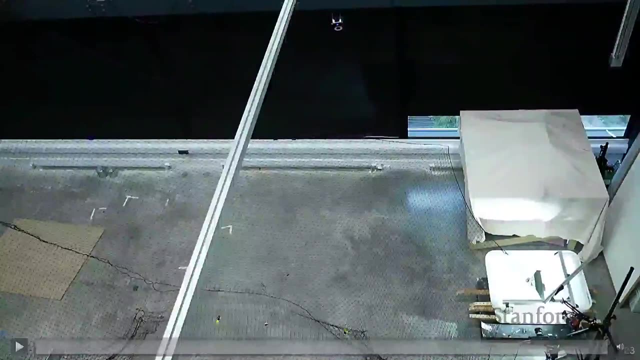 and therefore also the maximum distance. This is the flight zone that we had at Imperial College in London: Really nice space. The blinds are down, but you have the skyline of London in the back. It's beautiful, And the robot is sitting in its tank down here. 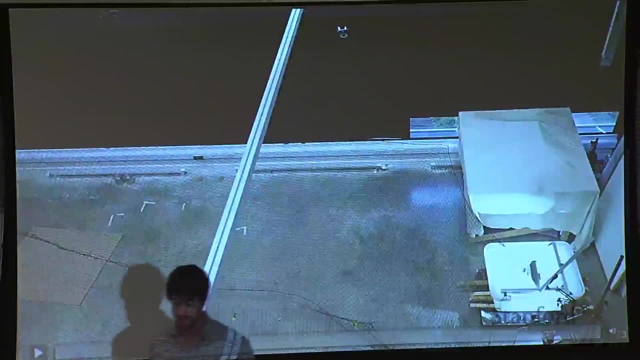 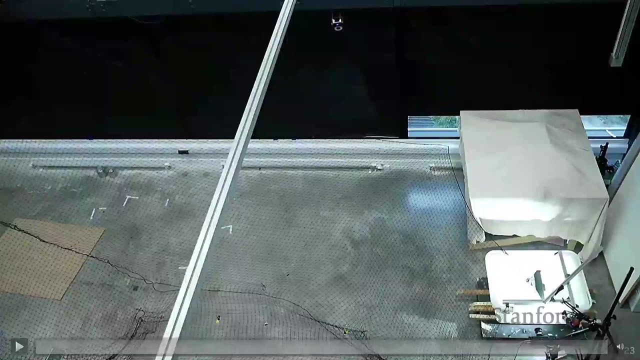 So we have it here: transparent window on the side so we can see in slow motion what it looks like, And we have about two-story high tracking zones so we can actually launch this thing quite high, And in this video you'll see how this works. 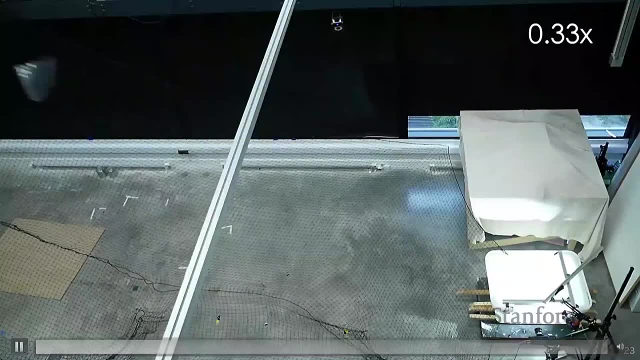 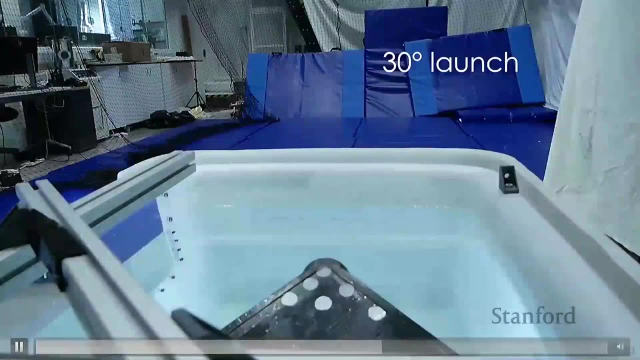 It happens really quickly, so we're trying to slow it down. There's more videos of the robot in close proximity. We're trying to also look at launch angles, because this is something that, when we design our electronics, we could shift around the center of mass and center of buoyancy. 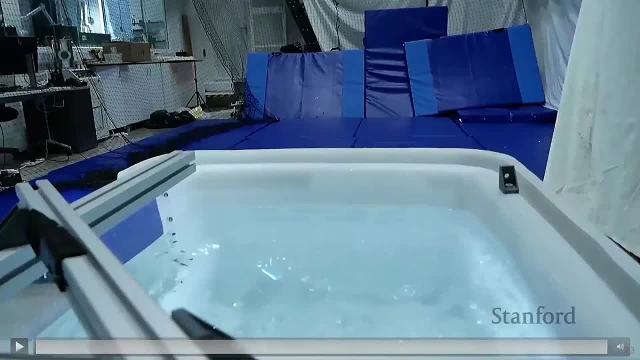 to change the floating angle and therefore the angle at which we launch. So this was exciting. We're able to essentially get these launches quite reliably And at the end, what you have in a robot like this in terms of electronics is not that many components. 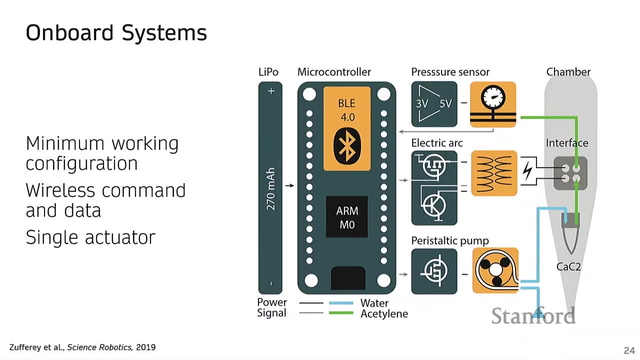 But they do undergo quite a lot of stresses and difficult things, including water, electric arcs. So, the way this was working, we have a small battery on board that was powering this microcontroller board with Bluetooth, So that was our way we were communicating with the robot. 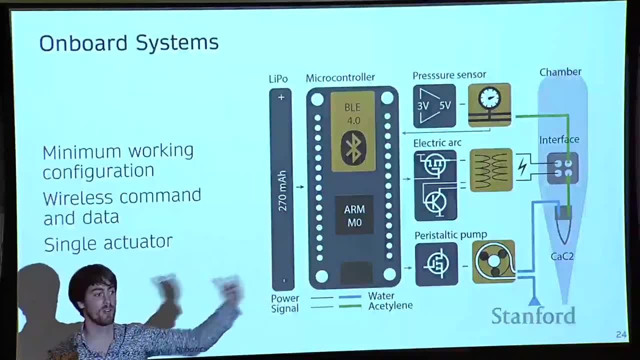 because at the end it's at the water surface and it goes into flight. So cables is not really an option here And this board is controlling a pressure sensor just recording data at kilohertz speed. because we did want to know, you know. 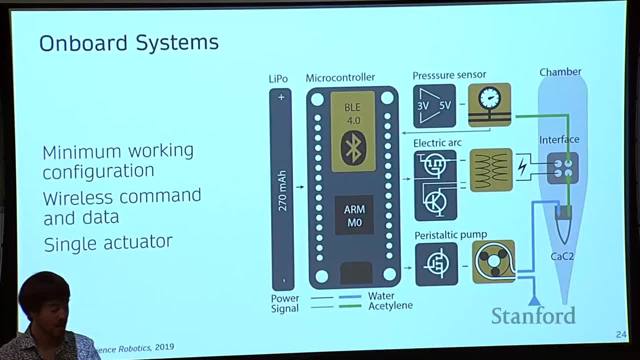 if we were actually getting the performance that we should be getting. We have an electric arc system that was generating, essentially, a spark within the chamber And, finally, a tiny peristaltic pump that was able to pump a droplet of water from the environment. 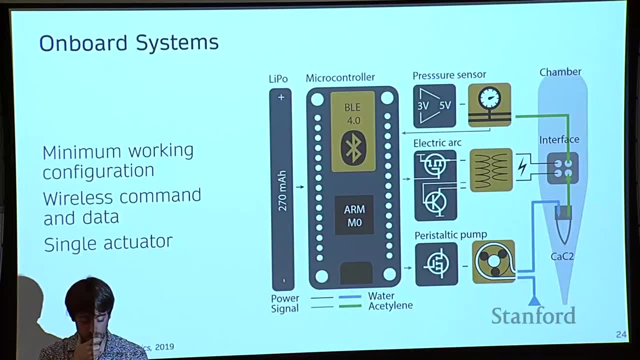 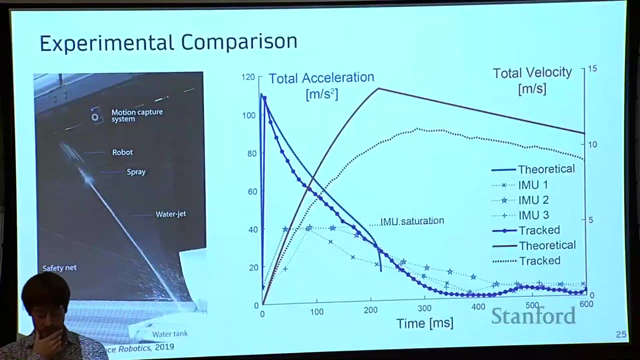 onto our calcium carbide fuel, And so all of this was designed out of carbon fiber: the interface, the main chamber, And so there's a lot of composite development there to make a system that could withstand the pressures that we have. We're looking also at accelerations and velocities of the robots. 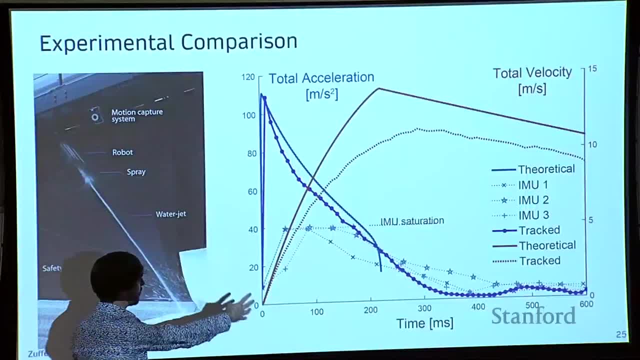 to see whether we actually get the performance that we predicted. And so here you see in blue, this was the theoretical performance of our robot, And we're able to get fairly close in terms of tracked motion. So that's the purple line- And also in terms of IMU data for the accelerations. 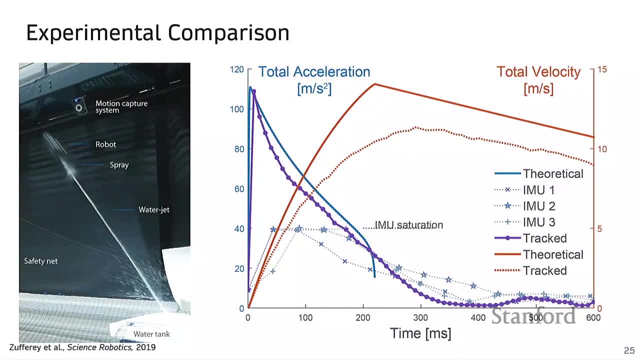 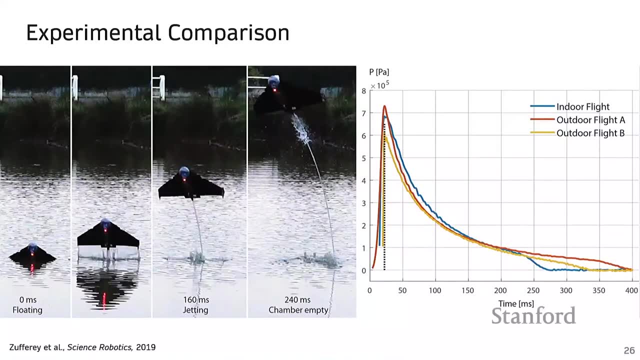 The velocity is a bit off, but in general we felt at that stage we had a good understanding of our system. This was then tried outside in an undisclosed location outside of London, where we're flying this robot outside of a pond. 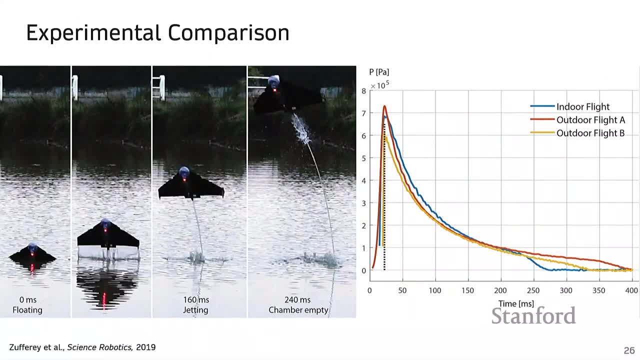 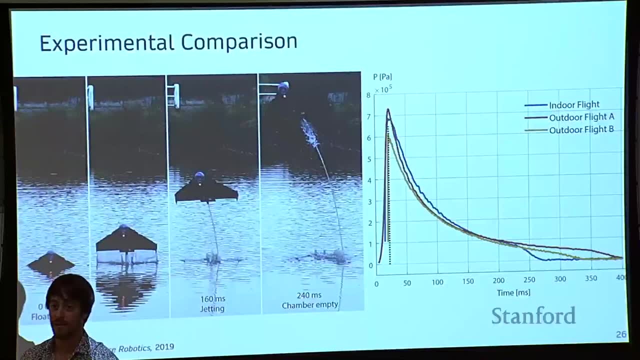 And you can see that within about a quarter of a second, the chamber is empty and we're flying into the air. This process was repeated several times, compared as well against indoor data, to make sure that we understand our system well. And here at that stage, 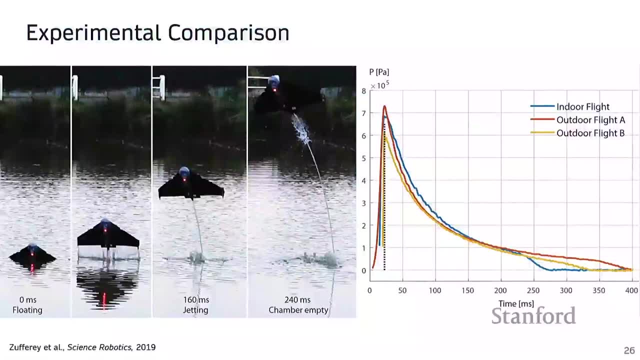 we're happy with the results, but we realized our robot is essentially a floating combustion chamber. We're not really going underwater, So why bother at all trying to escape the water? We'll just stay at the surface. right, And if we stay at the surface, 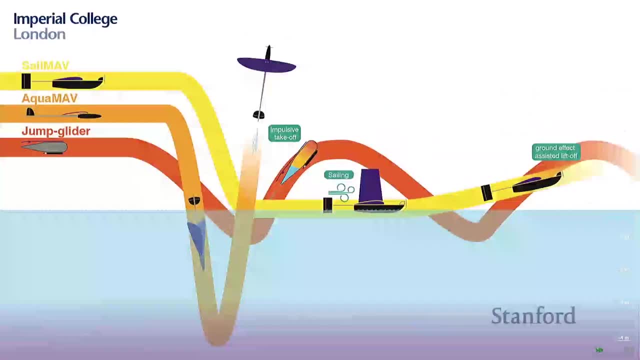 we ease certain some of these constraints and we can do more things, And that's when I developed the SailMap concept. So SailMap is the yellow line that you have here on the screen. It's a robot that we're thinking: okay, let's use those wings for locomotion at the water surface. 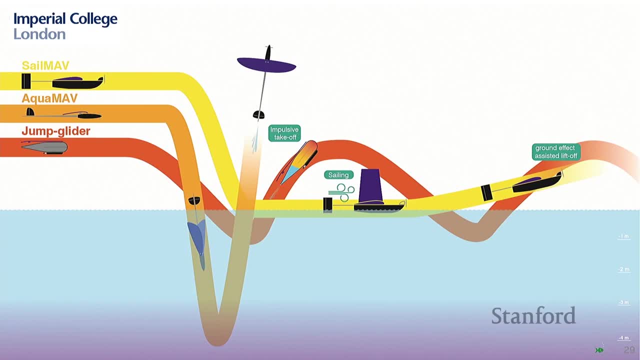 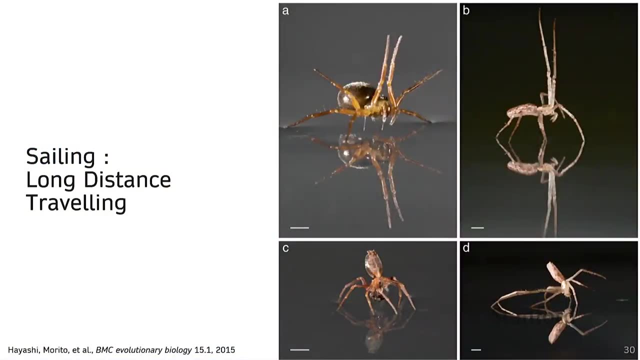 So this robot is able to land on the water and then pivot the wings upwards and essentially do sailing, And so animals have also been shown to do that. So there's spiders, swans, even jellyfish. They're able to do some levels of sailing. 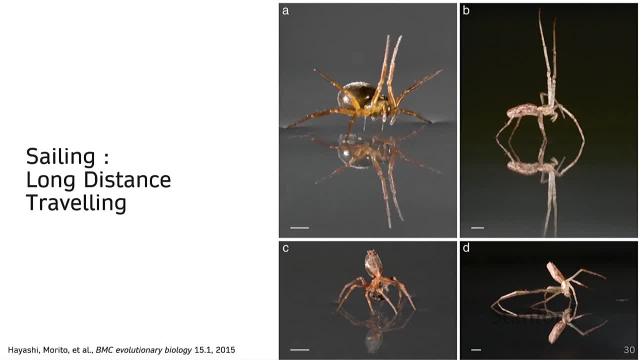 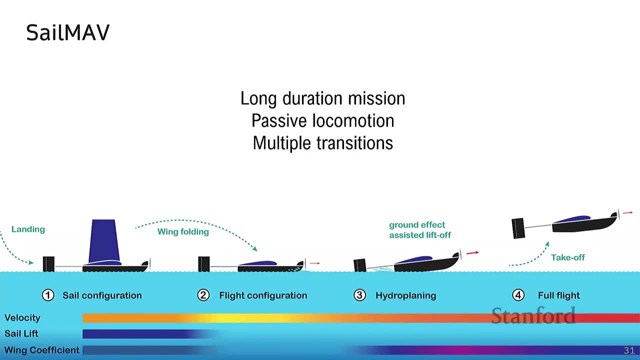 So it's not a completely unnatural approach to solving this problem, And the way this was done in the robot is the following: So the robot lands on the water, The wings become sails. We then fold them back once we've done our science mission. 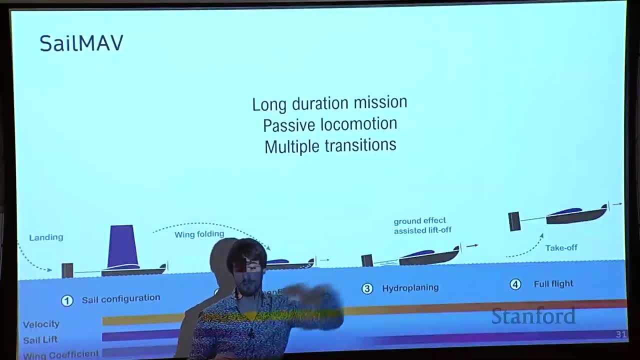 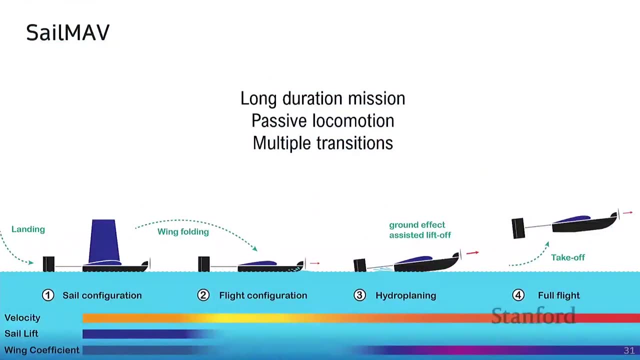 into the wing configuration again, We get into hydroplaning and then we take off, And so with that we suddenly have a robot that can do very long duration missions And so kind of the previous robots were. you know, you put them in the water, maybe a minute. 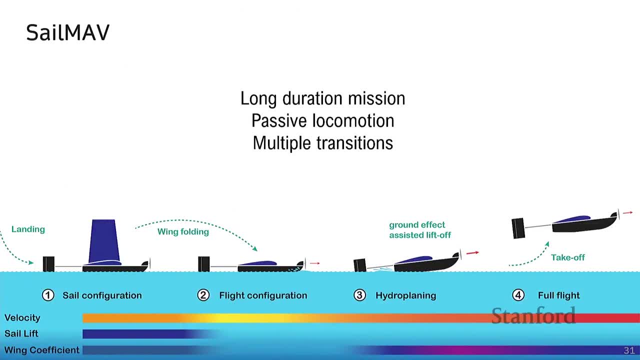 maybe five minutes, ten minutes, but then you know, the system is really not designed to work for a long period of time. And here, suddenly we have something that we could imagine: missions that extend over days, and even more really, because locomotion becomes free. 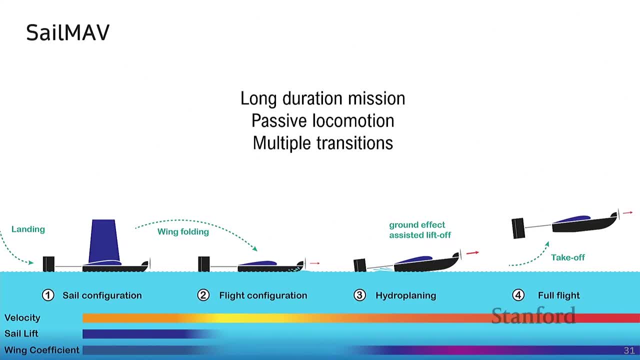 And also with this system we can imagine multiple transitions. There's nothing that speaks against that. So even if you say you're trying to take off and there's a fail there, you could attempt it again. So that robot was essentially an attempt at locomotion with sailing. 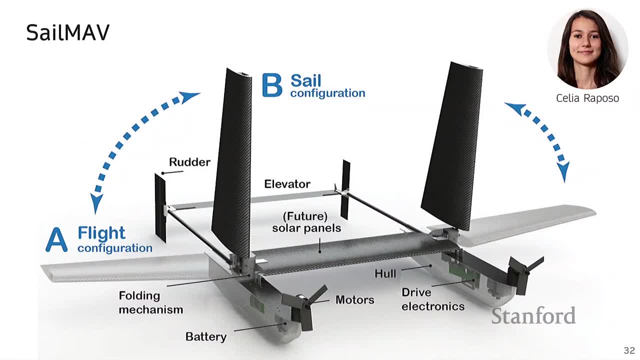 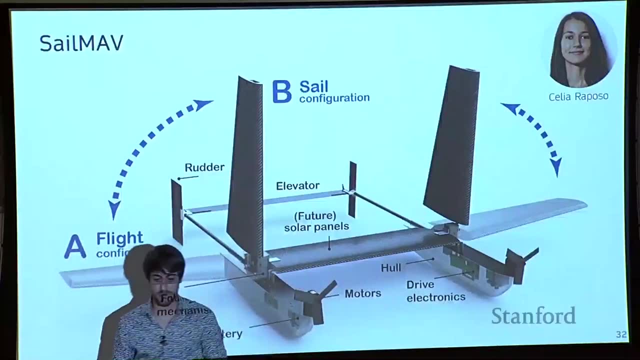 This is what the robot structure looks like, a bit the first concept design. So we have a wing that essentially is split into three segments And the center segment is a highly performant profile, asymmetric, and actually it's a box section, so that's quite nice. 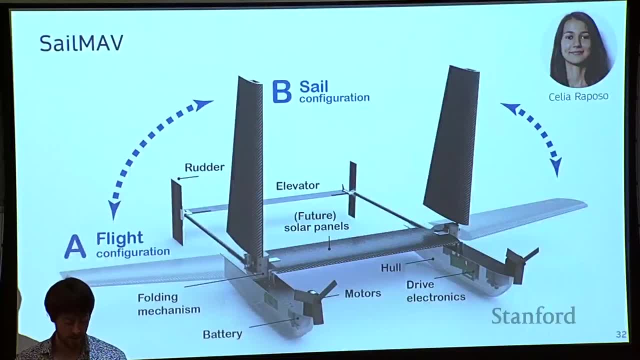 You get a wing that's completely enclosed when we're taking off, And the outside panels are symmetric, And so the reason for that is that when we're in the sailing configuration, we generate equal forces, whether the wind is coming from the left or coming from the right. 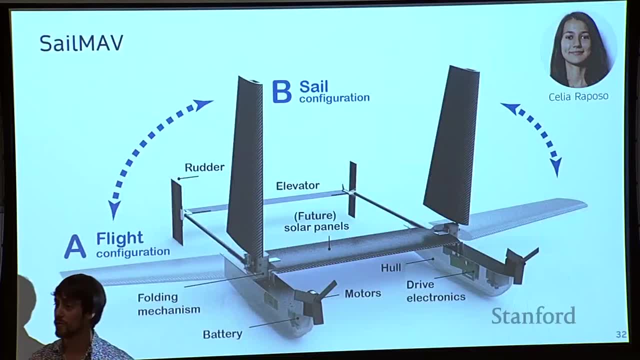 So, yeah, a lot of development had to go into making something like this work. as you can imagine, There's a lot of different components, so I'll talk a little bit about this. One thing that's interesting to note is: not only are we using 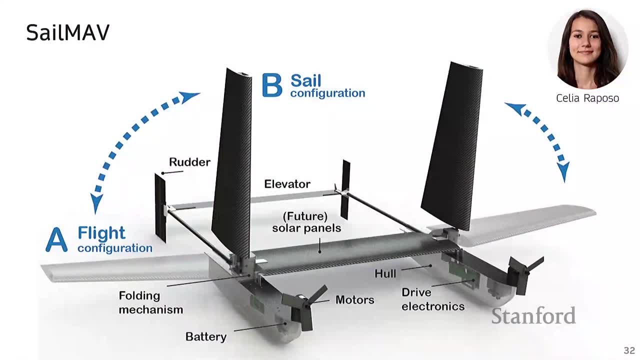 the same wings for sailing as for flying. we're also using the same control surfaces, So the rudder is the same for sailing as it is for flying, And so that's one way to reduce the amount of actuators you have to carry on board. 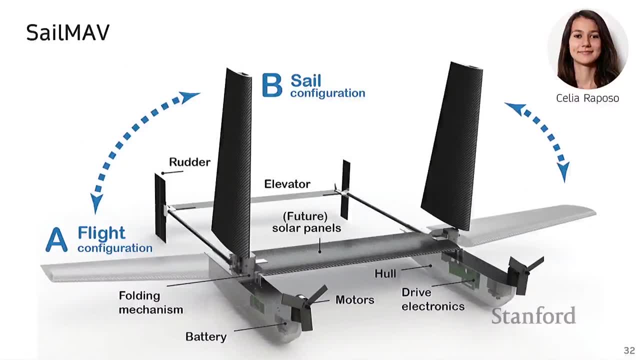 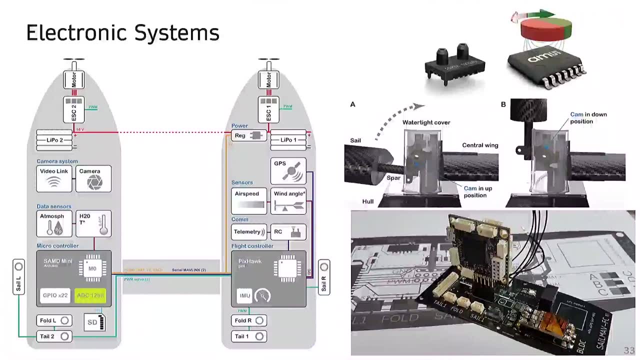 The elevator only serves in flight In the water. it doesn't have a purpose. So, yeah, let's talk a little bit about the electronics to get something like this to work autonomously, because that was the objective We wanted. these robots: You can just launch them by hand. 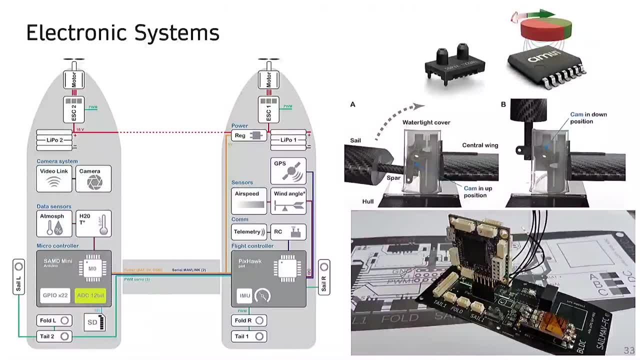 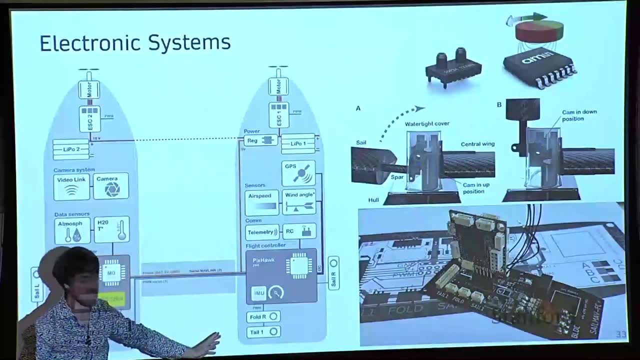 And then they do their own mission. So, as you saw, there's two hulls left and right, And what was decided is to split the electronics into two parts, So you have one half that only worries about navigation. So we have a PX4 controller here running on the Pixhawk. 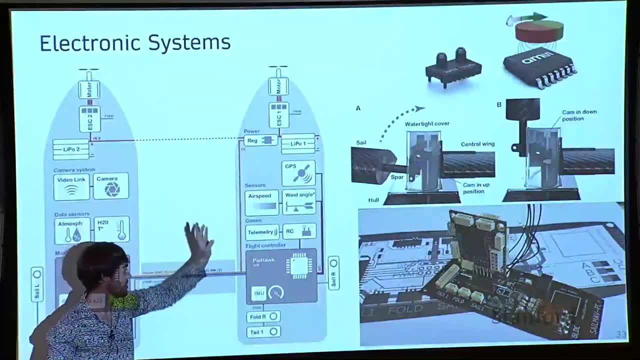 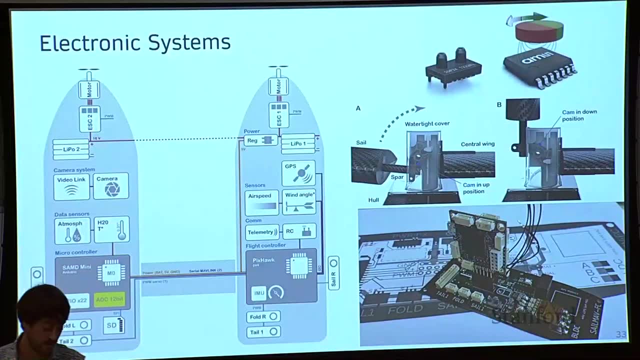 connected to remote control, airspeed, GPS and wind angle sensors. So wind angle was something that you don't typically have in flying aircraft- flying drones at least, And that you absolutely need for sailing, So if you don't know where your wind is coming from, 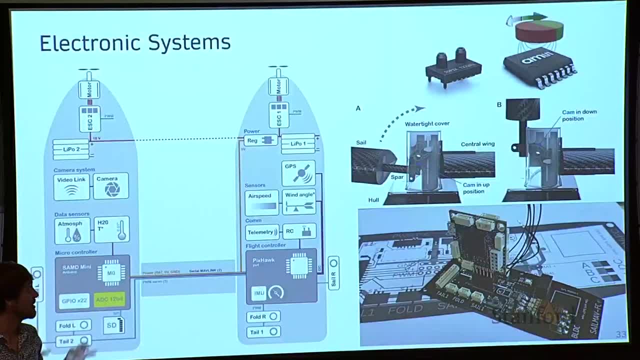 then you'll get very poor performance, And so what we did is we developed a custom sensor for sailing. So this is based on the chip you see up there in the top right. So the way this works is you have a hull effect encoder. 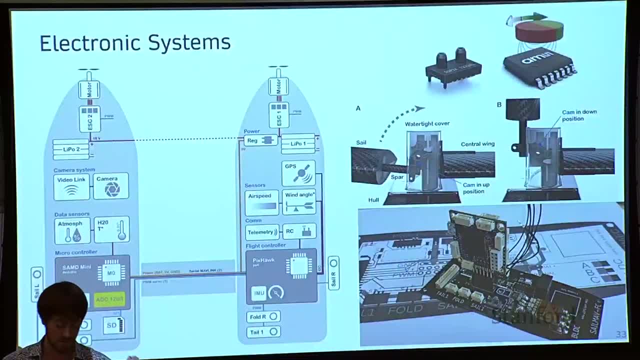 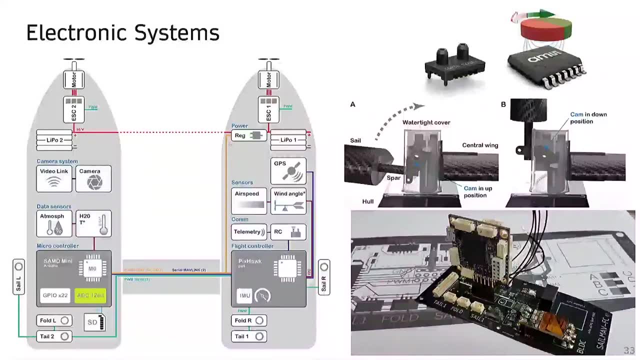 So this chip just basically gives you the very precise angle of magnet that you spin above it, And so what's nice about this is you can have the sensor on the inside of the robot and the magnet on the outside, So even if water comes there, it doesn't really matter. 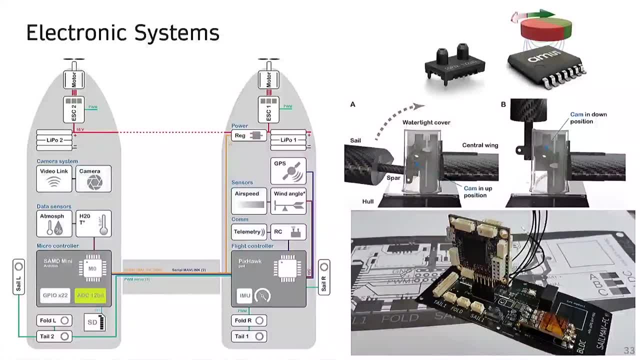 So with that we're able to get quite tiny sensors that were able to give us the wind angle, And the other side of the robot was essentially worrying about the scientific payload And the idea is to really decouple these two, So it had its own microcontroller. 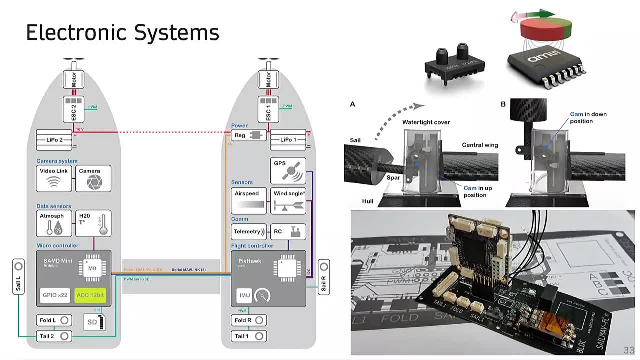 just communicating with the flight controller to know, for example, the geographic location of the samples you're taking, and so on. So yeah, all of this was developed with some custom electronic boards that were fixed upside down inside of the robots, So if any water comes in, it doesn't actually. 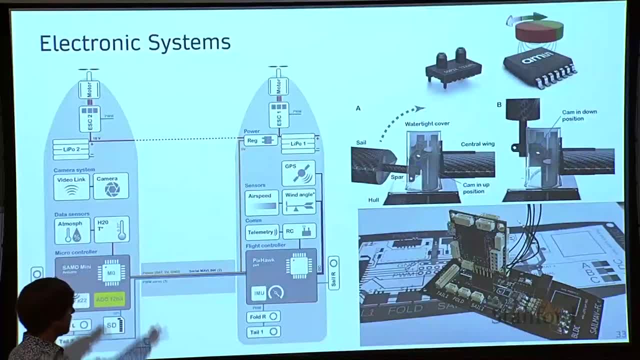 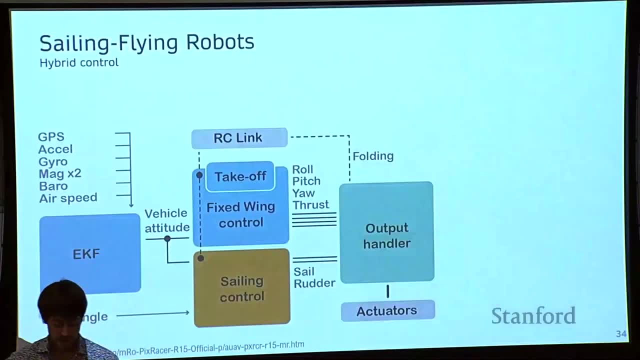 touch the electronics And yeah, I'll spare you the detail on the mechanical design- some essentially locking systems for both positions up and down. The flight controller had to be modified quite a bit because flight controllers don't handle sailing at all. PX4.. 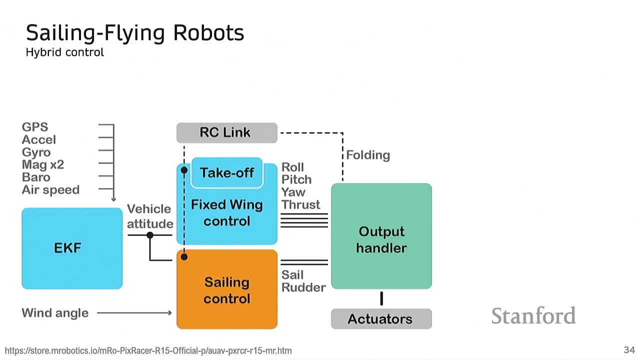 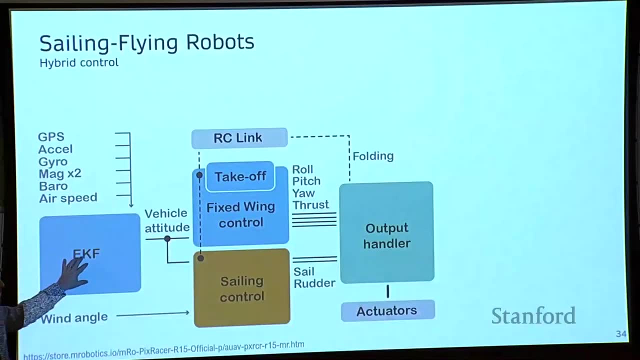 So what we did is we modified this code. I mean, it's basically just a very rough representation of how PX4 works, But essentially you get your sensor data, run that into an extended Kalman filter. You get your vehicle estimation, attitude estimation. 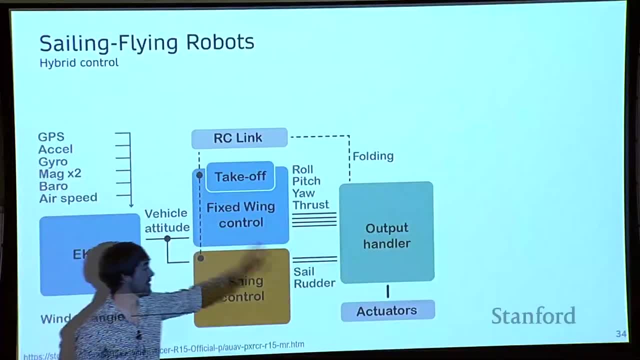 And that typically goes into a fixed weight controller and then to the actuators. And so what we did is, essentially, we added this sailing control block that we designed within PX4. that would, in addition, take also the wind angle, which we're not using in flight. 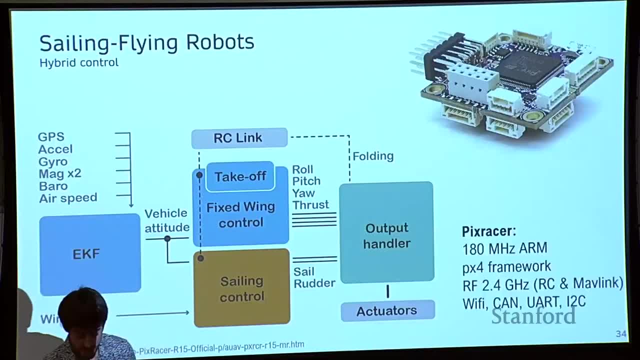 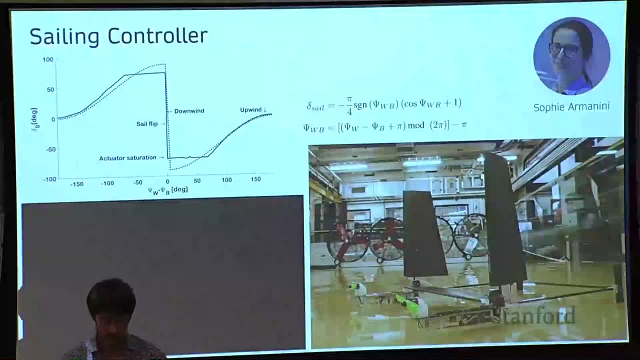 and output the actuator values. All of this was running on the PixRacer here, one of the tiniest flight controls that you can get, And yeah, with Sophie here we've been doing a lot of the sailing testing. So at Imperial College they didn't let us flood. 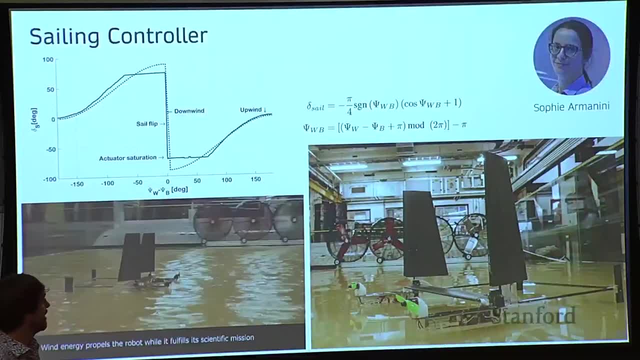 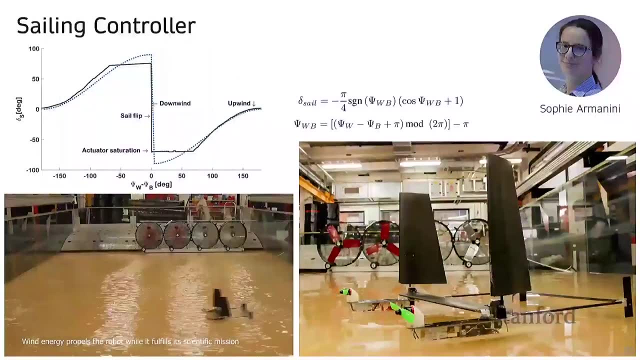 the wind tunnels there. So what we did is we put fans in the tank that we had, which was a very crude approach to wind tunneling, But essentially, with that, we're able to test our autonomous wind controller, And so there is a bit of challenges. 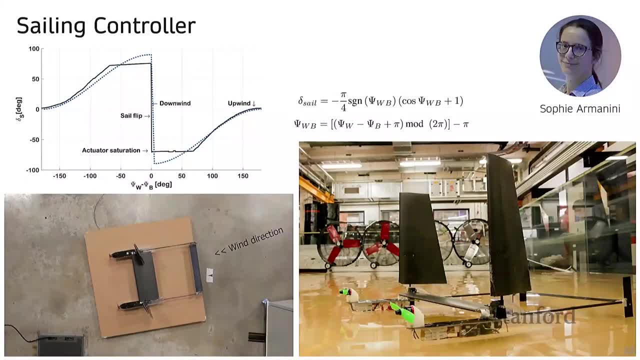 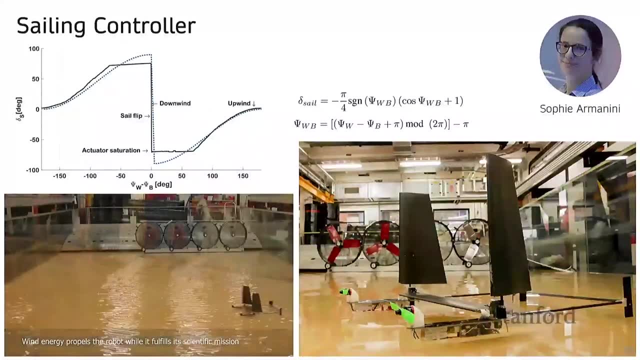 into designing these controllers as well, because your wings don't have full span, So ideally you'd have a wing that you can pivot 360 degrees, And typical servos don't allow you to do that, So there's a bit of work that went there. 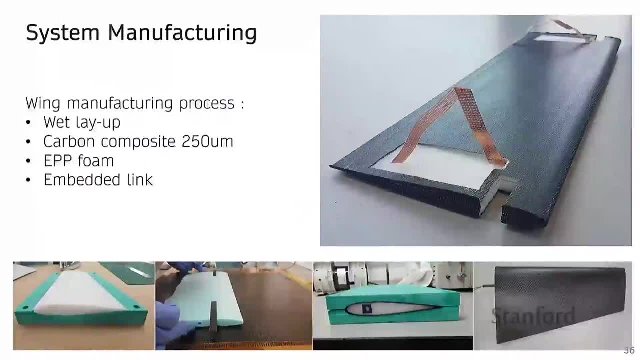 into getting the right controller. Also a lot of manufacturing for a system like this. We wanted the system to fly, So you need to go with light materials, One process that we've developed kind of over my PhD, which is nothing new, but we're able to do this. 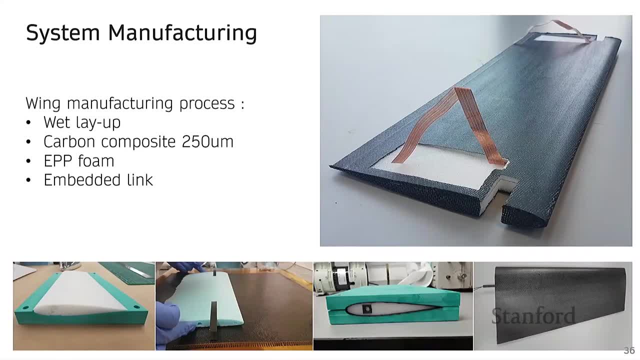 in a matter of hours- so that was nice- is essentially to produce these wings. So what we do is we CNC cut a foam core out of EPP foam, which is a foam that doesn't break very easily, And what you do with that foam is you put it inside. 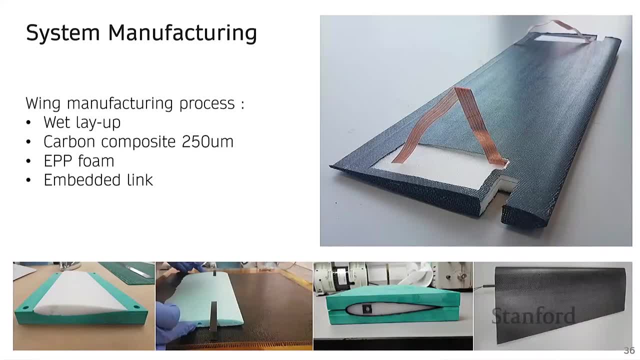 of your previously cut molds. You put your fiber around it which you've previously wet with epoxy adhesive. You then wrap the fabric around, put it in the mold and cure it all together, And so some of the advantage of this is just through. 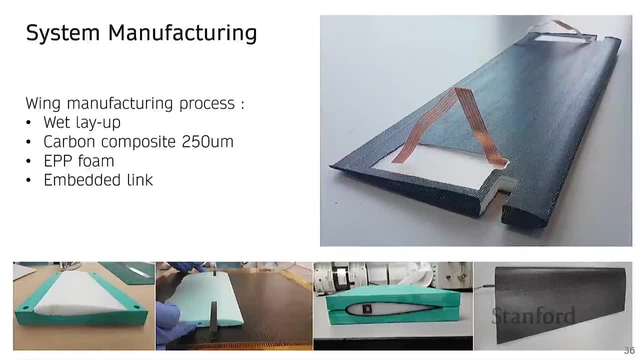 like some vacuum Pressure, we're able to get those wings, And one nice thing about this process as well is we're able to get electronic components. So here, in this case, it was just an electronic bus that was going through the wing And that was important to be able to transmit. 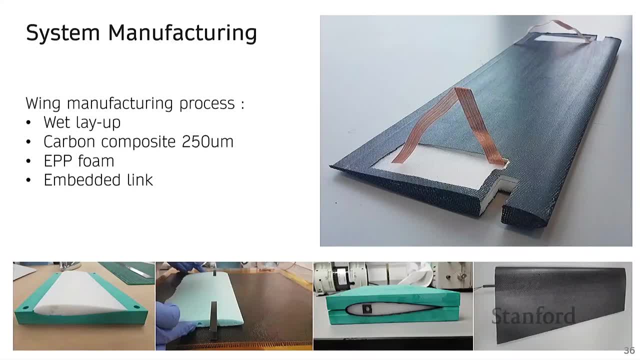 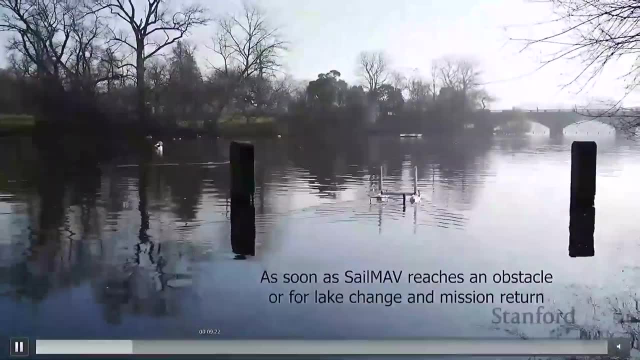 the signal from the left to the right of the plane. Yeah, So this is actually. let me stop this. Well, that's all right. This is in Hyde Park in London, where you're allowed to sail, So we're testing the robots there. 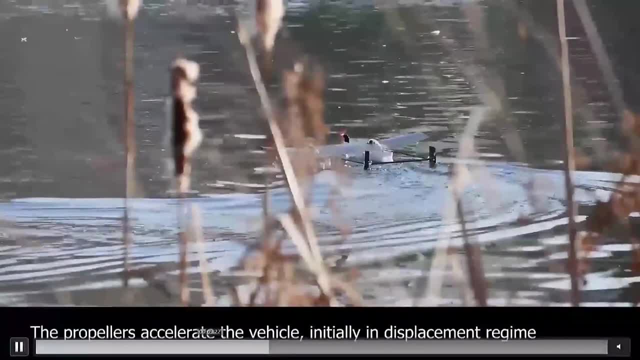 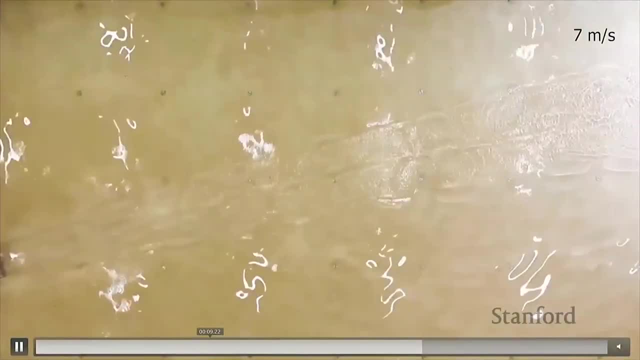 And here you see the robot in flying mode. So it's accelerating And it gets to hydroplaning speed, which happens at around 6 to 7 meters per second. And finally, we're testing the transitions to flight. We're not allowed to fly in this pond. 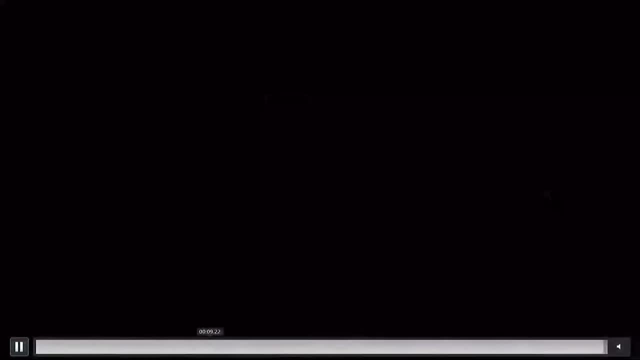 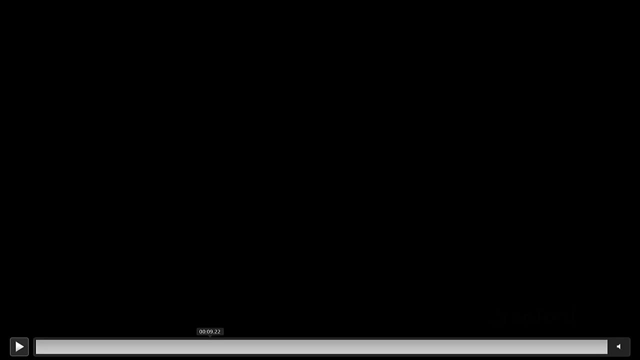 So we're obviously cutting off the robots. So that's why we're not showing any of the flight phase. No, but, jokes aside, there's still a bit of work to happen on the flight phase And it's still an ongoing project. 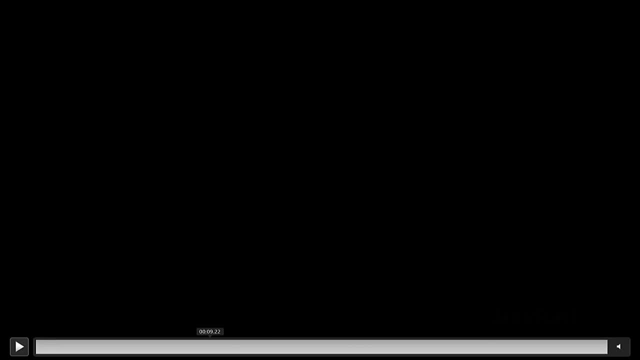 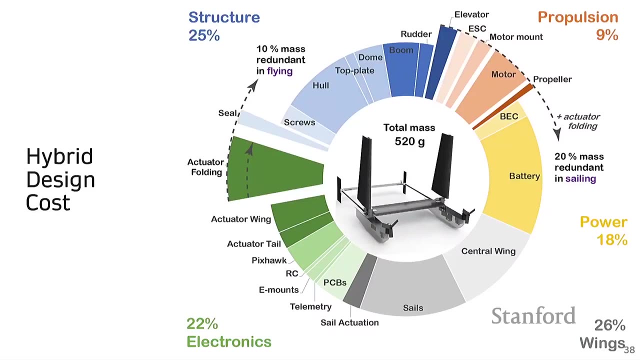 One thing that I think is interesting, and I think is particularly important when you do these hybrid robots, is: what is the cost? Because at the end it's great, It's like, oh yeah, now we have this robot, It can fly. 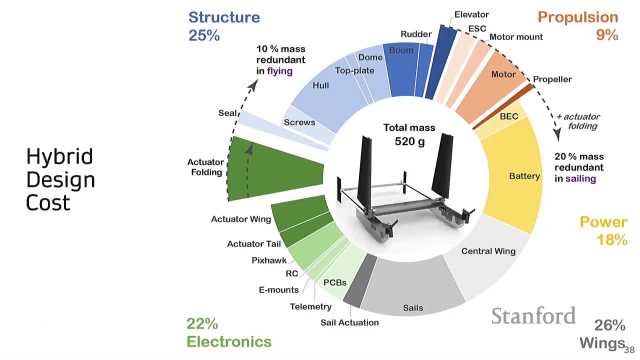 It can sail, But what am I paying for that? What is the price? And so what we did, the way we approached this is, we characterized the weight of every single component we had on the robot and then tried to look: OK, which components are redundant? 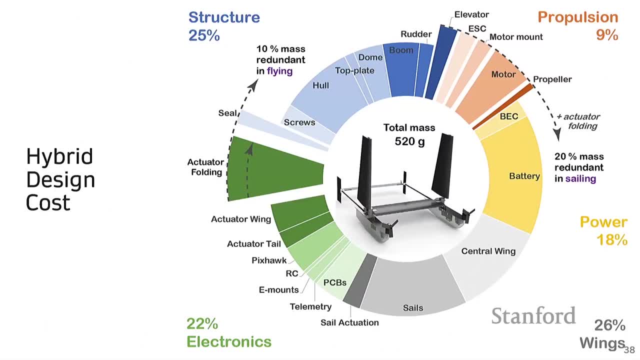 Which components would we actually not need? And so what we see is that in flying, we have about 10% extra mass, which is a small penalty, but it's still quite significant, And in sailing we have about 20% of mass. 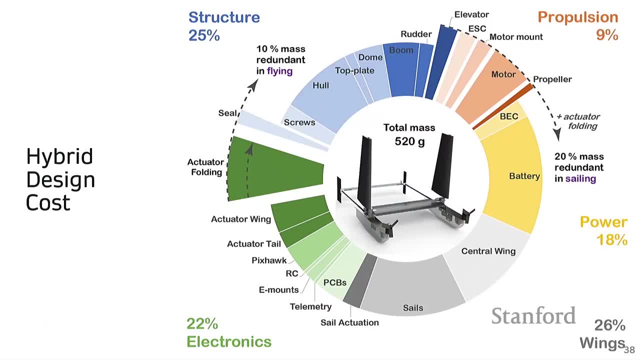 that essentially does not serve any sailing purposes. In sailing it doesn't matter too much, So this plays rather in our favor, And essentially we've been looking at these metrics for most of the hybrid robots. This then led also to field work. 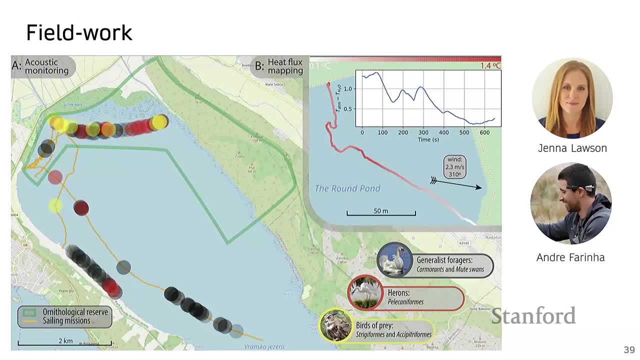 So this is in Croatia about two years ago, And one thing that's nice about sailing is it's silent, So you don't have any propellers that are spinning any underwater screw, So you can actually start to listen to animals quite well. 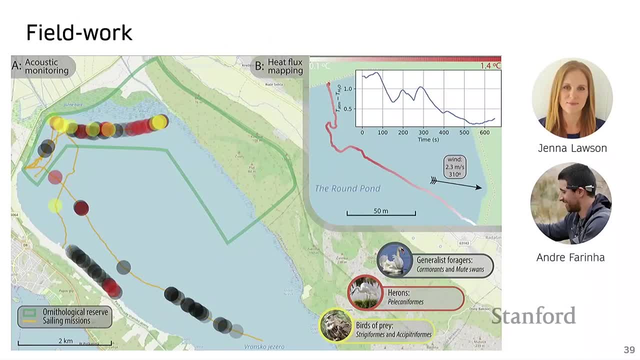 So what we did here is we put a hydrophone and a microphone on the robot And we had it sail around in this lake for about two hours. So it's quite a large lake And essentially here we're able actually to extract which species of birds. 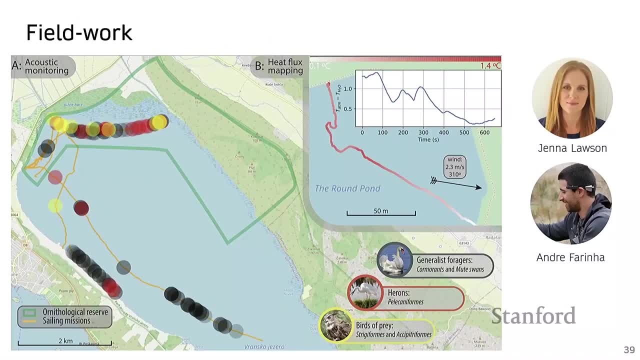 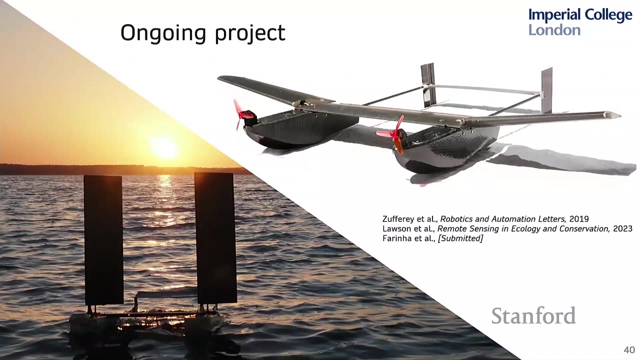 were on this lake and also underwater insects, And so this was published recently. It was in partnership with Jenna and Andre. Jenna was a biologist in the lab with Mirko. So great, Great work, And it's led to three publications. The last one is still in process. 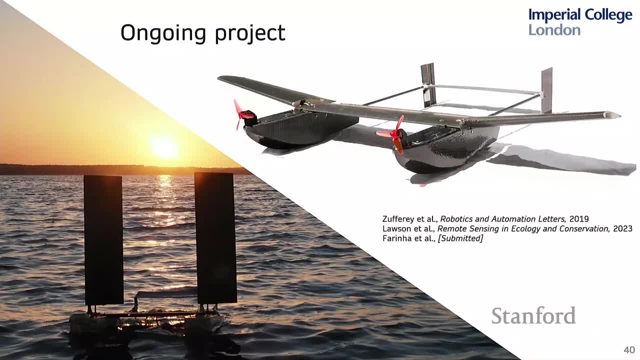 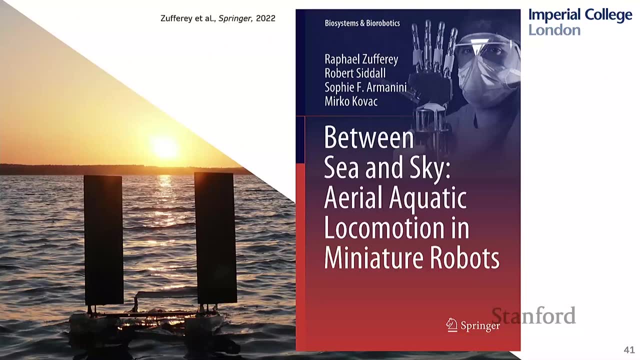 And it's a project that's still ongoing, So I'm very excited about this And I hope to see more things in the future about it Also led to a book publication which I wrote with Rob, Sophie and Mirko just after the end of my PhD, when COVID hit. 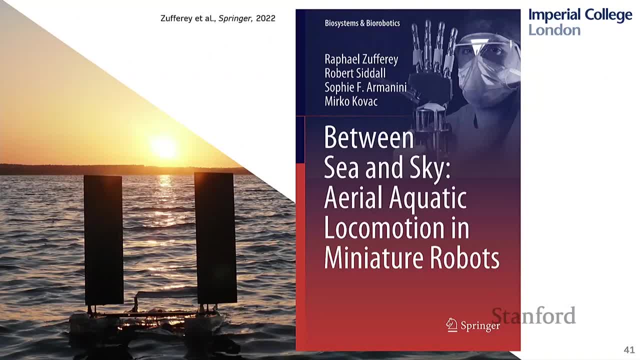 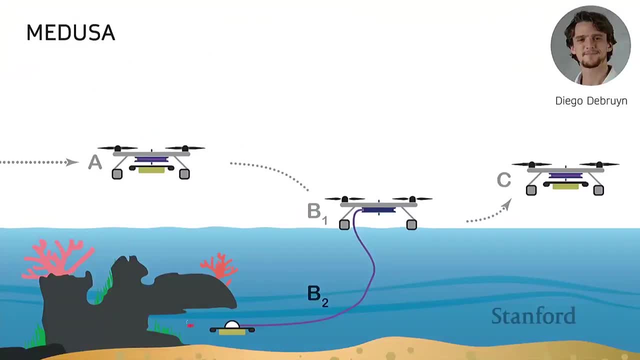 So it was a nice side project And it combines a bit the things I've been saying so far. I think one project we should still talk about It's Medusa. So Medusa is a dual agent robot, And so the idea is to look essentially. 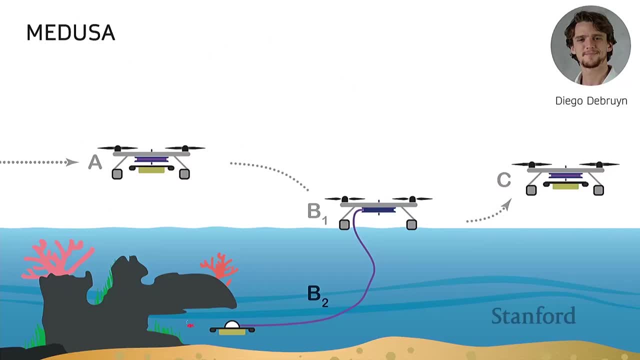 at drone technology, at quadrotors, to solve this similar task, And what we wanted to do is to have a robot that can fly, land on the water and then deploy this tether to actually access locations that underwater that you could not with just simply a quadrotor. 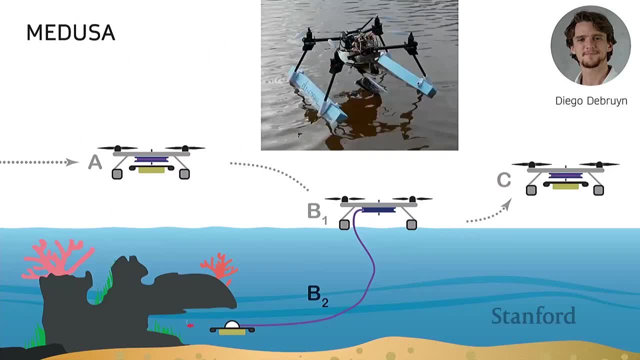 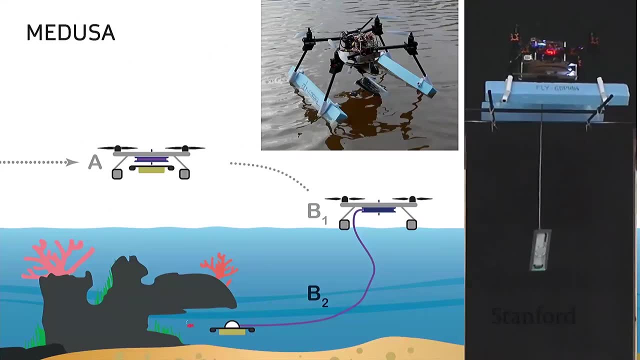 And then fly off. So the platform looked like this, floating here in the lake, And we had this pod that we could deploy from the drone And this pod here looks like not much, But you'll see we've actually worked quite a bit on this. 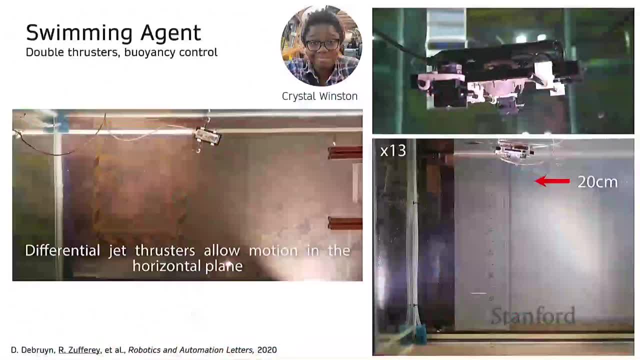 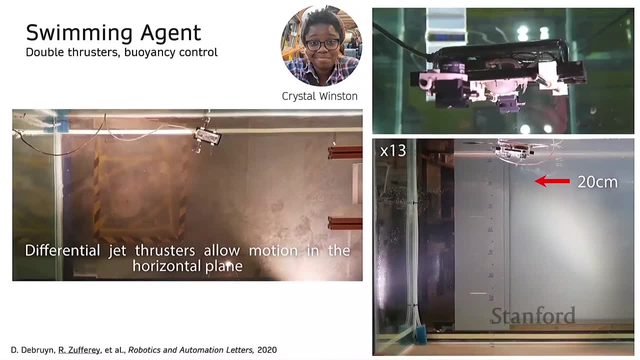 And so this is what I call the swimming agent, Because actually there is quite a few things it could do, So it could regulate the height at which it was swimming, And so for that we had this soft membrane And we would control the pressure inside of the robot. 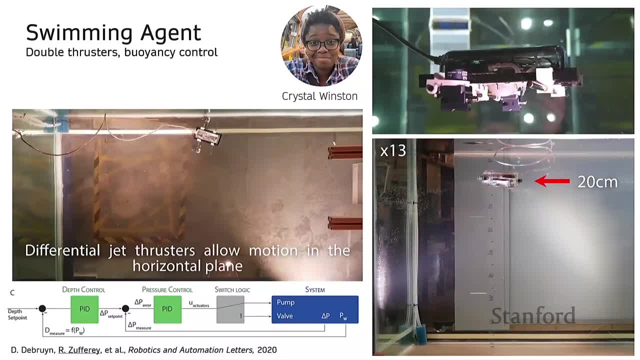 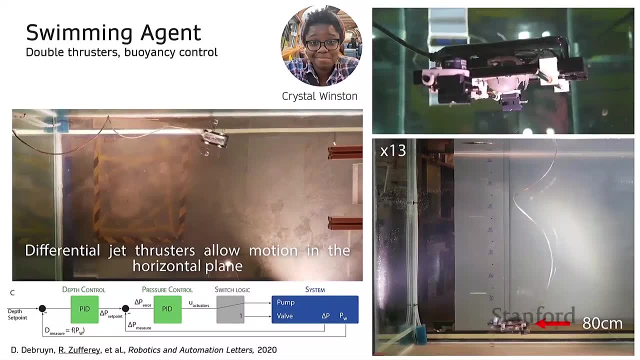 to move up and down. This was controlled through a double tether. It was a PID control loop and was able to essentially regulate to a certain depth. We also had jets on the robot And with that we were able to navigate in x and y. 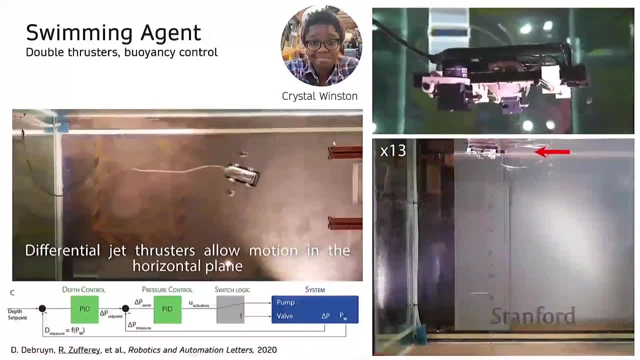 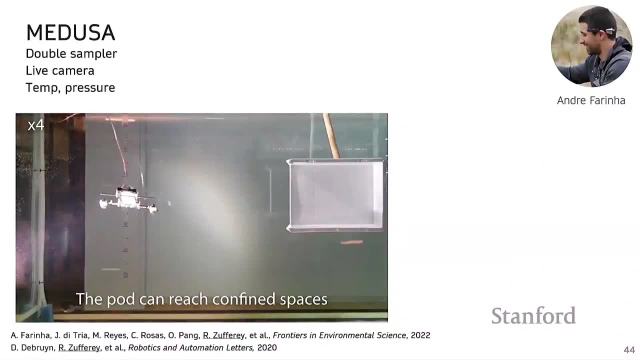 to the position that we wanted. Of course, you're limited by the tether, So it's still within kind of a 5-meter sphere. You can go around the robot, And I think what's really nice is suddenly we have a way to get live video from underwater. 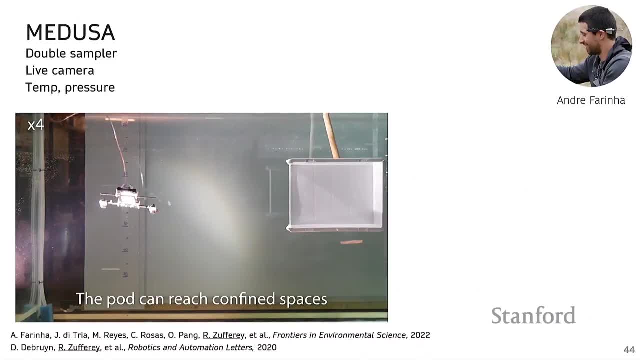 relayed back over the robot, over the drone, back to shore. So that's quite unique Because typically underwater robots they don't have a video link, They have just a very poor way of communicating and transmitting data, So usually you don't get video. 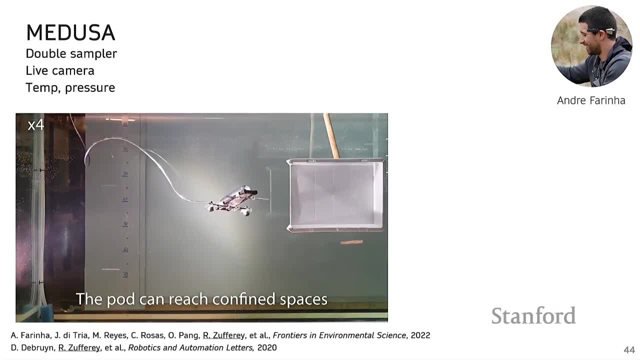 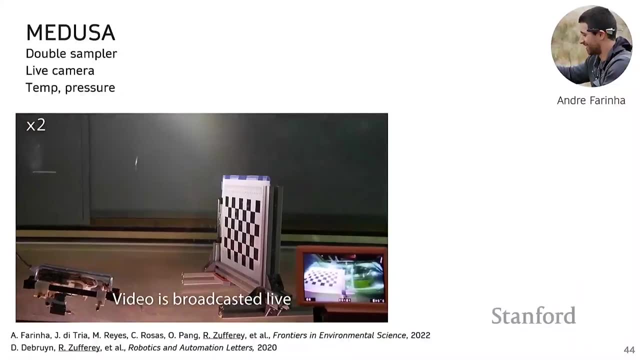 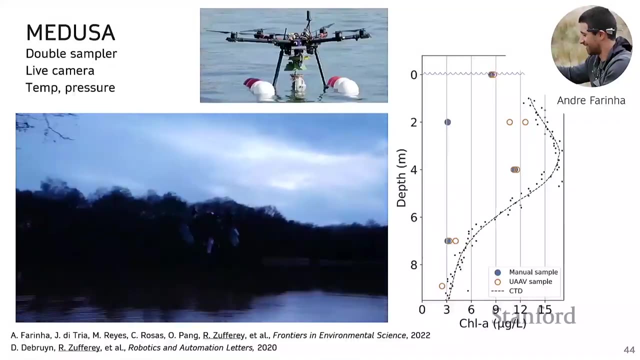 So that was nice to see that we're able to get that And we're able to navigate the robot into relatively tight spaces through the xyz control And here relay video data back to the user and doing also some flights outside. This was also tested then in Switzerland. 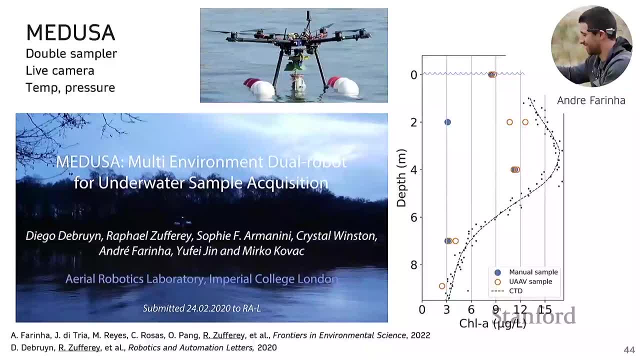 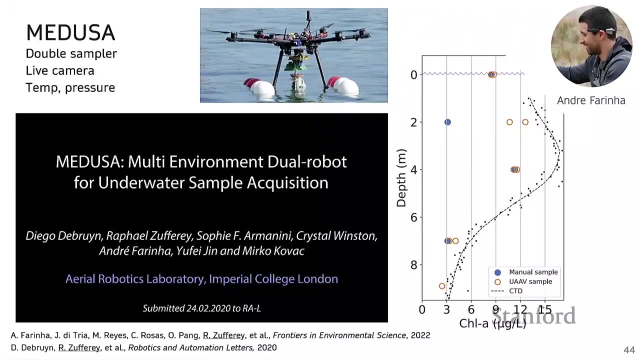 on a lake where we were able to compare chlorophyll content within the lake at certain depths, And this was compared with other types of measures that biologists were doing there, which are typically manual, very big sensors and quite expensive to deploy. 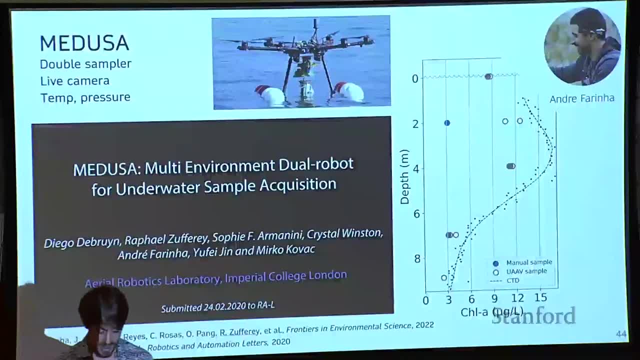 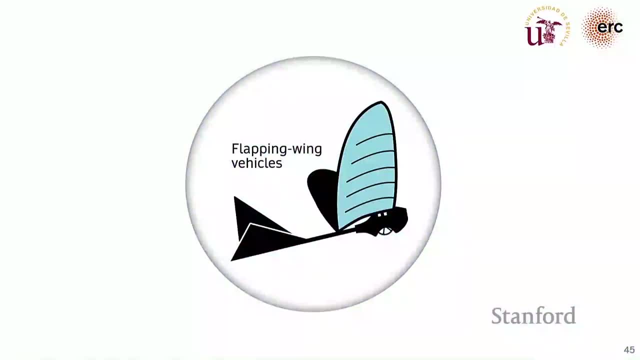 The robot has evolved a little bit, but I'll spare you the detail, And after that I moved on to quite a different project, working on flapping wings, And flapping flight is something that Anibal Ollero was doing a lot in Spain. 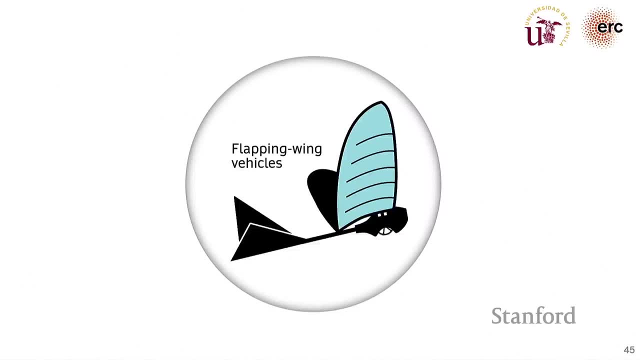 And when I arrived I realized, OK, well, this is cool, but why do we actually bother with flapping flight? I mean, propellers are really good. We have drones everywhere. You can go to the store, buy one for $300, right? 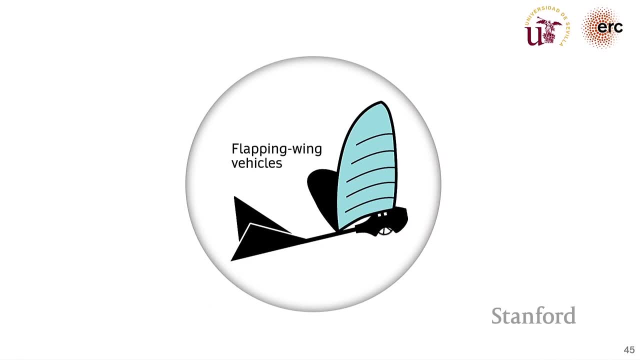 So why do we bother with flapping flight? And I think there's very good reasons. First, and I think it's one of the most important, it's safe, And I really mean that. So we're having these robots about this big, flying around us. 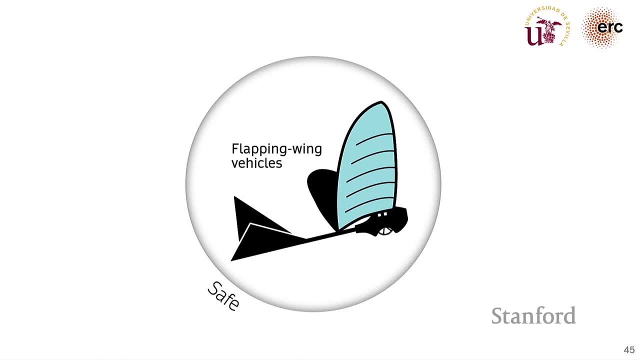 and you can catch them in flight. So it's really something that you're not worried about, And this is due to the fact that we're using the low velocities of the wings compared to a propeller. That comes with it. It's also quiet. 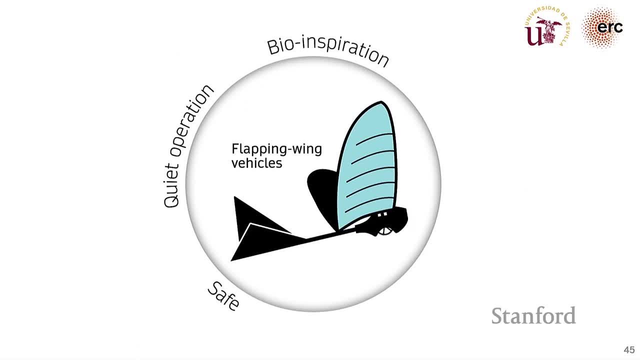 You don't have these high-spinning propellers. It's bio-inspired, so you can actually look at animals and copy to get inspiration when there are certain metrics that you're having a hard time to figure out and to model. It does show very high maneuverability potential. 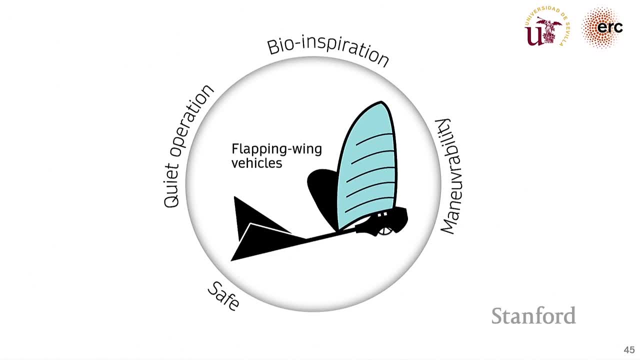 So you can flap one wing on one side and really stop flapping on the other side and therefore get really high turn rates. And finally- and I think that's really important- you can fly at very high angles of attack, So that means you can really have a robot. 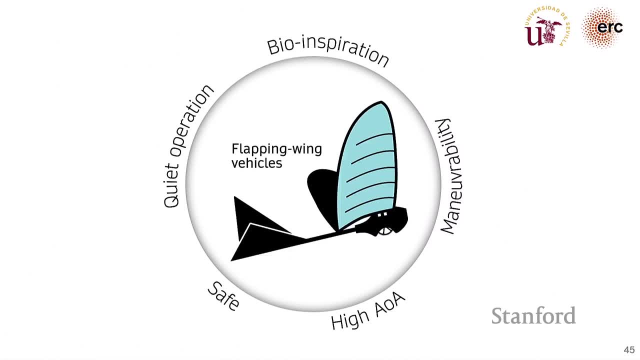 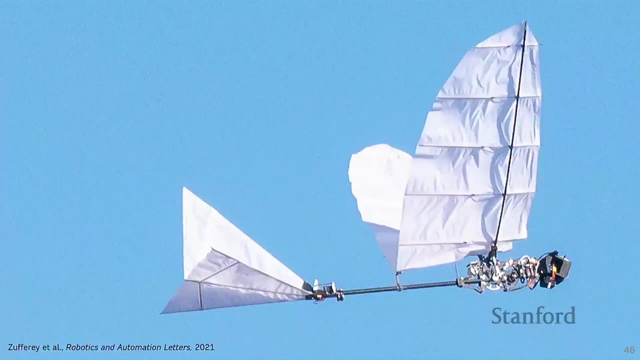 that flies slowly at high angles of attack and quickly at low angles of attack while remaining relatively efficient. That's the hopes. Birds are really good at this. Robots still some ways away from that, And so this is the robot that we published in 2021 in flight here. 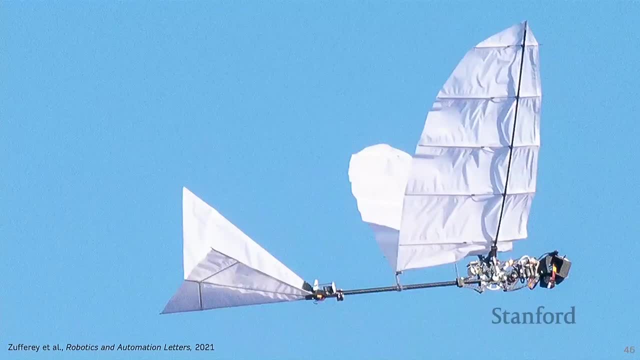 So we're talking about 500 grams- this big- And one of the questions that we had is: OK, how do we do physical interaction with this? It's great, but we throw it by hand and then it crashes on the ground and that's the end of it. 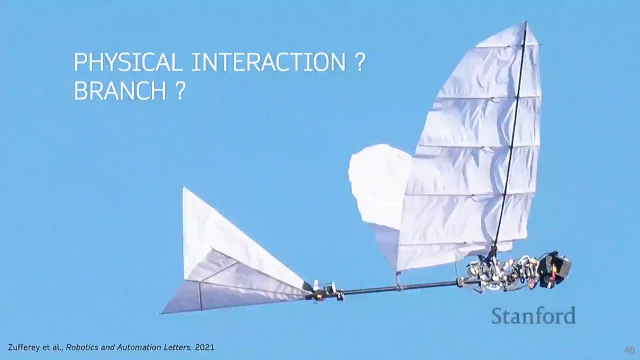 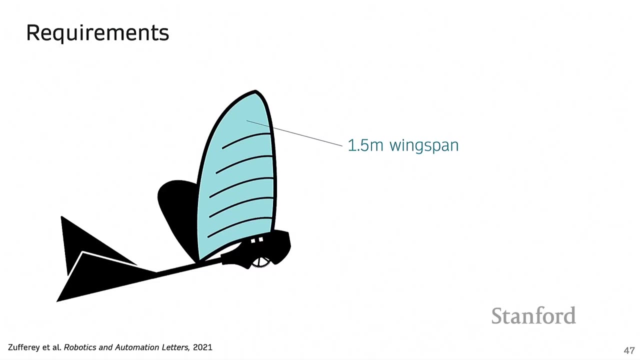 And, specifically, how do we land it onto a branch? So the requirement that we had to be able to do this is develop a robot that has this 1.5-meter wingspan, 500-gram weight, but also 500-gram additional payload. 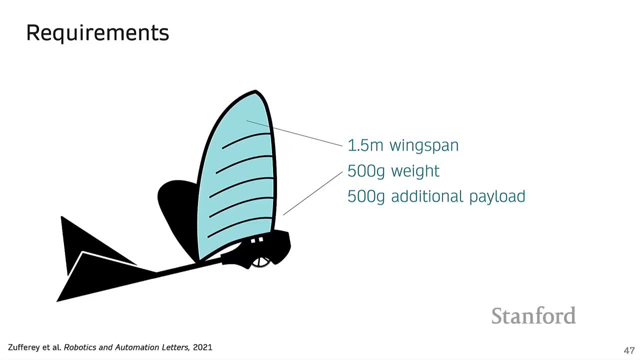 And so that was really important, because at that time, most flapping wing robots were not able to carry so much extra mass, And so a lot of work went into getting this additional payload, which meant we can actually start to add stuff to our robot. 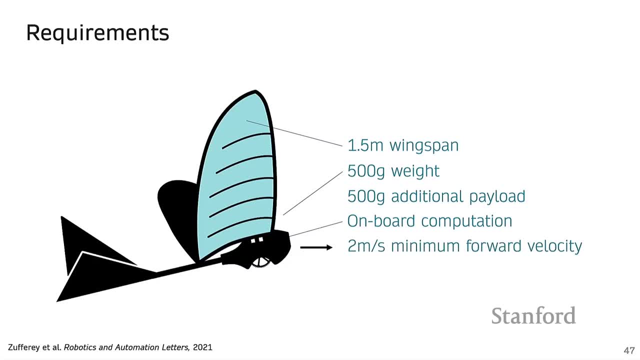 Onboard computation and, very importantly, we had a 2-meter-per-second minimal forward velocity. So that's really slow. That's this you walking quickly type of speed. So that's really good news if we're trying to attach to a branch a static object. 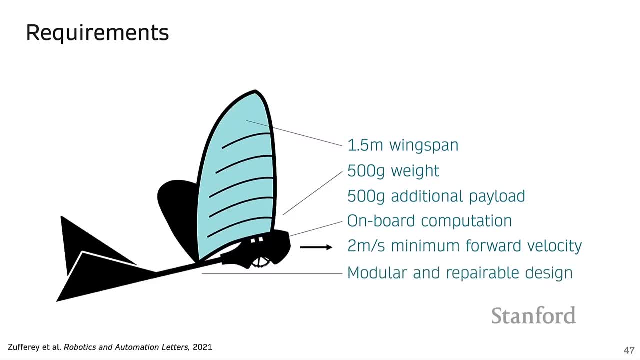 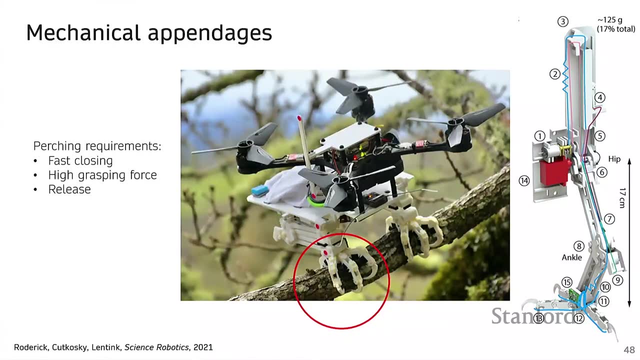 And, finally, a modular design, important for when things don't work out. So, of course, when we talk about, of course, when we talk about mechanical appendages, one great work comes to mind- led here, of course, And what I want to do is look a bit more. 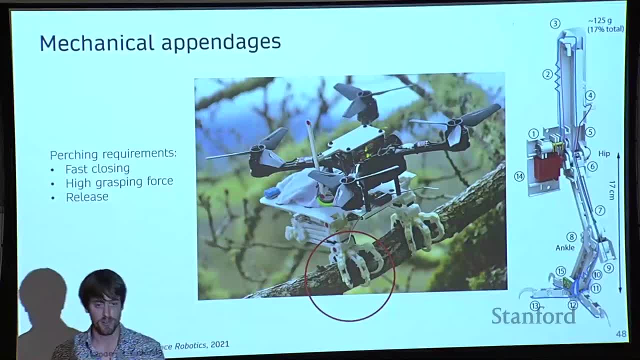 at the perching aspects, at the claws themselves, And we see that there is several requirements that we need to be able to do this with a flying robot. So first we need to be able to close very quickly onto the branch. So that's very important. 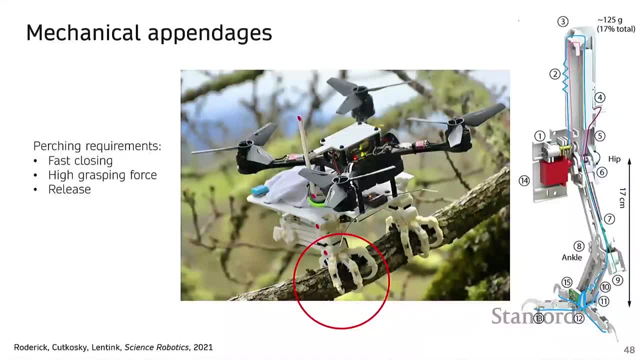 And same applies for flapping wing robots. We need high grasping force, because we need to be able to stay on the branch and not slide off, And finally, we need to be able to reopen the claw, Otherwise we're just landed. 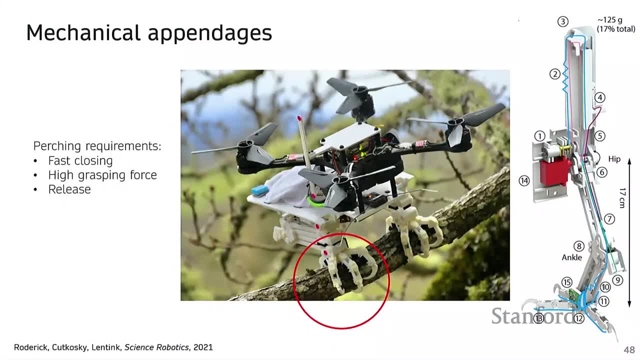 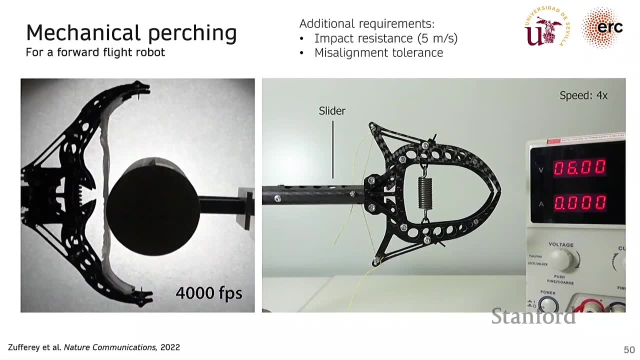 We're just staying there. And so we worked on a similar concept in a way, if you want, But we had slightly additional requirements, I would say, for our forward flying robot. First is the impact resistance that we needed, So suddenly we needed to be able to stop. 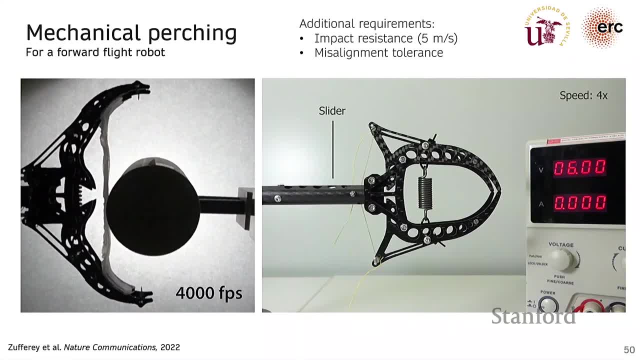 this forward flying robot. And finally, one important aspect was the fact that our flying robots, we can't control them in position very well, So you get them into trajectory, but there's still there's oscillations in flight, And so that was a problem. 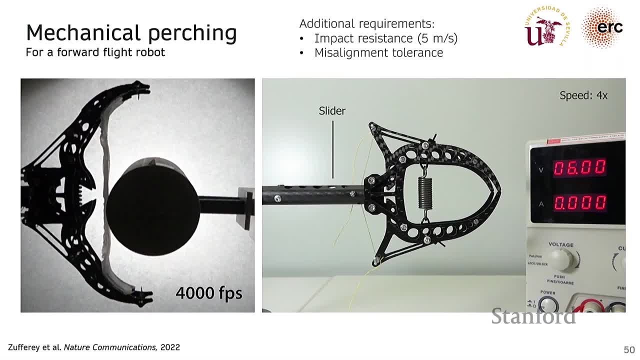 And we're able to find a solution- that I'm presenting here- that was able to tolerate this misalignment. So here you see this in 4,000 frames per second. The branch hits the center of this claw, which is bistable. 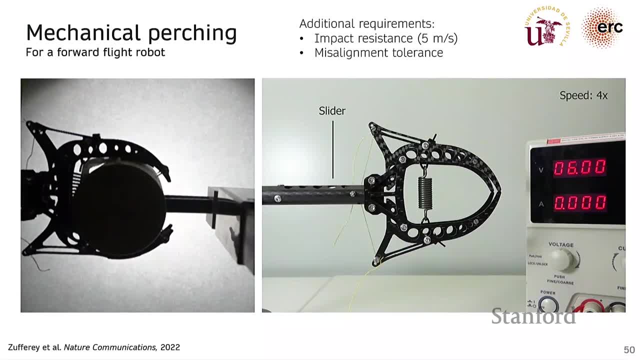 And the moment we hit the center, the claw actually closes within 25 milliseconds. And, of course, this was essentially pulled open with some tendons, And these tendons need to be able to be pulled to reopen the claw. So this was something that we implemented here. 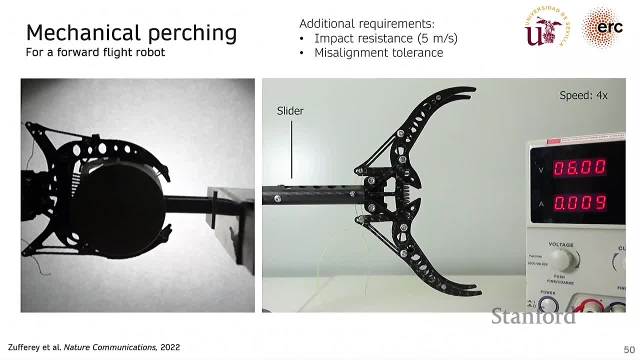 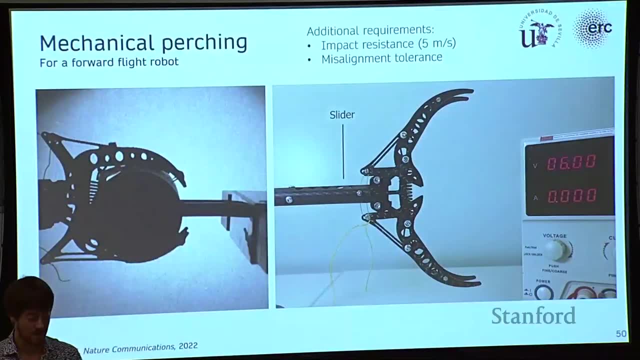 So we have this integrated slider mechanism within the leg. It charges by opening the claw and pulling on the tendons and then releases the tension within the tendons. So they're now just loose And you can come with a branch and essentially close. 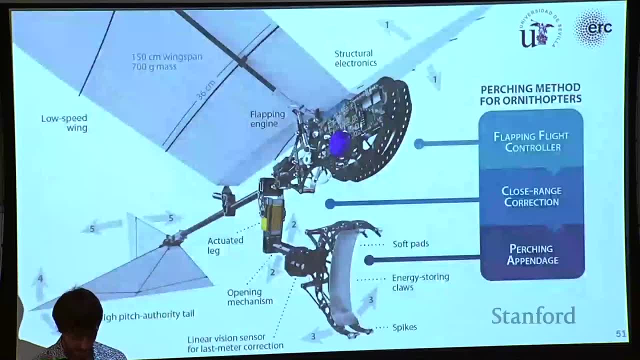 very quickly. So we integrated all of this within our forward-flying flapping wing robot And we realized to be able to perch something like this. there's really three components that need to work together. First, we need a flapping flight controller. 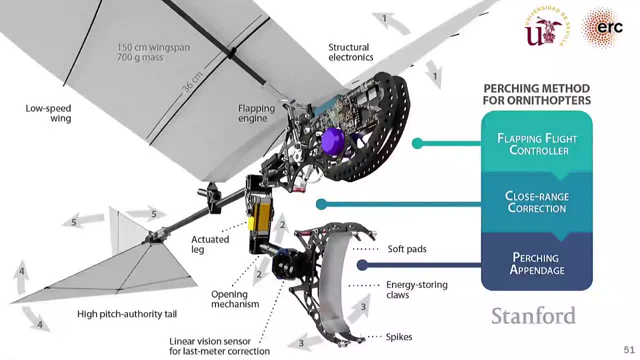 that is able to get us close to the branch right, Because if you don't get that, then nothing is going to work out. And then you have these oscillations because of flapping flight. Birds are pretty good at this, Robots- we're still a bit further away. 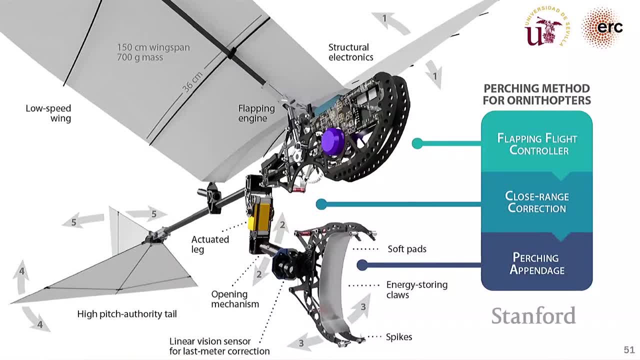 So your center of mass actually moves up and down as you flap at 4 hertz, So it's relatively quick. So you need some way to correct this misalignment. that's bigger than the branch that you're trying to perch on, So we need a close-range correction system. 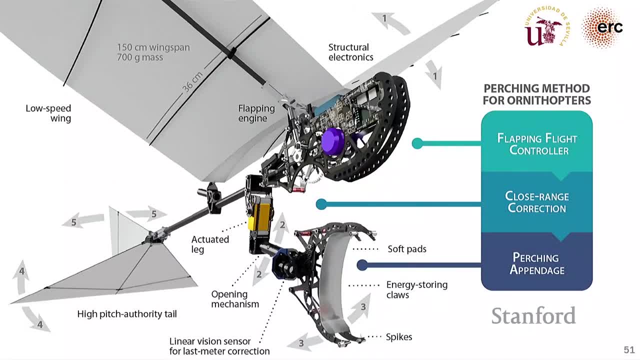 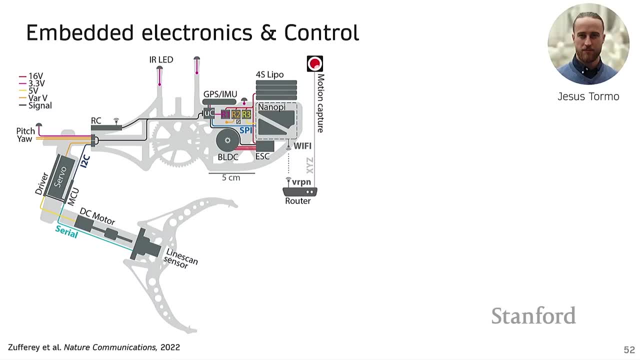 And finally, you need to actually perch on the robot, Perch on the branch. sorry, A lot of electronics goes into designing something like this, So the way we developed this was essentially have a network of electronics that's sitting in the head of the robot and that. 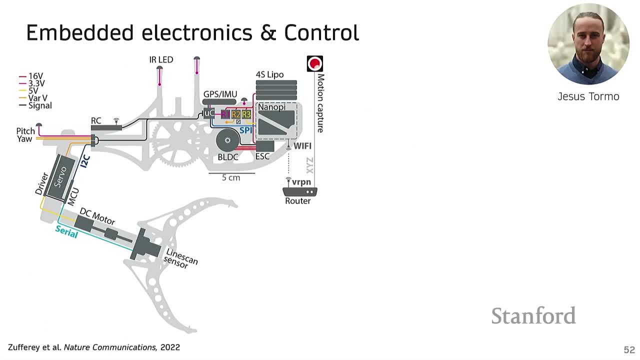 is connected to this claw, that actually carries its own microcontroller and own controller. We decided to go with a structure that's an entire printed circuit board actually, And so it's a really nice thing, because, at the end, printed circuit boards are glass fibers, right. 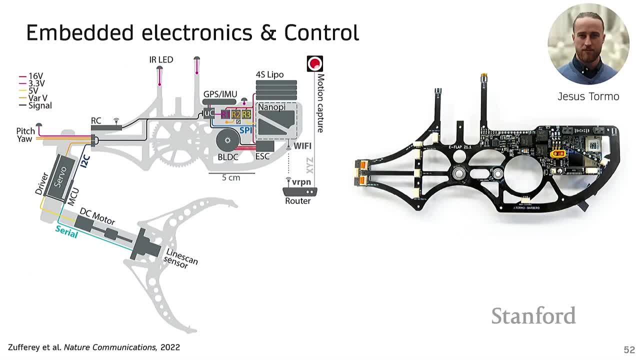 So structurally they're quite good. They're a bit heavier than carbon but they're able to take very high forces, And so most of the sensitive electronics were in the front of the robot, carrying actually a small Raspberry Pi, And the connectors were in the back of the robot. 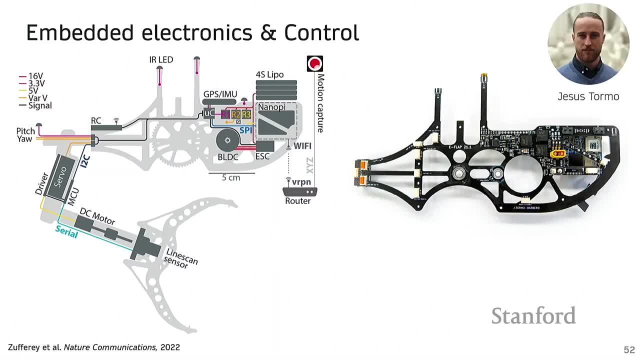 So we're minimizing the amount of wires that we have on board In order to manage flight. so this was done in a motion capture system. So obviously the next step is to do this outside, But in the scope of these experiments, we're doing things in a motion capture system. 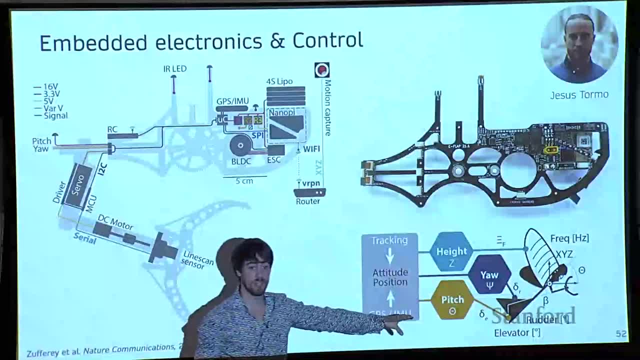 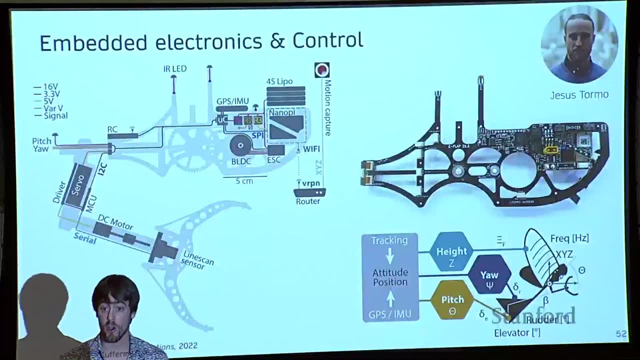 And what you're doing is you're essentially controlling height, yaw and pitch of this robot, And you're doing this by controlling the frequency of flapping, So that regulates your height, And the yaw and pitch is controlled more by a standard aircraft with a rudder and an elevator. 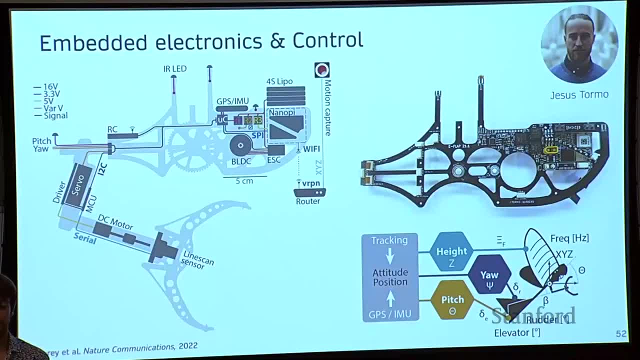 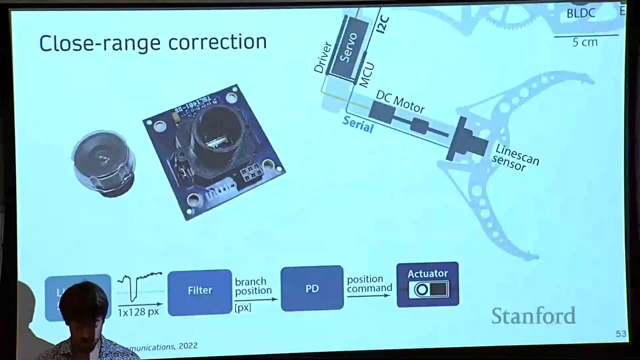 Birds typically have tails that are a lot better, that can twist, turn, extend, But that adds quite a lot of complexity And it's actually an ongoing field of study. So at that point we decided to stick with rather known controllers. 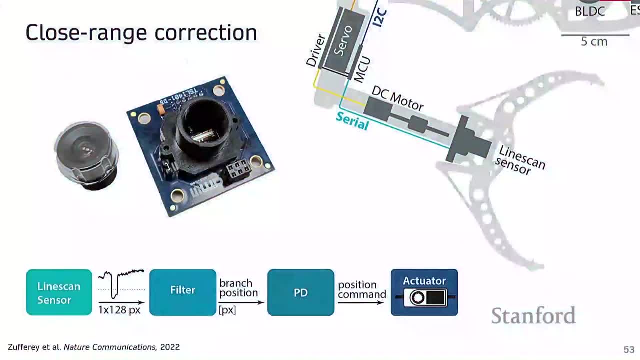 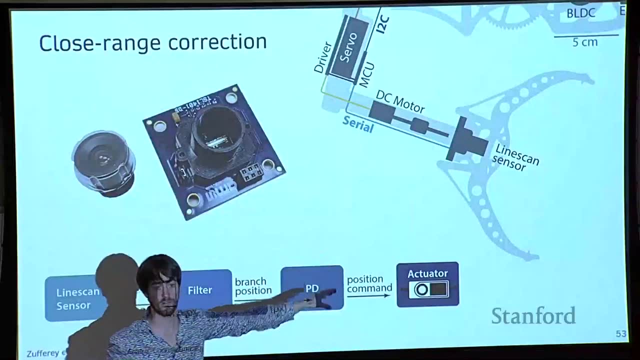 Now I said, as we're getting towards the branch, we need to compensate these oscillations. So for that, this is the solution we came up with. So what we had is we have a line-scan sensor in the front of the claw. 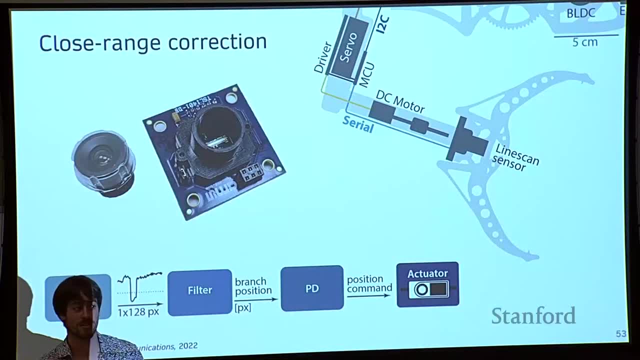 And so what that does is essentially a one-pixel array of camera. So you get these 128 pixels vertically, And what you can do is you can just do contrast detection So you see the branch which is darker in front of a light background. 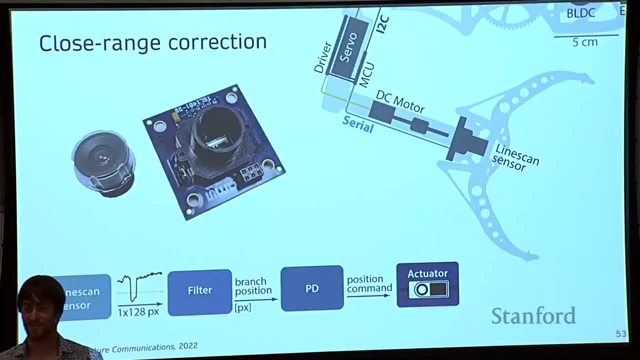 Now, obviously, this is a very crude approach to vision. I would say it's a first step to get some sort of vision. What's really nice about it, though, is you can process this very quickly on a microcontroller, So we're able to get 200 hertz vision feedback. 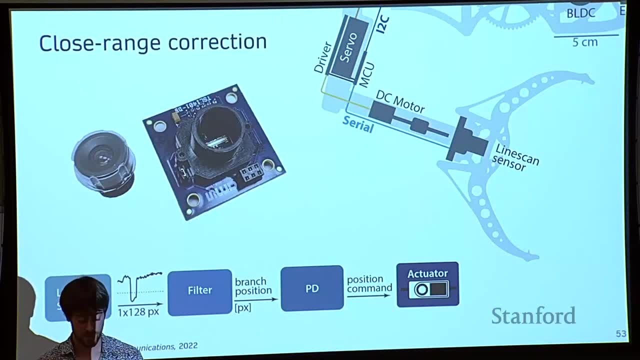 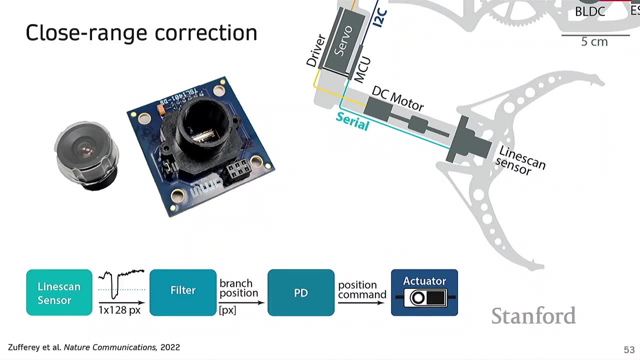 with this sensor running on just a standard microcontroller, which is something that would be very hard to do with a proper camera. The sensor is relatively small. It has a tiny lens, It's sitting next to the claw, And so what it does essentially. 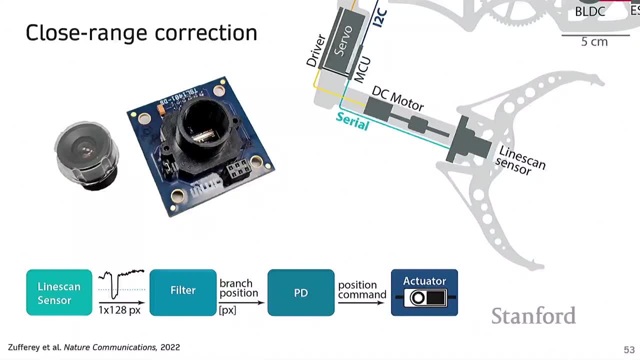 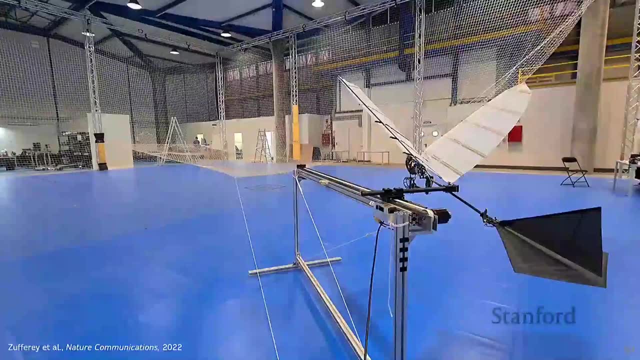 is. it tries to align the claw at all times with the branch when it detects it. Let's go on to some videos, because I think it's the more exciting part. So here we have the robot sitting on this launcher system. That's the thing that I developed when I got there. 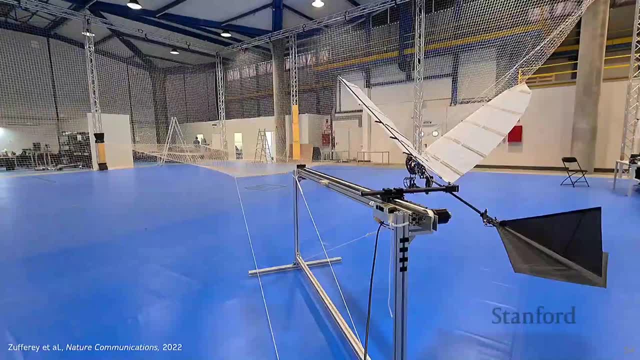 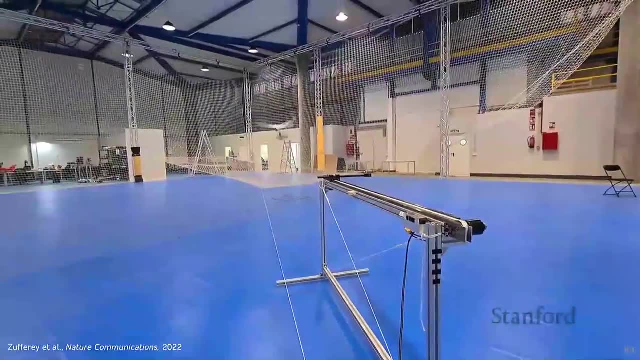 to be able to get repeatable takeoff. And so here we're accelerating to 4 meters per second And you'll see the robot flying across this motion capture zone to the corner to get the maximum distance. And here we're essentially tuning our flight control. 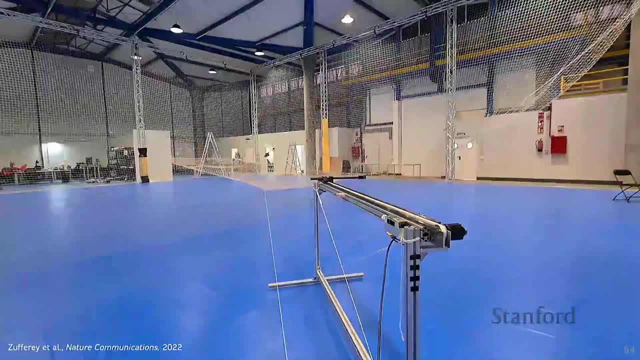 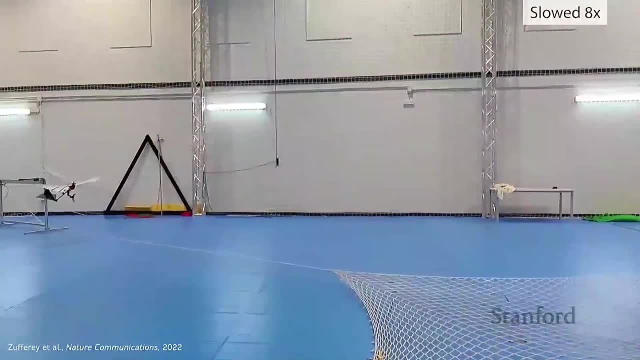 and making sure we can get to the same location. We then took the same robot Once we're happy with the way it flies, And so this is in slow motion now, So our real flapping speeds are about 4 meters per second. 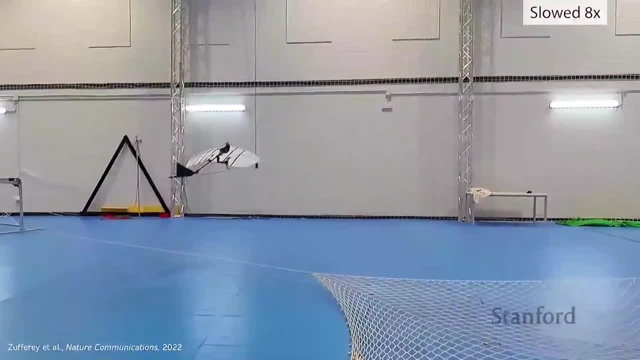 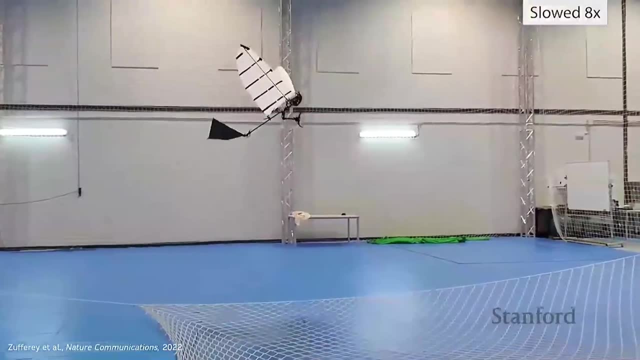 And the step that we did is we actually put a branch, But we didn't put a real branch because we were afraid of breaking the robots, So instead we mounted a piece of foam that's just free hanging in space. You'll see it in a second. 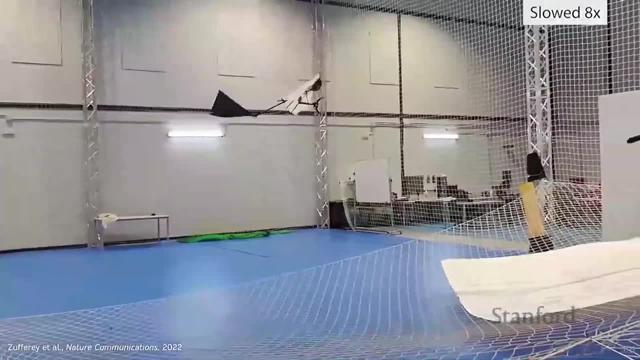 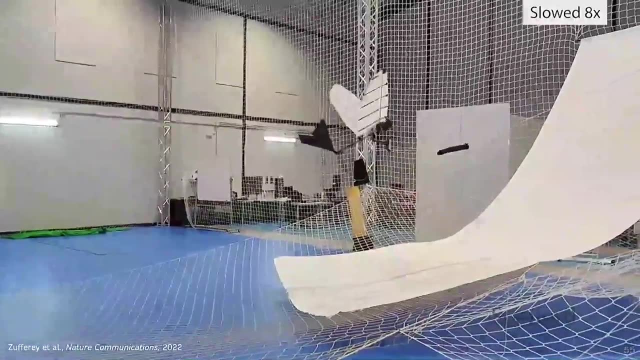 And the robot can already try to adjust and get to the location of the branch. So it was a bit the first test to make sure we don't break too many things. But we still have a black object that we can detect And, you see, the robot gets to the object. 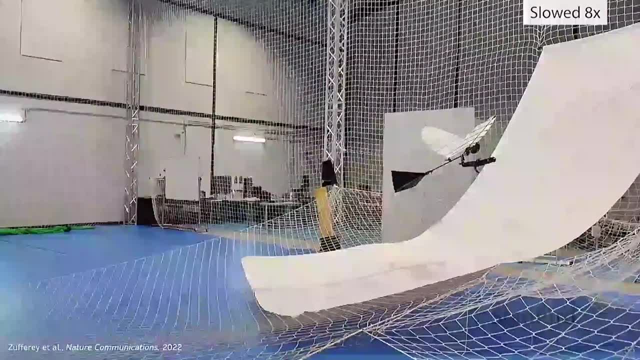 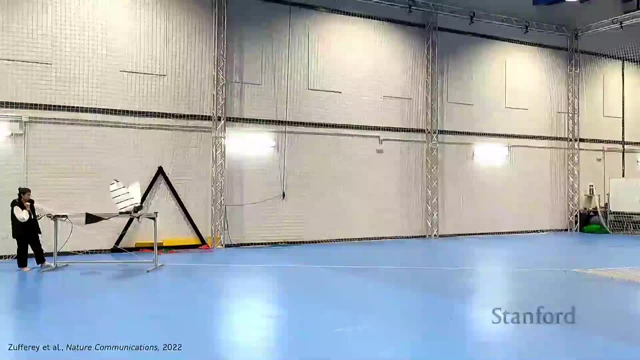 So that moment was like, oh cool, This might actually work, But still it wasn't quite clear whether it would work with a hard branch. So then this here is the first time we were able to perch this robot, And in real time it's flying across the room. 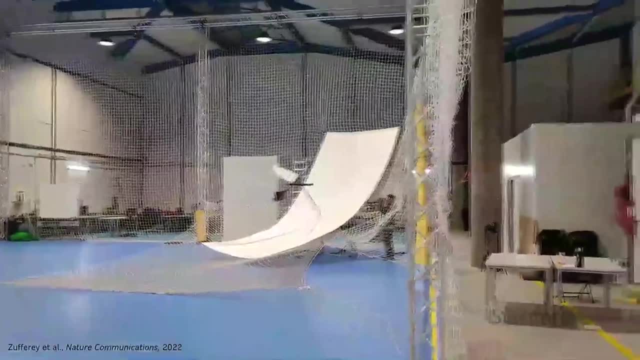 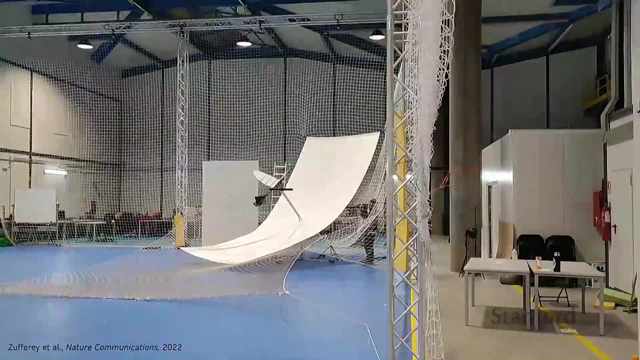 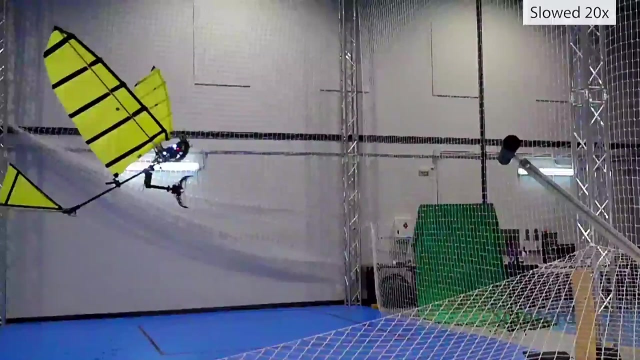 and getting to branch and perching there. So that moment we're extremely happy, Opening bottles of champagne in the lab- big achievement, But yeah, But still, we wanted to see if this is actually a solution that can work multiple times and is relatively robust. 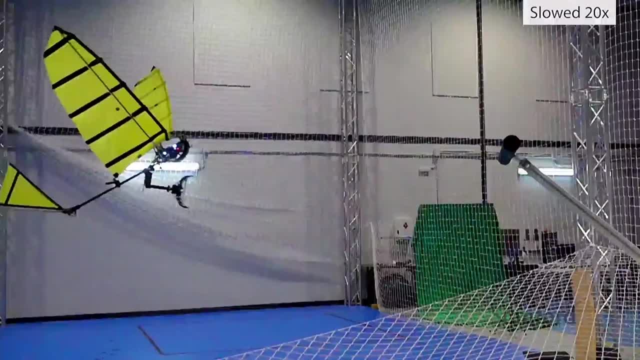 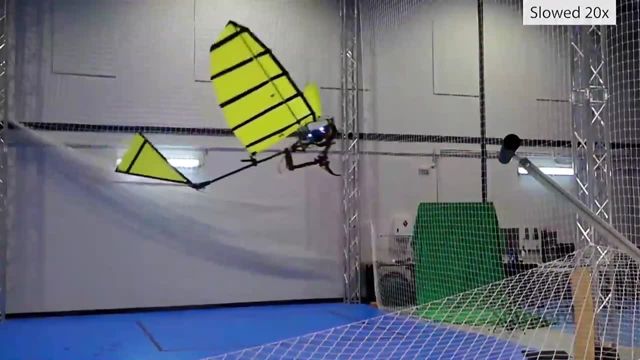 So what we did is we built a second robot. Here it's got yellow wings, But actually the electronics is also a bit different And we're able to repeat that same exact flight without any sort of retuning. So altogether we were quite happy to get this robot. 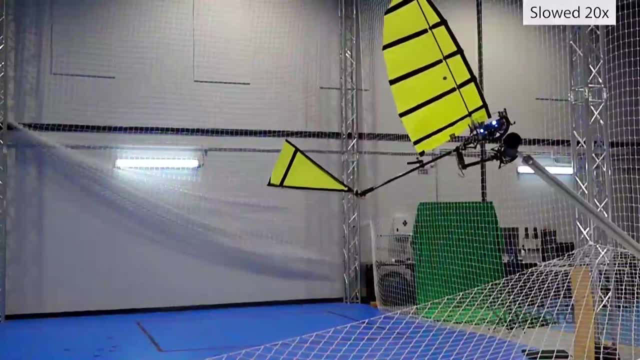 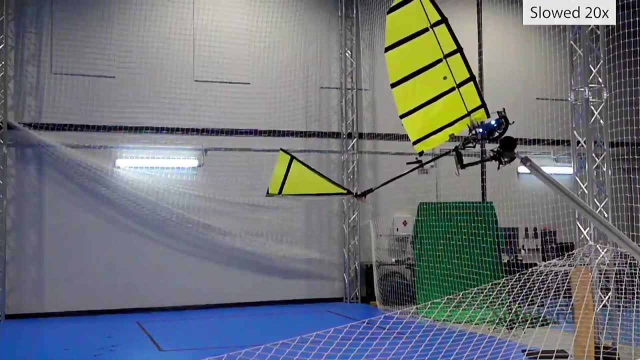 to perch multiple times And even on a second robot. Yeah, I have a lot more stuff I can show, But for the sake of time I'll switch subjects a bit. Now I'll go to essentially what I'm doing right now. 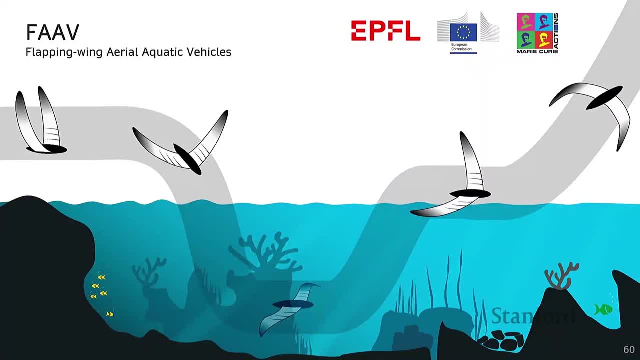 I really like these flapping wing robots. I think they have a lot of potential, But obviously my background, my previous background, was just aero-aquatic locomotion And my next thought was actually: can we do this? Can we get these flapping robots to also swim? 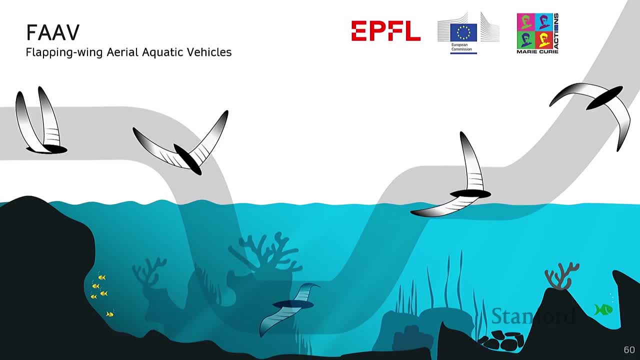 And there it makes a lot of sense to look at the birds. So this is an Atlantic puffer- Atlantic puffins- is this really cute tiny bird about this scale? There's a lot of them in the north of Scotland And they're able to just pivot downwards. 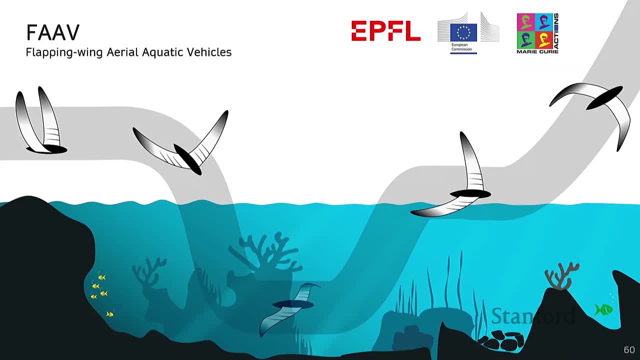 and continue their flight underwater, And so one thing that's really nice about this bird is it doesn't use its feet to swim. A lot of the diving birds continue their underwater locomotion part with the feet, And so this guy here uses its wings. 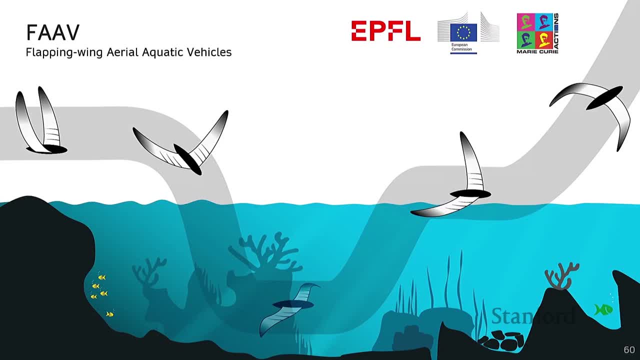 And so that's really nice for us as engineers that try to develop these systems, is we might actually be able to get away with using the same wings for both locomotion, And that really simplifies the mechanics of our robots. So this led to the project that I'm working on right now. 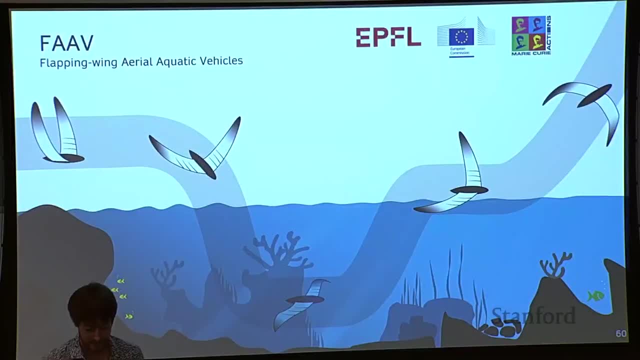 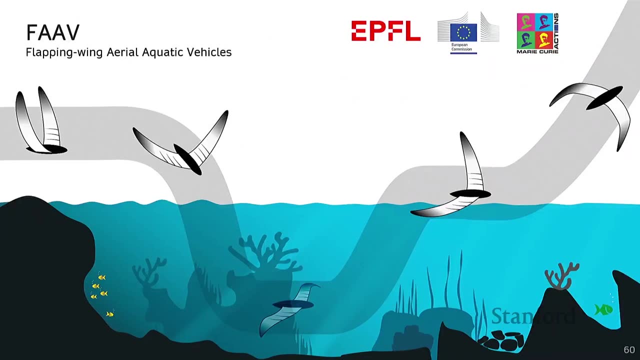 where we're trying to do, these hybrid robots that can fly and continue their swimming underwater. There's a lot of difficult parts that we're trying to break it down into the different steps, But as this is an ongoing project, I'll give you a bit of global highlights of what we're doing. 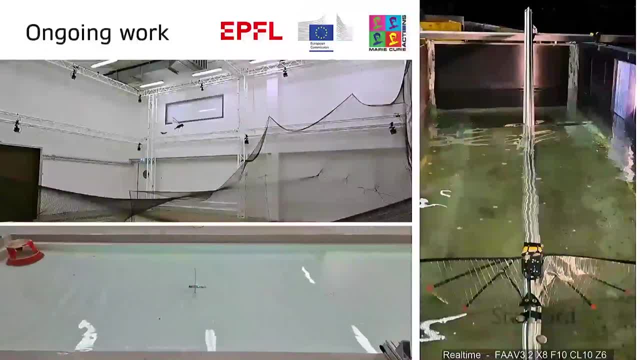 at the moment. So here we have the same robot that is able to fly and swim. So this was already a really big step, because we suddenly have a robot that was designed for air and we're still able to make it work underwater. 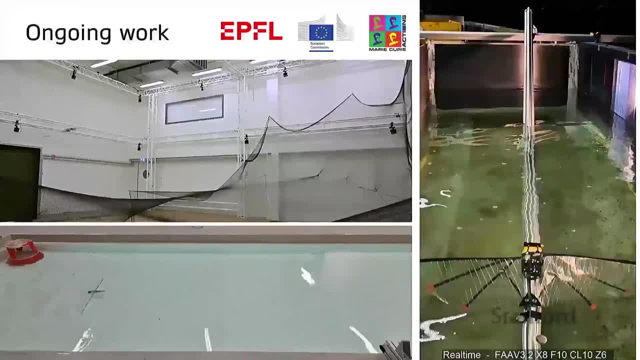 And so there's a lot of structural constraints, communication constraints, electronics constraints, to make something like this work. But yeah, so this is for the flight phase and for the aquatic phase, And one of the things that we've done, that we've been looking at more recently, is the water exit. 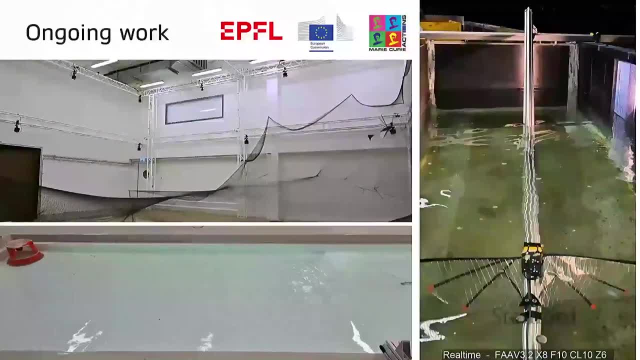 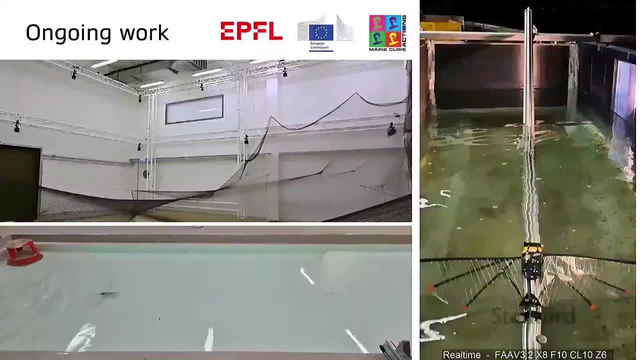 which is the more energy-intensive part and is something that we need to care about. So here you'll see it on the right. This is real time, so it happens relatively quickly. The robot is underwater, affixed to a rail, so we don't have to worry about controls for now. 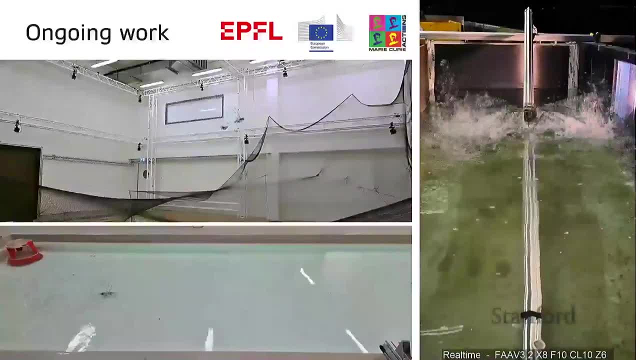 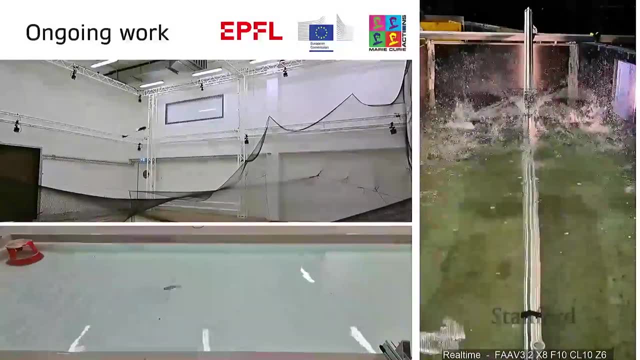 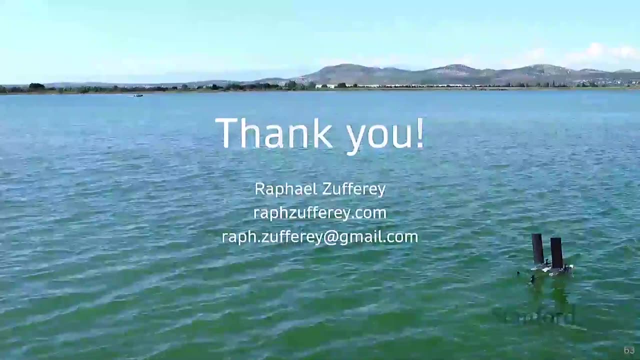 And you'll see what happens as it flies into the air. So this is, let's say, a first step. The robot is still supported, But the next step obviously would be to look at this without rail support. With that, I'd like to thank you very much. 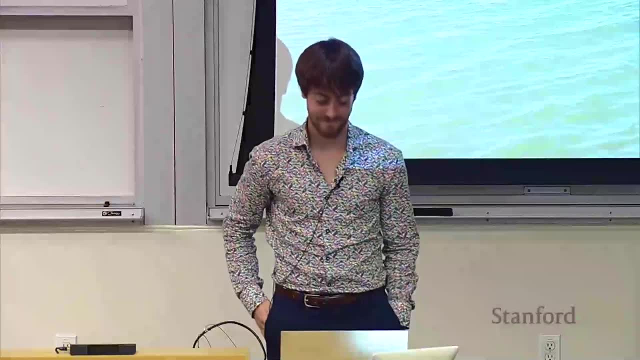 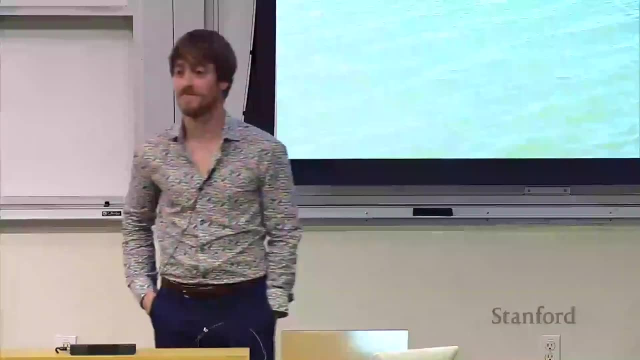 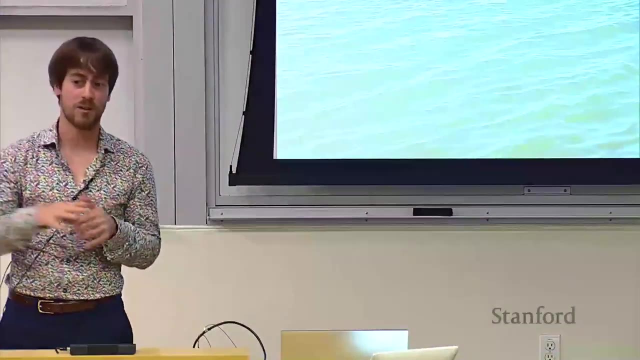 and happy to take any questions. Yeah, Do you do for the flapping robot? do you do trajectory planning or just like a set point that you're trying to get to? Are you talking about the one that's perching on the branch? 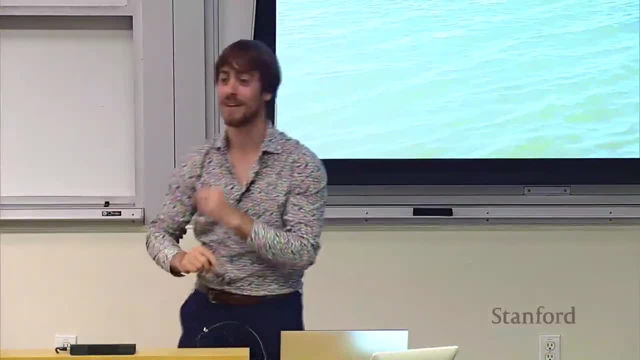 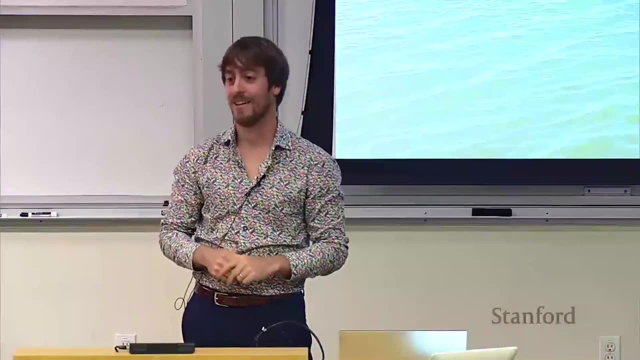 Yeah, no, so that one doesn't do trajectory planning, but we totally should be doing that, I think, because there's some really good work. looking at eagles by Graham Taylor in the UK, right where it'd make a lot of sense. 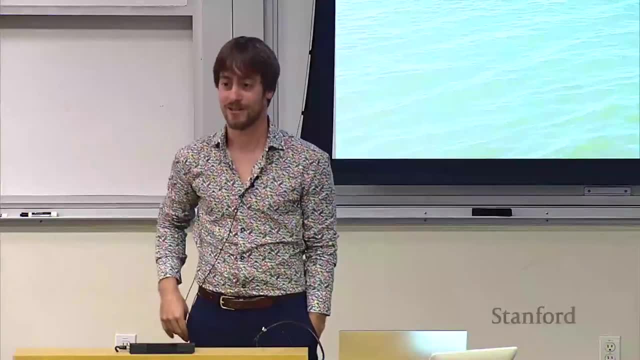 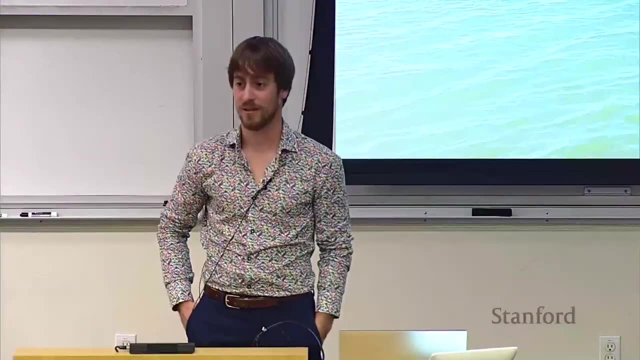 to kind of minimize the stall time that we get to land onto a branch. So this one here is an approach that's basically no trajectory planning, We're just regulating altitude angles of the robot. Awesome work, Thanks. Yeah, With your floating robots. 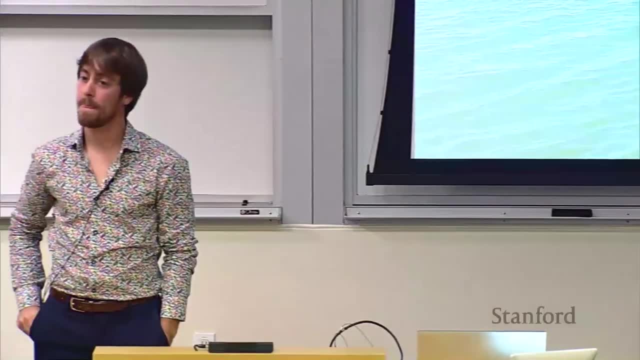 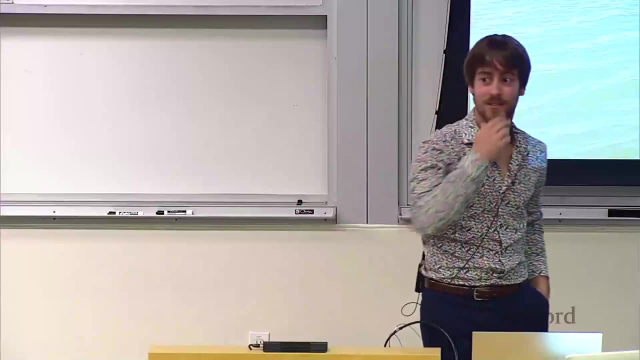 how did you help design them to make them be able to handle waves? Ah, yeah, that's a good question. So you're talking about the one that jumps consecutively right And also the one that had the wings that pulled up on the screen right now. 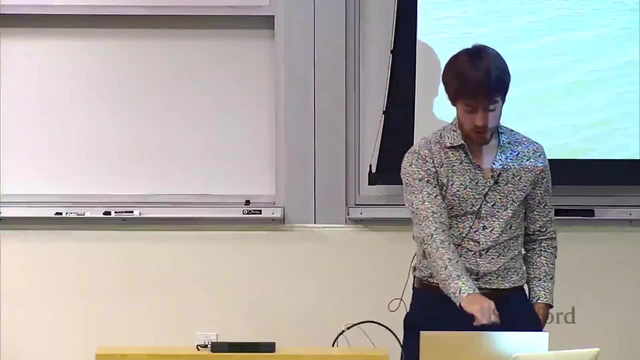 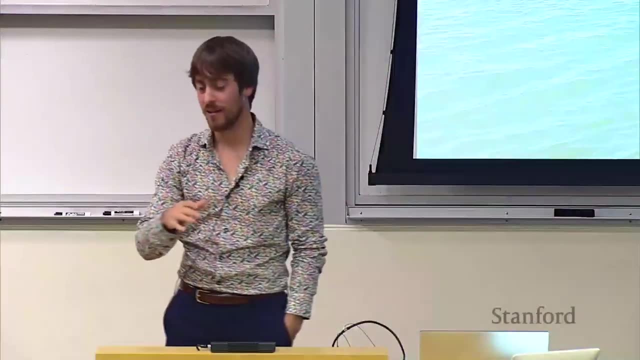 Yeah, so that guy here, So the whole robot, is actually waterproof like top to bottom. so, as in, you know, if a wave kind of comes over it a bit, it's okay, But yeah, it will completely hinder takeoff. 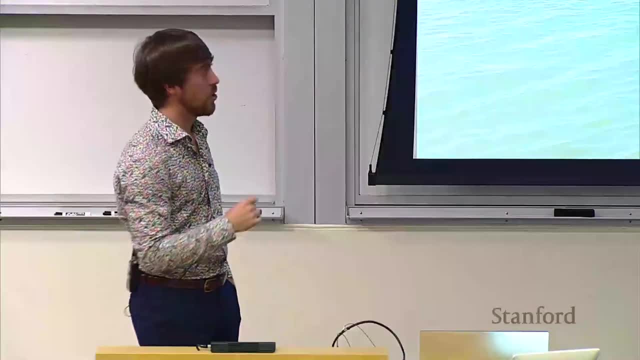 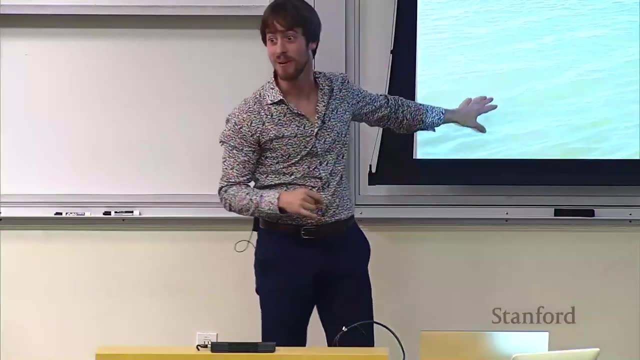 That's clearly a problem. So right now all of the tests have been in calm lakes. I mean, you see here that's already like big waves for this robot. So clearly this is something where you know more work needs to be put in to be able to handle waves. 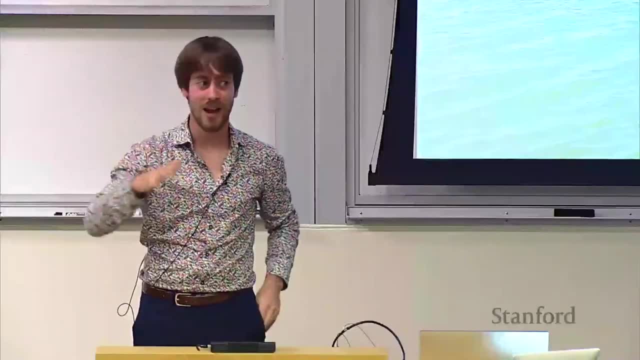 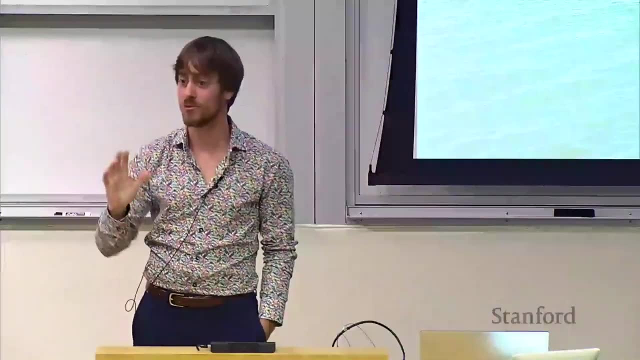 It's a very good question. The other guys that were essentially jump gliding had less of a problem. So actually we put this into a wave tunnel and we're able to see that essentially it just floats with the wave right. 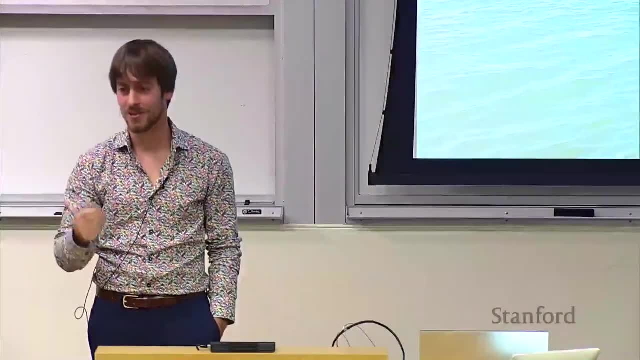 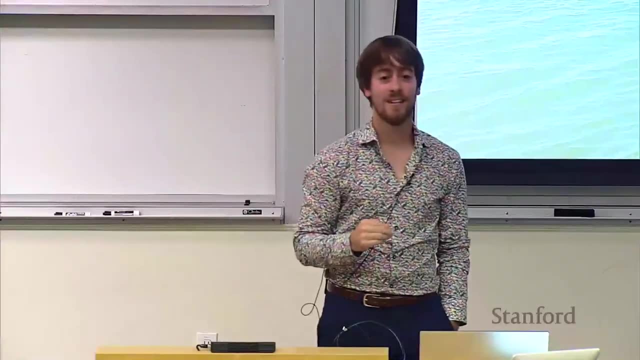 So it doesn't have that much of an impact there. Excellent question. Yeah, Hi, For your sailplane, the one on the screen there you were talking about trying to save waves. Have you made the wings hollow Or are you able to do that? 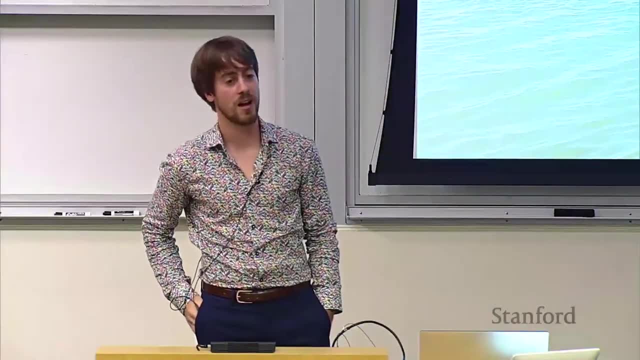 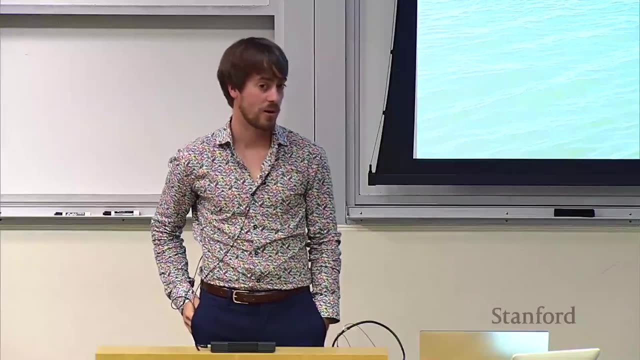 It's a good question. I think if it was hollow you'd have problem with water coming in at some point, probably. So here it's a foam core which is fairly light, So we've optimized which foams we're using. 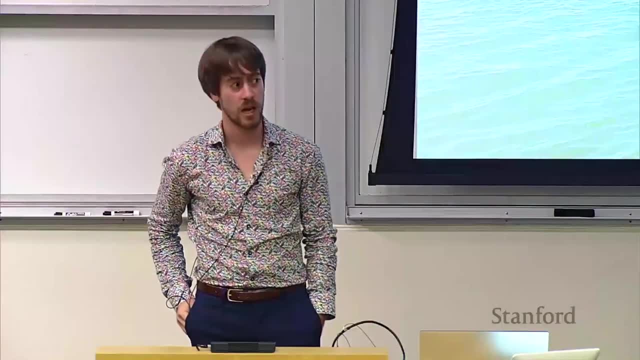 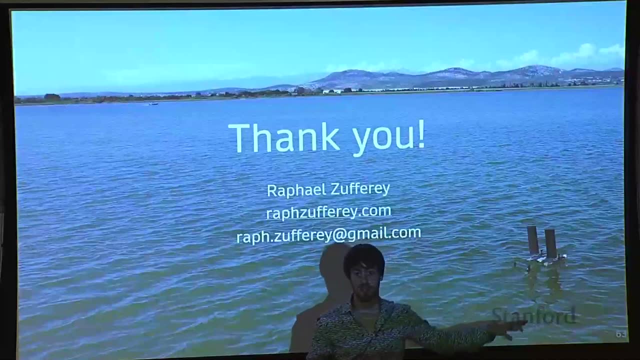 So we're able to get wings that were fairly light. I would say, rather, one component that more work needs to be put in is rather the floating part, Because that's something that is hollow. Therefore, you need a shell that's relatively strong. 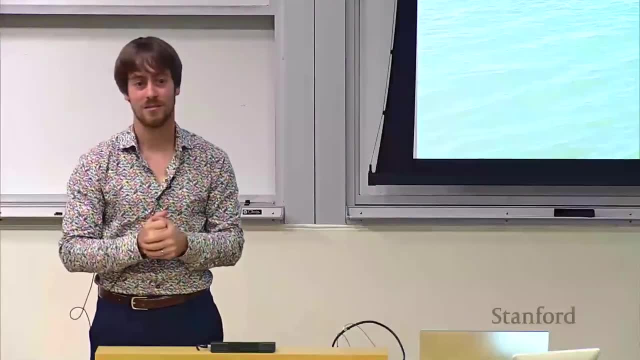 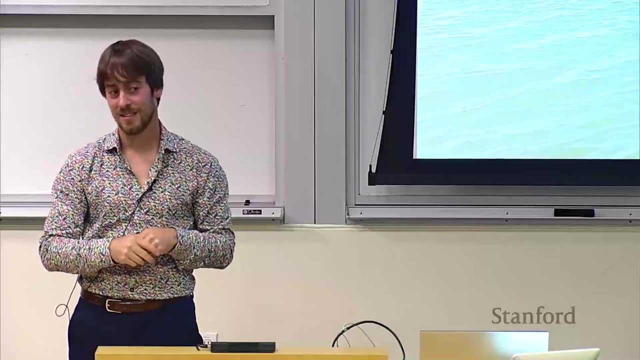 So there there could be more work. definitely to make it lighter, Yeah, But yeah, good question. Yeah, I know, for the flapping robot, all the examples you showed of flight kind of involved, it being, I guess, assisted by that launcher. 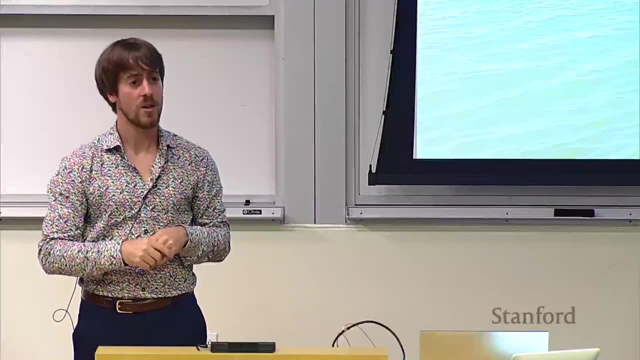 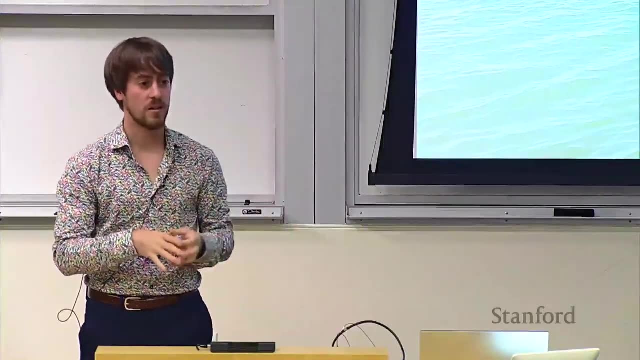 Is it possible for it to fly just kind of on its own off the ground? Yeah, There is publications that demonstrate takeoff from the ground. A lot of them are mostly kind of the smaller scale, Also robots that are capable of hovering. 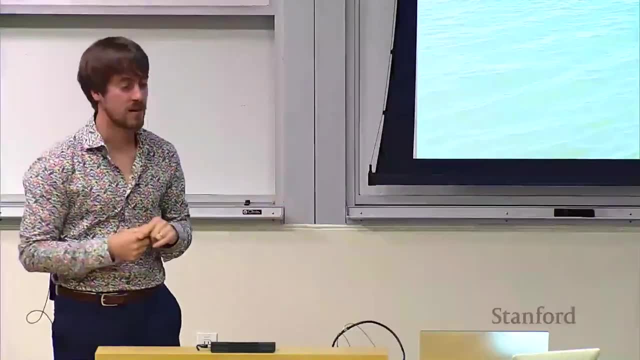 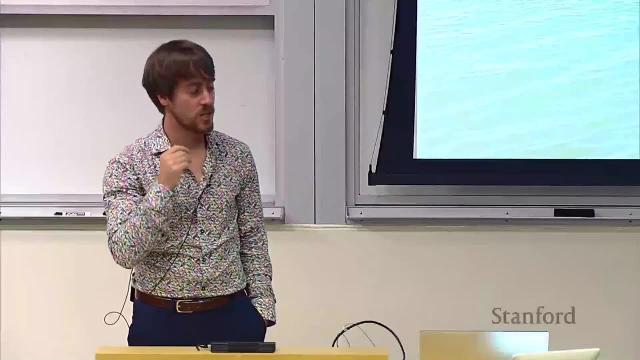 So if you can hover, you can usually take off. Yeah, But a lot of the times we're also just hand throwing them, And actually that works quite well, because a flapping robot generates quite a bit of thrust at low flight speeds. 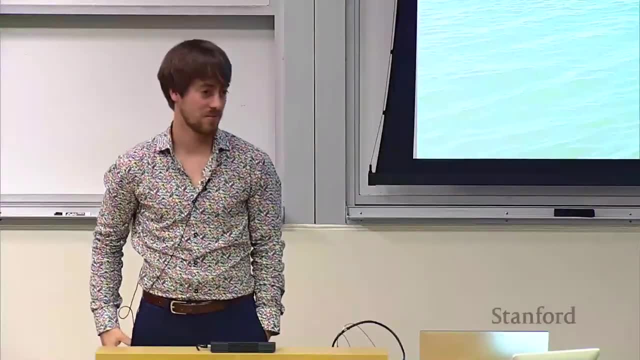 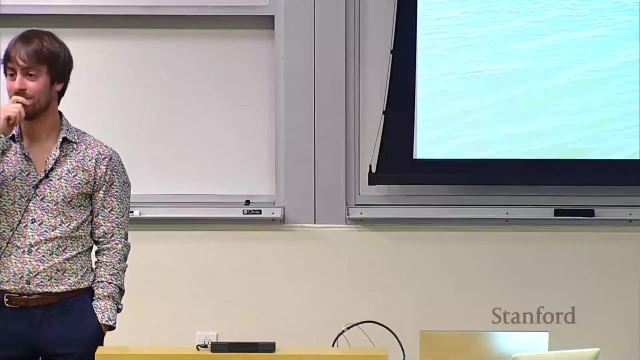 So you can just take in your hand and just throw it like this. But yeah, it's a good question. Thanks, Yeah, How would you compare the types of maneuvers you can do with a fixed-wing robot and a flapping-wing robot in terms of flight capabilities? 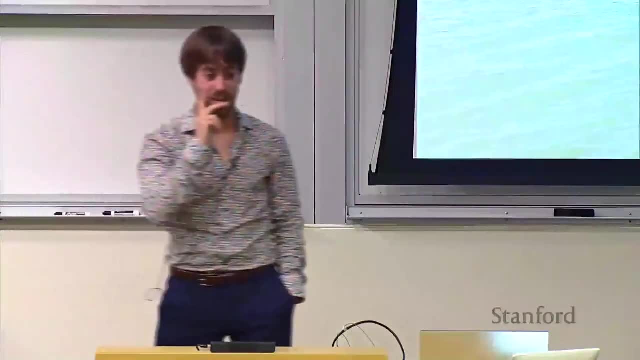 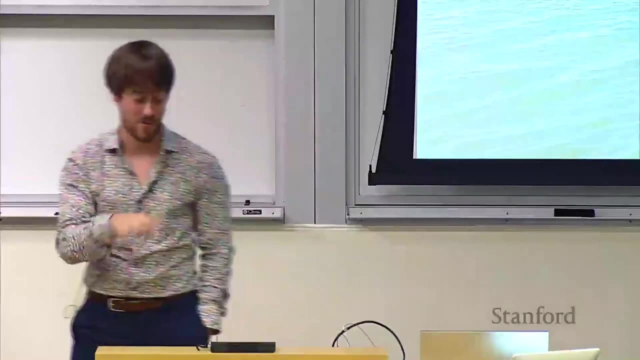 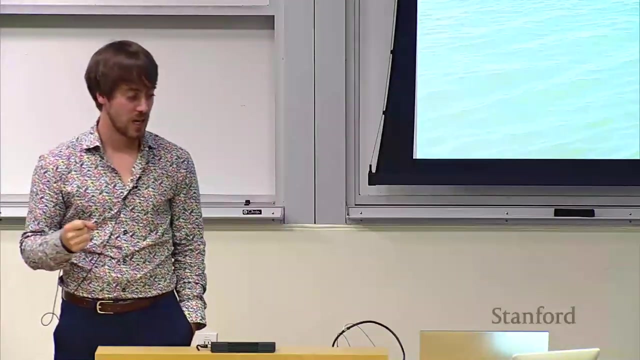 Yeah, Excellent question. With the flapping robots you can really flap one wing and stop the other wing if your mechanics permit it, And then that gives you really sharp turn rates. So that's something that you can do because it's very interesting. I think in terms of fixed-wing robots, that would be more difficult. Now there is also a lot of work going on in my current lab where they actually try to change the geometry of the wings. So there is, let's say, ways around it. 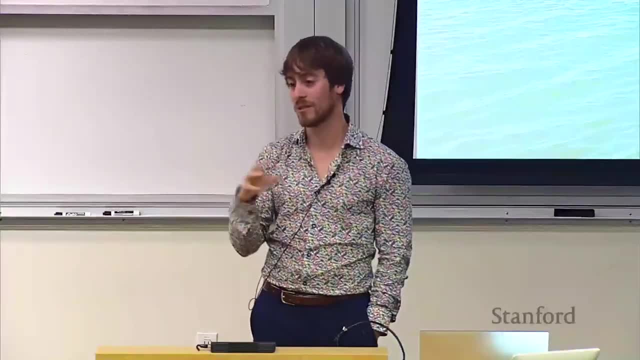 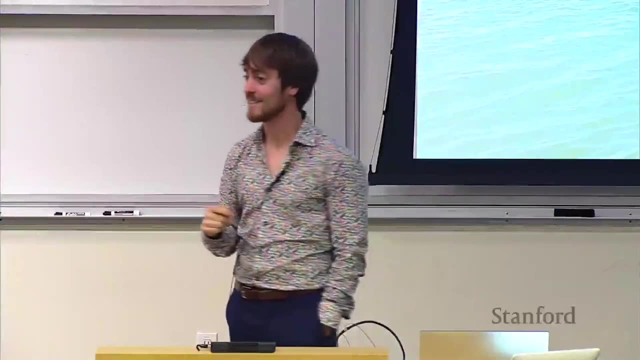 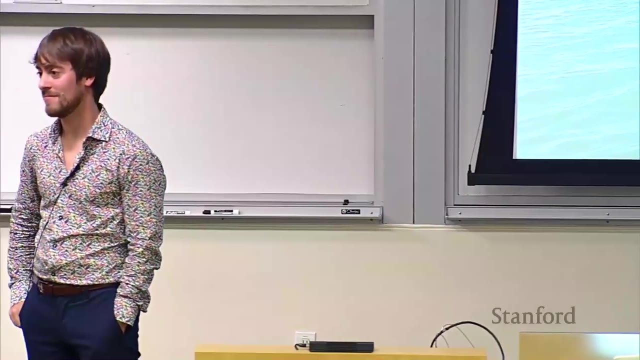 that you could still be in a fixed-wing configuration, but you're morphing the wings to actually get higher maneuverability, So it's an ongoing field of research. Thanks, Yes, Is there any desire or any work looking into being able to dismount from a perch? 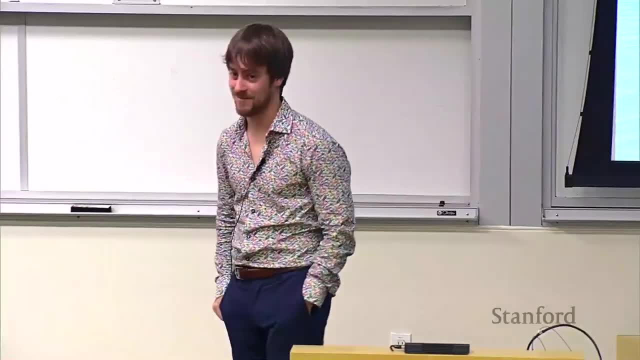 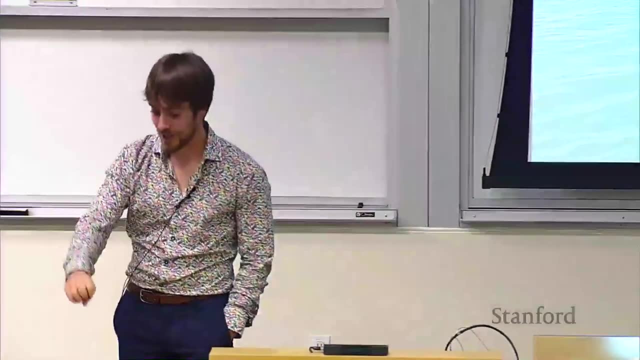 to go to maybe another perch. Have the mechanism be able to handle that? Yeah, excellent question. It's clearly like you see this. you're like, OK, well, no, how does it get off right? And we did design the claw so that it could open. 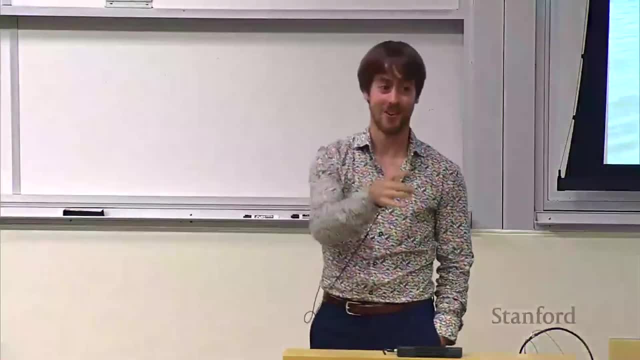 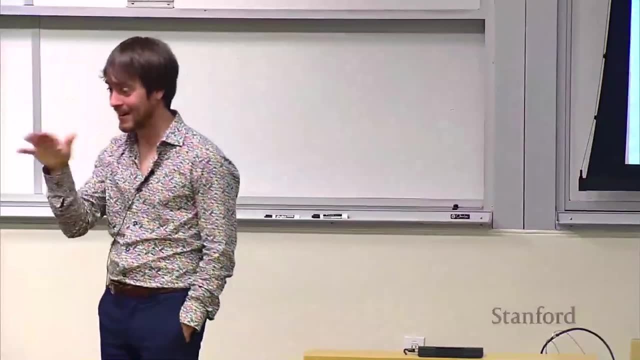 And fly off, But obviously it doesn't work right Because you need the launcher to actually get to a certain flight speed. So at that moment I left the lab, So I didn't get to continue to work on this, but this was clearly the next step. 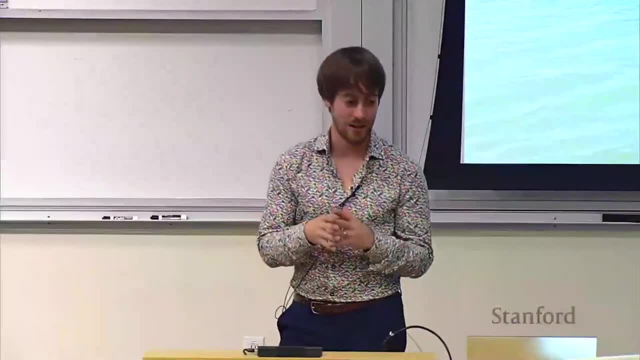 that I was the most excited about. I guess there are several ways you could do it. Either you could let yourself fall, So if you're far enough from the ground, you fall, and then you get your flight speed from that and you continue flying. 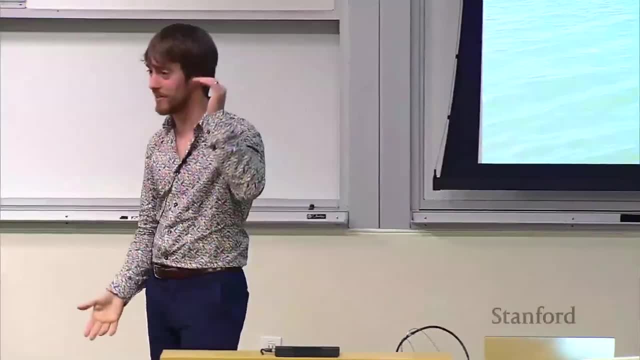 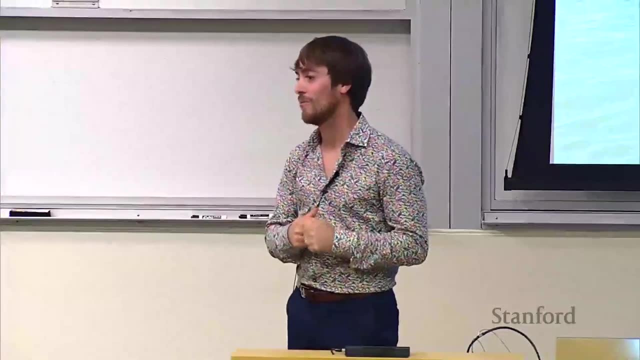 So that's a first option. It's probably the simplest if you have the distance, but often you don't right, Yeah. The other approach would be to actually have some sort of jumping built into your legs, which I think would be the most interesting to look at. 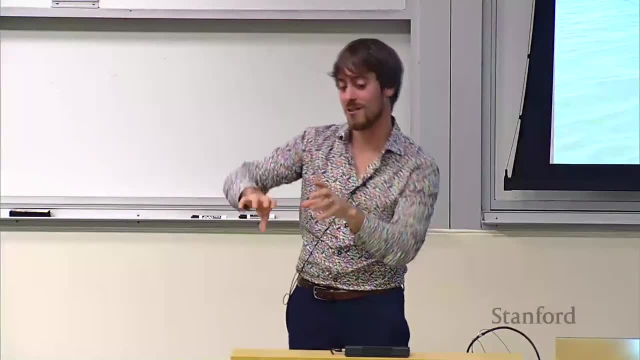 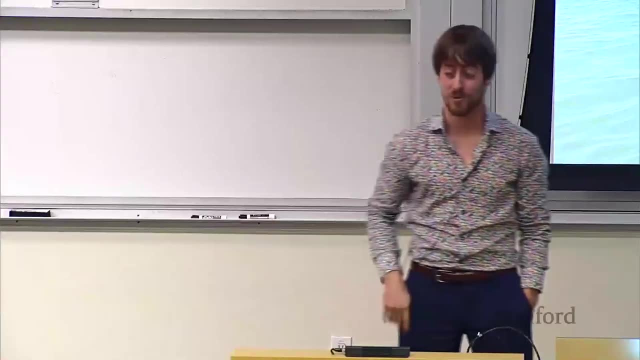 But it's quite challenging, right, Because you land onto your branch and then so you need to adjust your position so that you'll be able to do the jump right. So I think there's still a lot to be done, especially with these flapping robots. 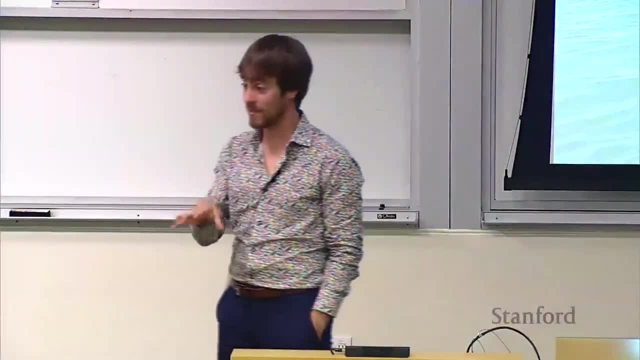 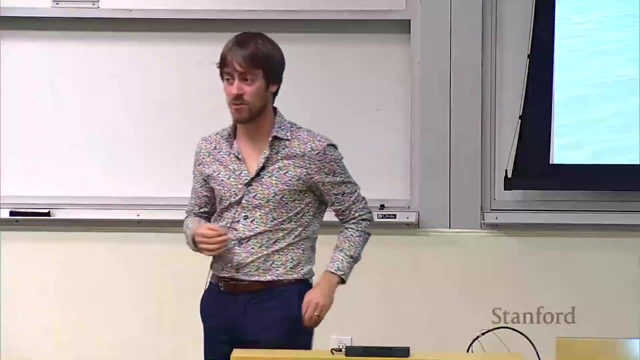 Or you increase- that's the last thing- or you increase the power momentarily that you can give on your flapping wings and start to look at hovering with these robots. But in large scales it's quite difficult, Yeah, But excellent question. 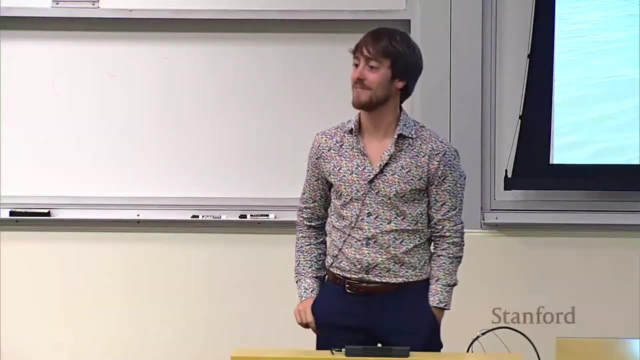 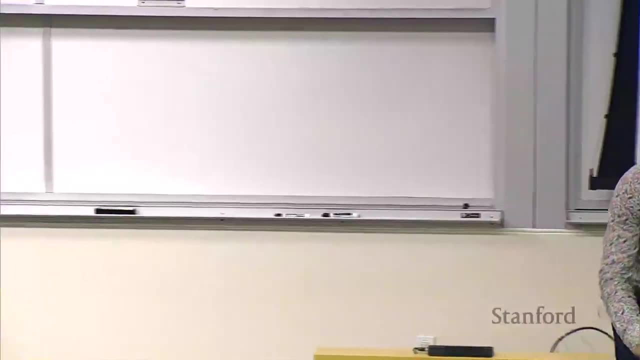 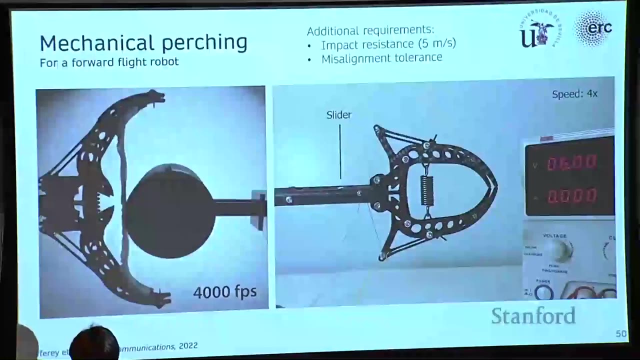 Yeah, Yeah, For the claw once you hold onto the tree. I was wondering: how do you prevent rotation of the actual robot? Do you just rely on pure grip strength or is there something? Essentially, yeah, Let me go a bit further. 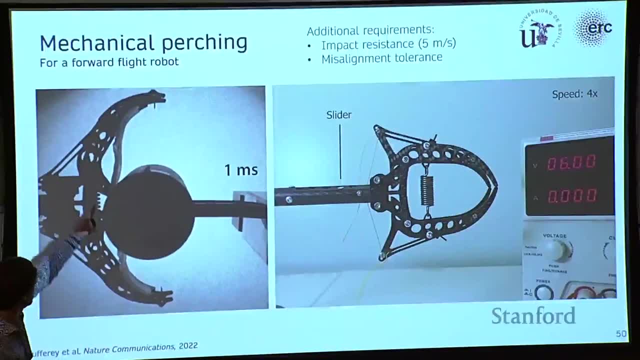 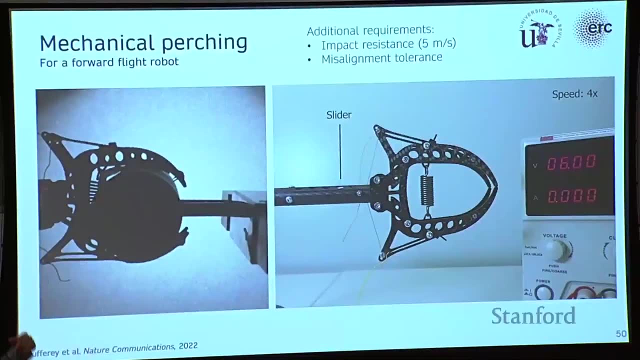 So yeah. So what we have here is we have a silicone membrane. You see it here. It deforms right, And then you have two spikes in the front, And so what that does is it's not really so much the spikes that are holding. 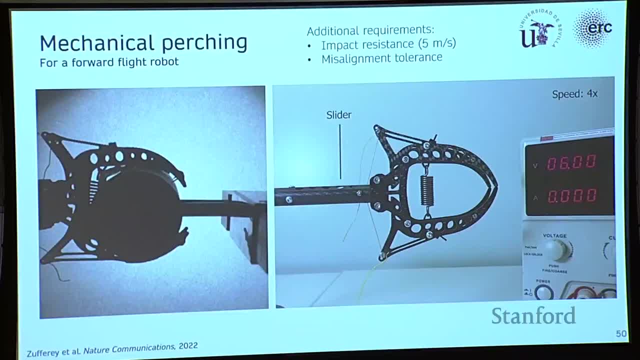 because the wood is really hard that we're using It's actually more that it's pressing the wood into the silicone that you have here that coats the inside of the claw. So really the silicone in here is doing a lot of the holding there. 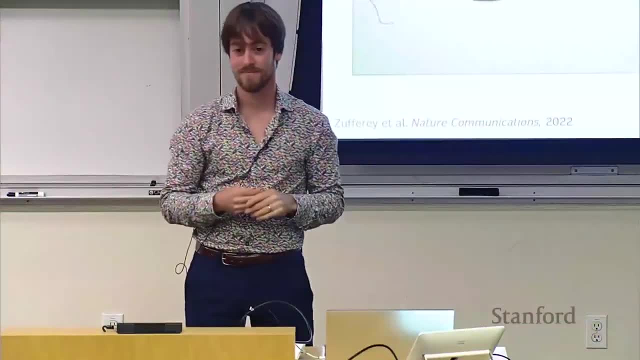 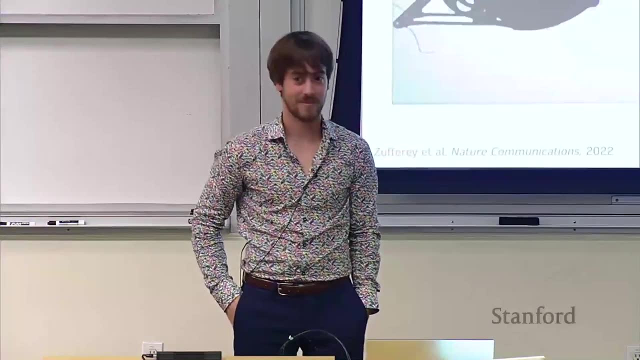 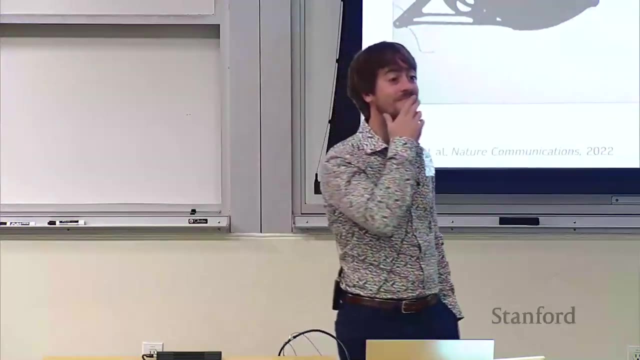 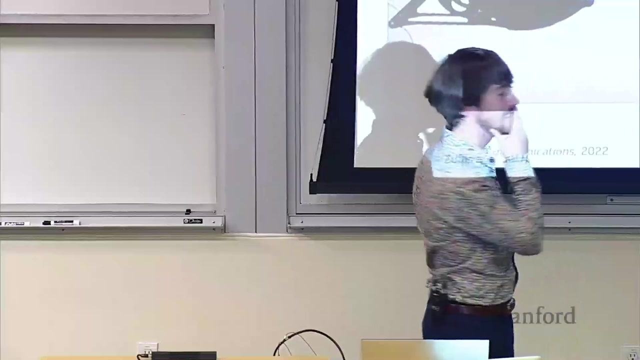 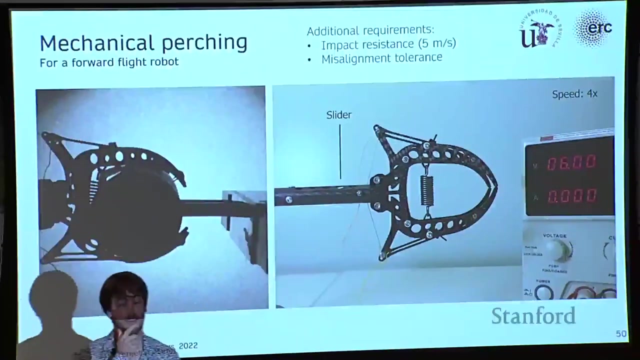 Yeah, All right, Any more questions? Yeah, You mentioned about that. there are risks of fast-moving propeller. you cannot pull them. Yeah, But what other is associated with this claw when someone catches it? So would it be dangerous if you are gets into it? 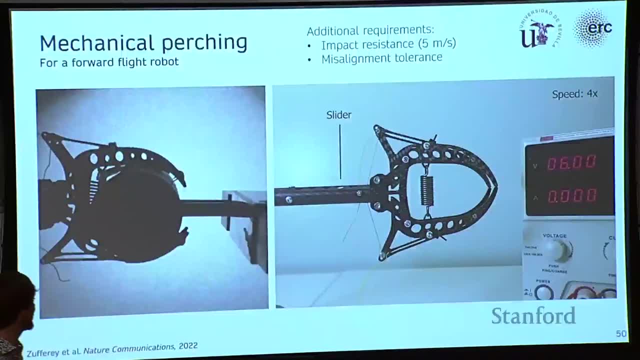 Yeah, Yeah, Easy answer. yes, I mean, here you have something that I mean. the problem is probably like these spikes, I guess the actual closing we had it on our arms. It's okay, But yeah, you still have these spikes. that wouldn't be so good. 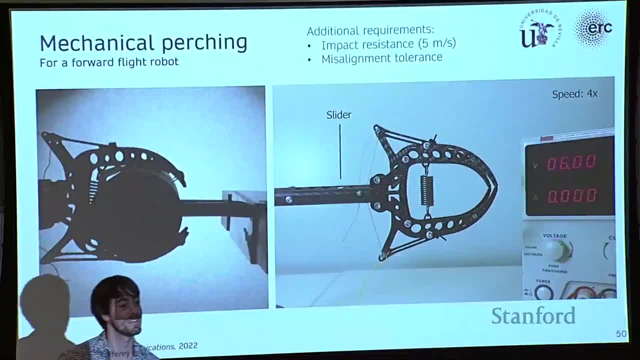 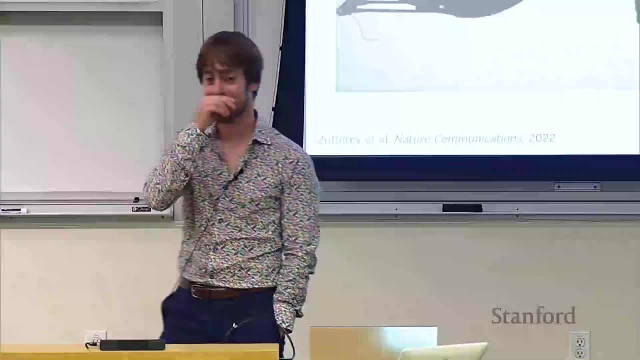 if it was to actually close onto you, right, That would be something to avoid. yeah, Definitely. a lot of more soft robotics approaches would be good there. Yeah, How would it take off again? Yeah, That's a good question. It relates a bit to my previous answer. 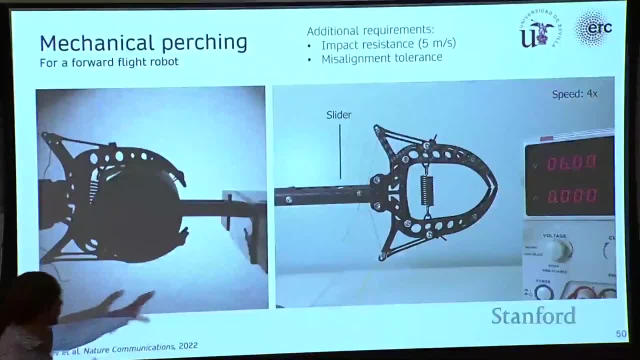 Yeah, So essentially here it's able to reopen. So that part mechanically is possible. But then the problem is getting to the flight speeds right, So getting to have this initial energy to be able to take off, Or you go into a hovering flight. 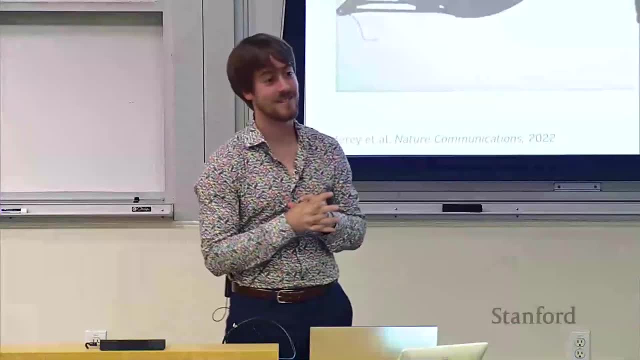 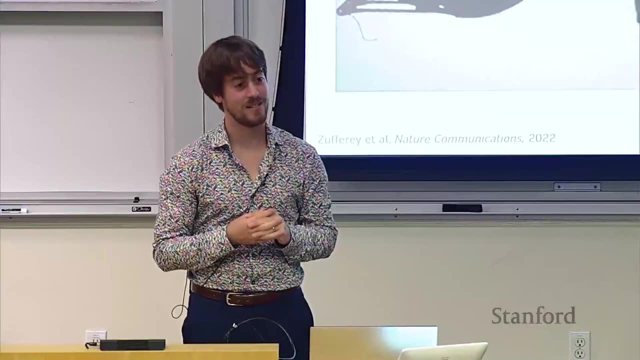 That's the other option. Yeah, Opening the claw takes a lot of time. Yes, And that time most likely the bird will just fall off the branch. Yes, Could you like conserve some energy in some spring Or something to help it rapidly? 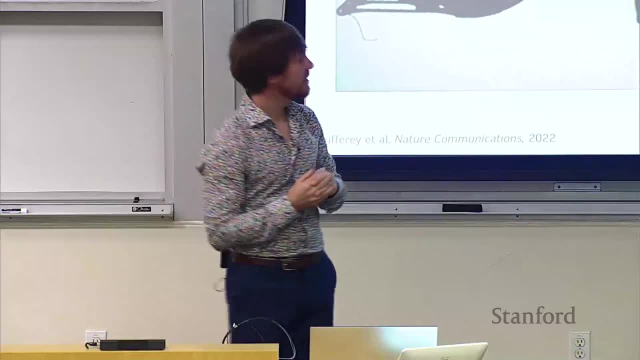 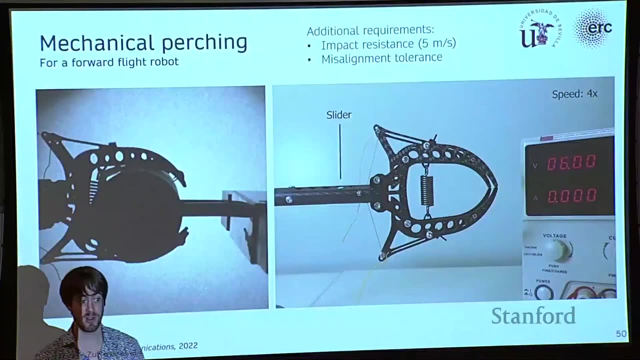 It's quite difficult because the problem we have is you need the high forces right. So by having a system that's bi-stable and you preload with energy right, Allows you to give like to get very fast speeds and very high forces.